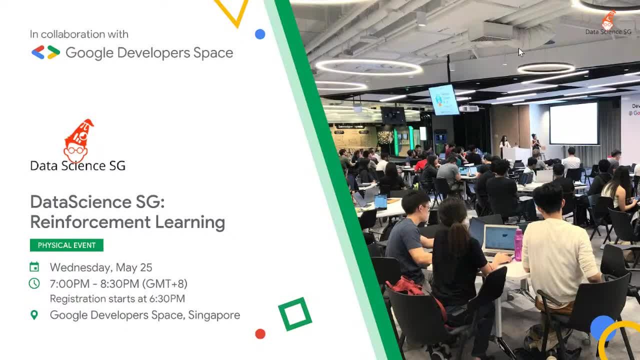 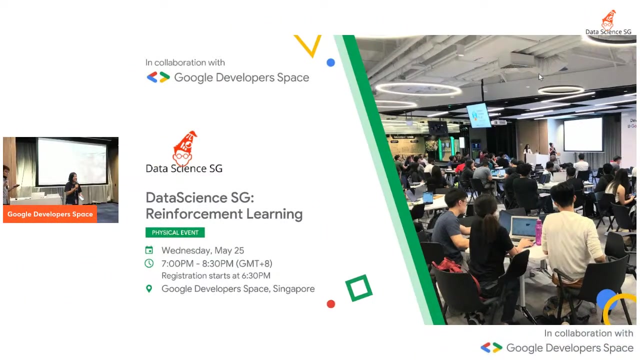 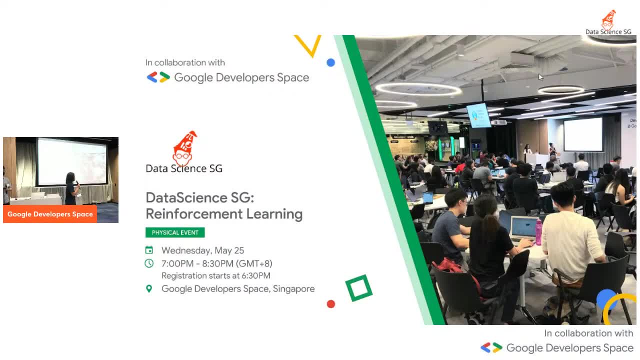 Yeah, and just a show of hands. how many of you? this is your first physical event for this year. Oh nice, That's a lot of you. Yeah, a warm welcome to Google Developer Space And just a quick introduction on who the team. 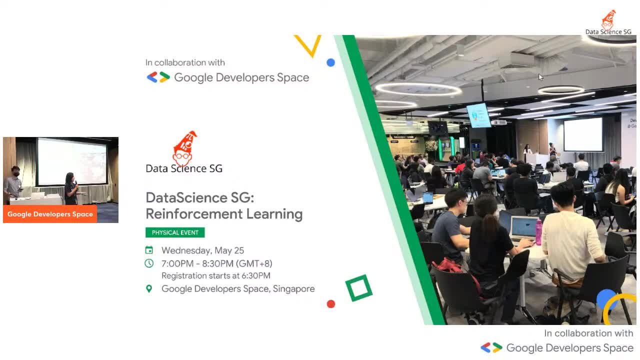 who is in the team? I'm Jiaxing from the Google Developer Relations team, So I take care of the developer and startup communities in our region. And Lawrence, over here. he's our events manager And I'm the team manager at Google Developer Space. 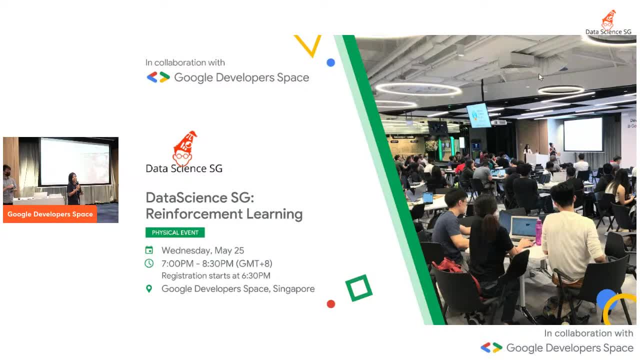 I think many of you will have seen him online for the past two years if you have joined Data Science Singapore's online events. So, yeah, really happy to see everyone here in person. Thank you for traveling all the way down after work. 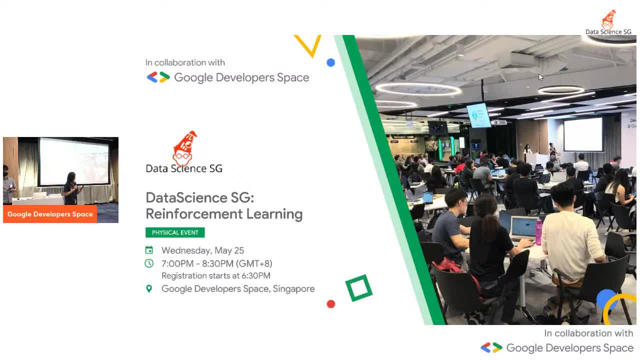 be it from your office or working from home, And a couple of housekeeping. We do need everyone to keep your mask on at all times. So I do see everyone has their mask on. Thanks for doing that, And yeah, except for me. I'll put my mask on straight after this. 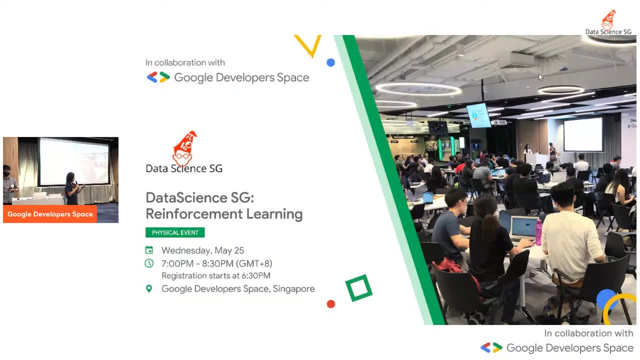 Yeah, and shout out to Data Science Singapore's team for hosting your session with us here today. I'm sure there are no stranger to you- People like Ivan Kaixing, Koo Sonima Raizal. I think you'll see them around later on. 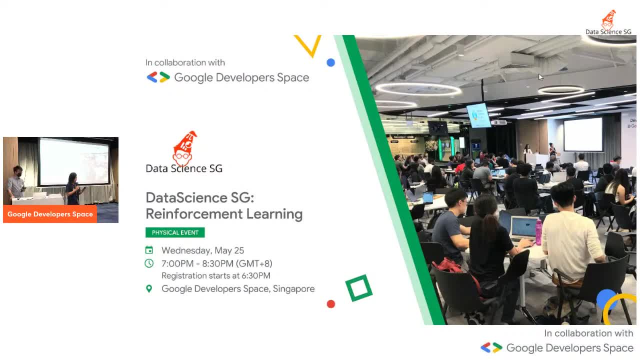 Really happy to be hosting everyone here. And, yeah, before we begin our presentation for today, let me just briefly introduce what Google Developer Space does. So we are home for developers And startups from around the region to learn and connect with one another. 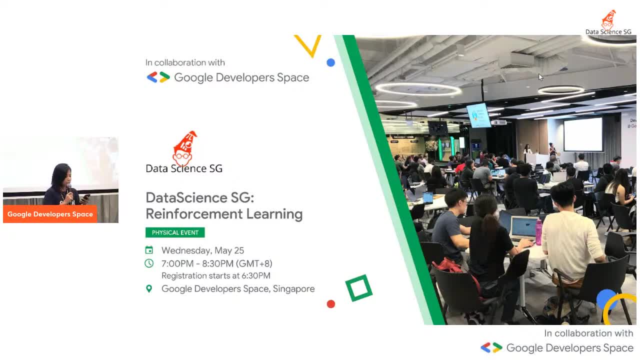 And we want to empower and connect the communities through our people, programs, network and technologies. So, yeah, take lots of pictures. while you are here today, I saw many of you taking out your mobile phones, taking pictures. Yeah, and do tag us as well. 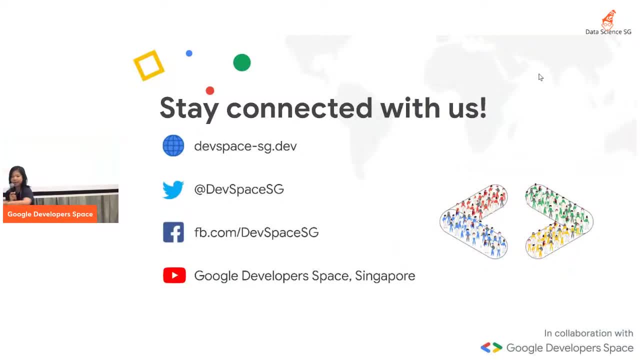 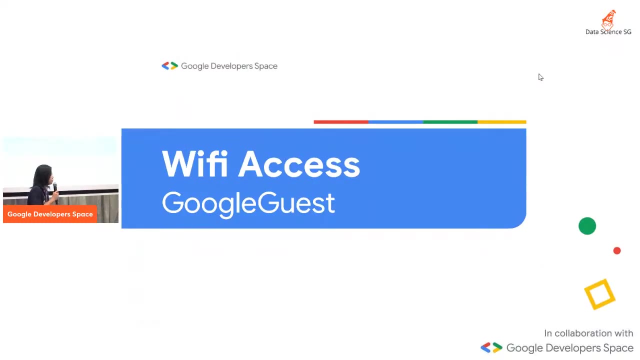 We are on all these social channels, Yeah, so on our website we update the events that we have, And we are also on Twitter, Facebook and YouTube. And yeah, the next one: Wi-Fi access. If you need Wi-Fi, it's Google Guest. 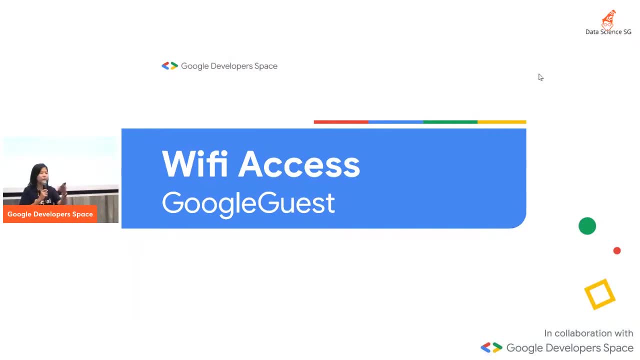 And if you need to use the washrooms, they are at the back of this space, So feel free to use them. And yeah, now I would like to pass the time over to Ivan, who will: Oh, no, okay, last slide. 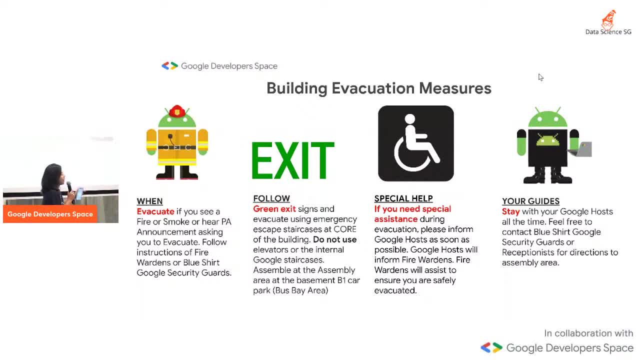 A very important slide. So this is the building evacuation map. Building evacuation measures. It's very wordy, But TLDR, if anything happens, look for me, Look for Lawrence, Follow us. We will go down to level one. 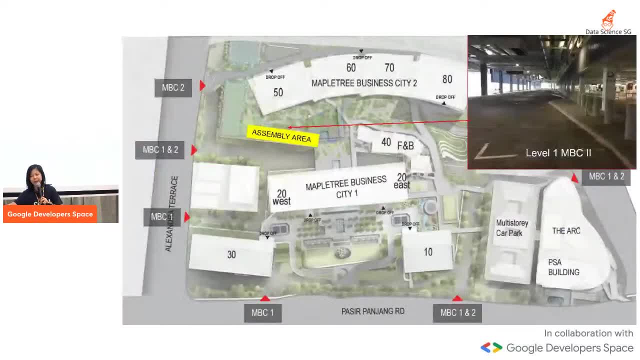 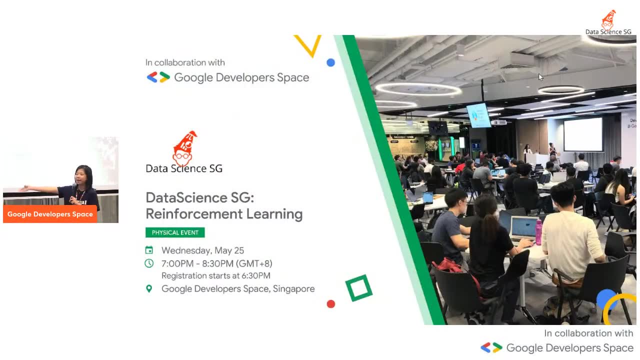 This is in case of an unlikely emergency. Yeah, so don't worry, You are safe with us. Just look for us and follow us on our way down. And yeah, last but not least, Ivan, the organizing team for today, will be sharing more about today's agenda. 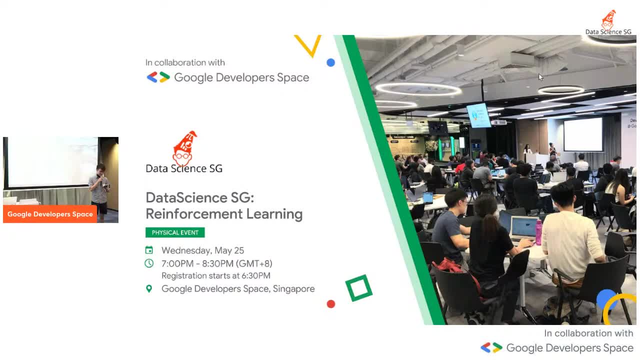 Hello everyone. Thanks Yaxing for the introduction. So thanks everyone for coming down, despite the dicey weather we have today. I hope nobody is drenched. So we are running a bit behind time. I'm going to quickly go through the agenda. 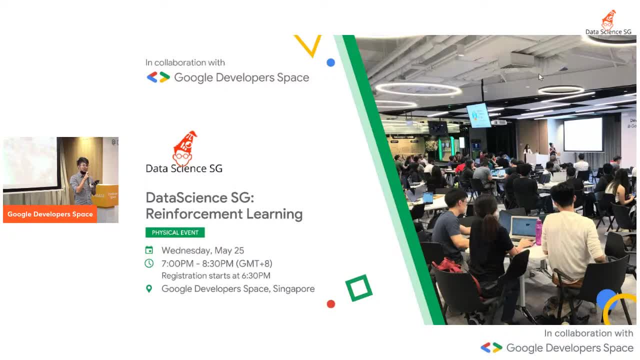 So from 7 until 7.40, we will start off with the basics of reinforcement learning. 7.40 to 8.20, we will have practical reinforcement learning And then for the last 20 minutes- Oh sorry, 10 minutes- we are going to have the Q&A. 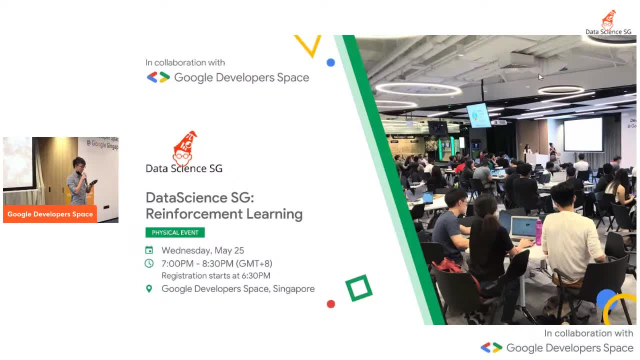 So I will quickly introduce our first two speakers. The first speaker we have Tuya, who is a machine learning engineer. Tuya, can you? Yeah, just wave your hand. So he is an experienced machine learning engineer who likes to create applications. 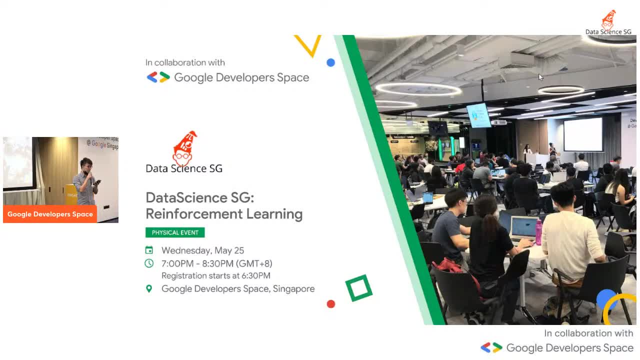 build data pipelines, scale machine learning models and move them to production. So he is also passionate about AI technologies, mainly in reinforcement learning, computer vision and generative adversarial networks. So during his free time he contributes to the tech community by organizing hackathons. 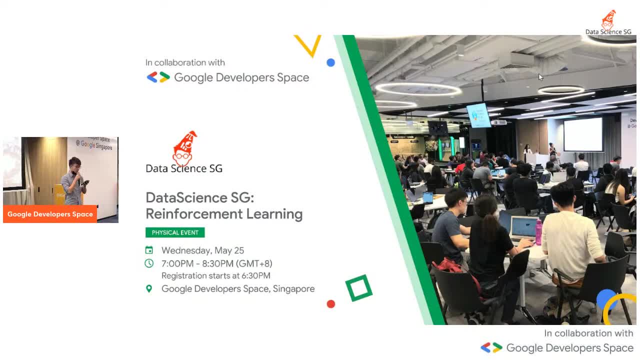 conducting workshops and mentoring the next generation of developers. So for the next speaker we have Kai-Singh, who is the VP of machine learning and innovation at DBS. Kai-Singh, can you wave your hand? Yeah? 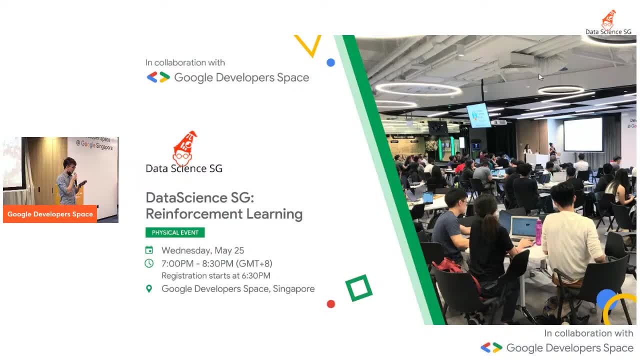 So he works at the intersection of data and product innovation. So over the last 10 years he has led data teams in developing machine learning Products such as deep learnings, animal models, knowledge graphs, recommender systems, segmentation. 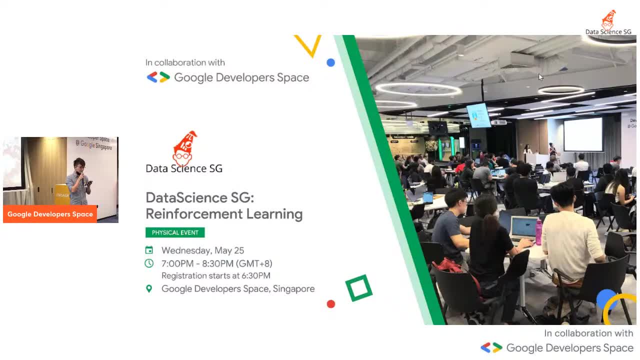 and targeting across industries like finance, media, jobs, e-commerce and healthcare. He also specializes in interactive intelligence, designing systems where AI and human intelligence can coexist harmoniously and thrive. So, without further ado, I am going to hand over to our first speaker. 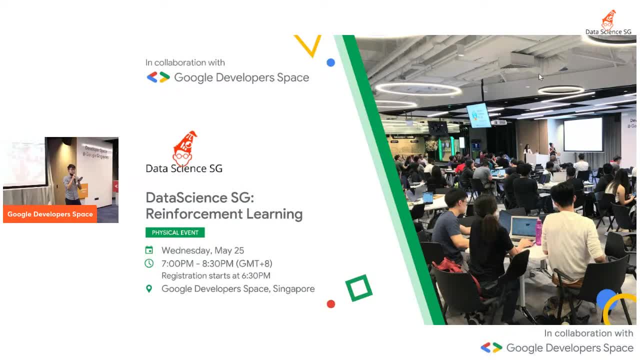 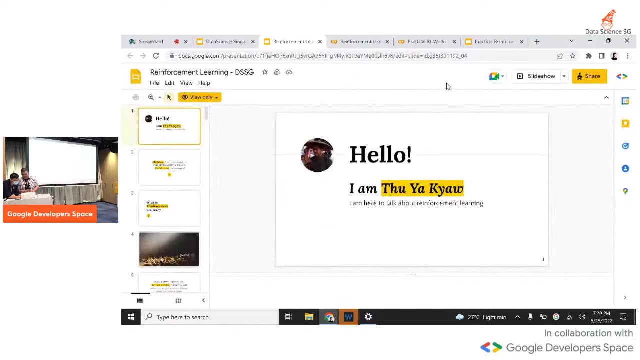 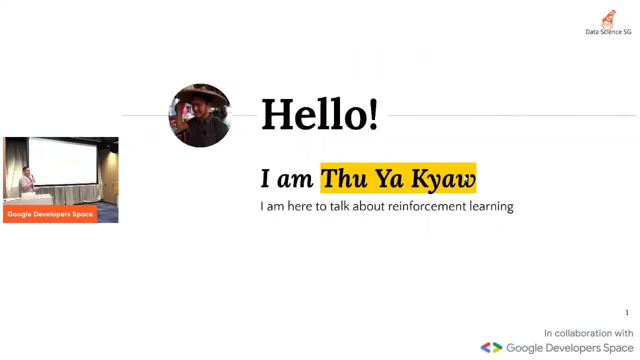 Can we put together our hands to welcome Tuya? Thanks, Evan, Hi everyone. Thanks so much for coming this evening. I know you have a lot of other things to do, but you decided to spend the time with us, So yeah. 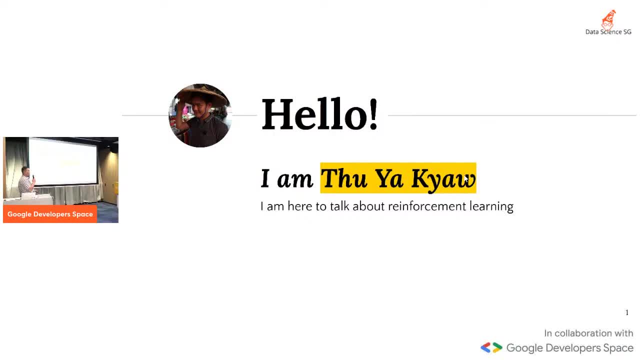 Thanks so much for it. And yeah, And I am here to talk about reinforcement learning. Like there is a lot of discussion on speaker bio and stuff, But yeah, Today I am just here to talk about reinforcement learning, So don't worry about that. 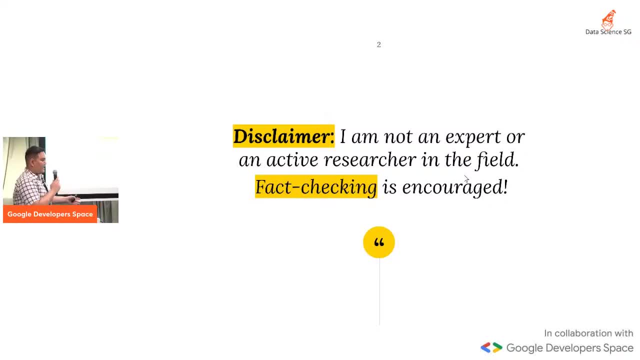 So- and I am not an active researcher or expert in reinforcement learning- I am not using it for my work. So, yeah, Try to do a fact check. Make sure you know you consume the content. I am trying to do my best, but it might not be 100% correct. 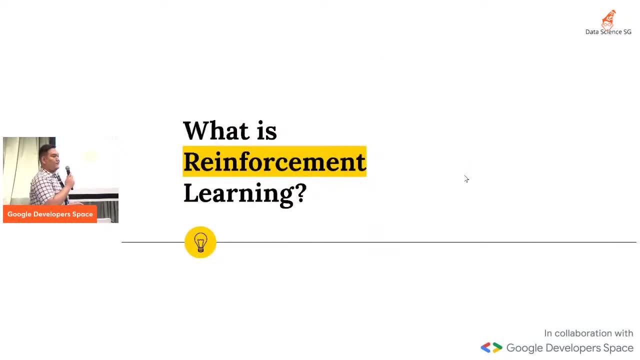 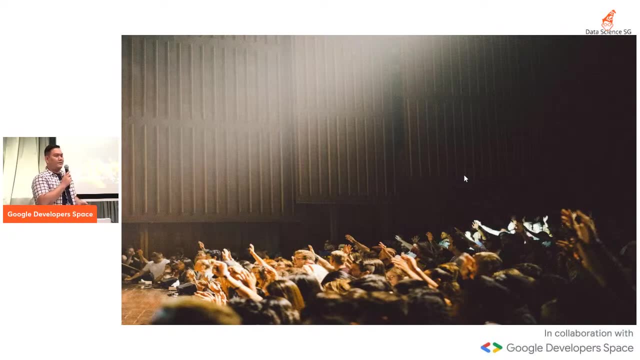 Just to be sure. So yeah, So what is reinforcement learning? Right? May I have a show of hands? Anyone heard of reinforcement learning before There is a few Wow, That's a lot. Then I think the content I cover probably will be too basic for you. 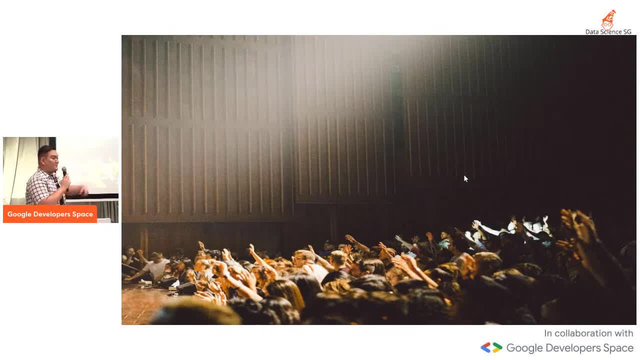 I am sorry if that is the case, But I will try to be, you know, more active and, you know, try to kind of give you some of the things that you might find useful for that. So, in a nutshell, reinforcement learning. 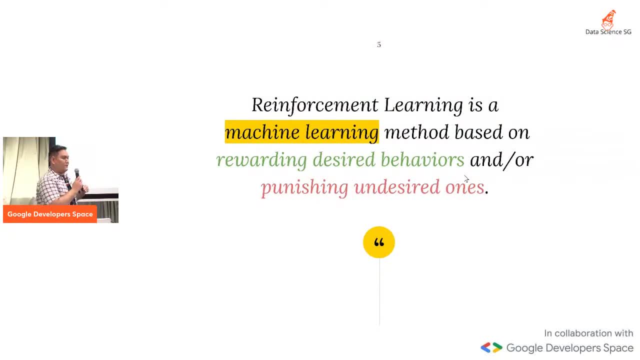 Reinforcement learning is just a part of machine learning method that you know. you reward the good behavior and you sort of punish the one that you do not desire to do. So, instead of training from your past data, you just let it explore. 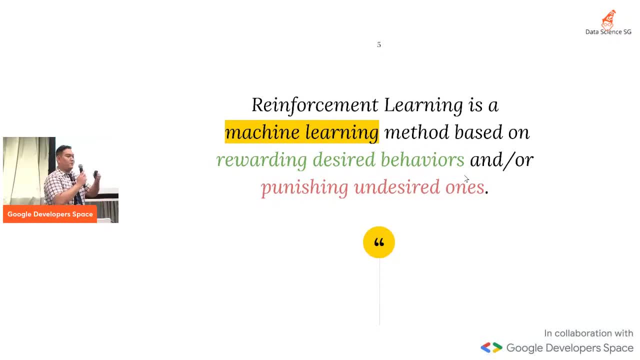 So in reinforcement learning we do not really make model and we do not call that thing a model, We call that an agent. So imagine you are like a toddler trying to learn things by interacting with the environment. So we will expand that idea in a while. 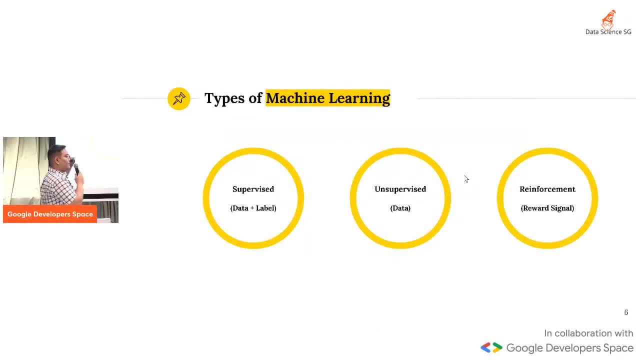 Right. So first thing, first, Right. So there are different types of machine learning. If you are already aware of it, please bear with me for a while. So there are supervised, which you have the data and which you have the label. 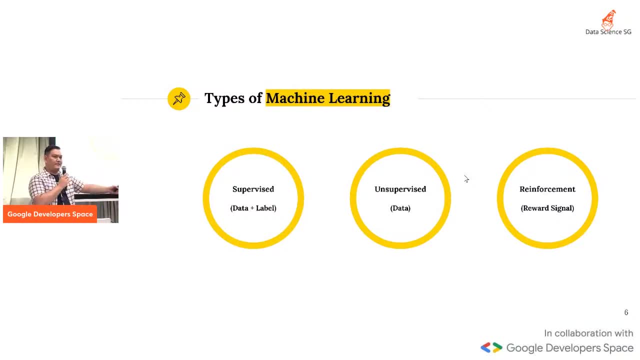 Right. So you just use label data. try to find the, try to approximate the function of it between the two. Right. Try to find the causation. Then you have unsupervised learning, where you only have the data. 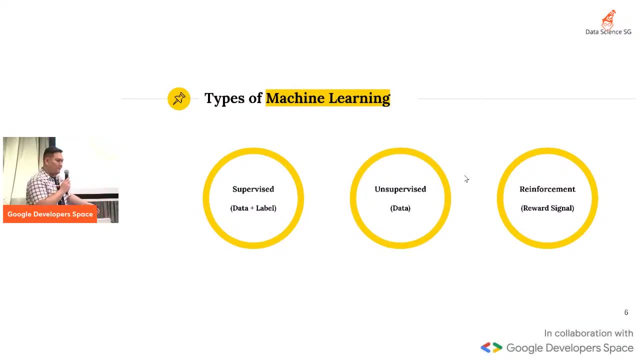 You have no sure what the labels are going to be. You try to find with the algorithm. give you the hopefully the best label or the correct label possible. So in reinforcement learning aspect, right, we do not sort of like we do not really use. 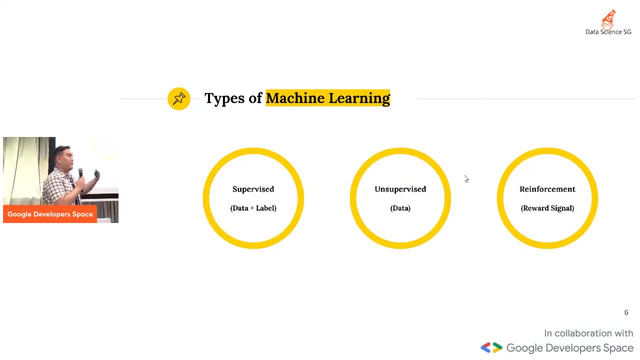 data because we sort of learn from experience and reward signal. So we try to find that reward signal so that we are doing the correct thing or the intended things that we are supposed to be doing. So there are some example. I am sure you have heard of AlphaGo before. 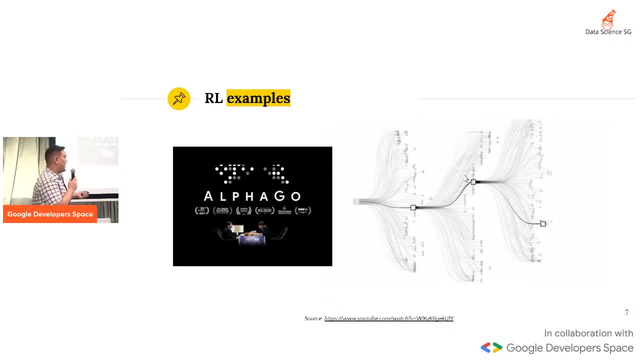 So this is like Go, Chinese chess game that is played by Google And it beats the. you know, some AlphaGo teams try to build the AI agent that can beat the world champion in AlphaGo, And that was like a long time ago. 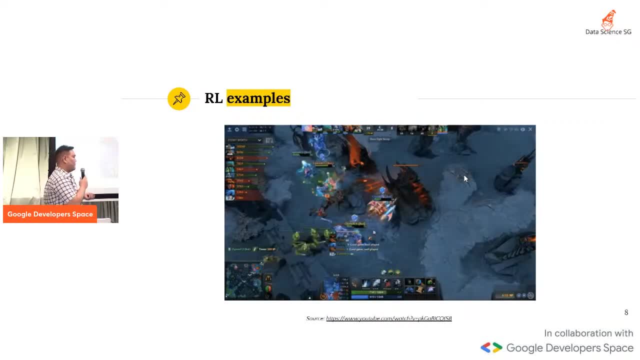 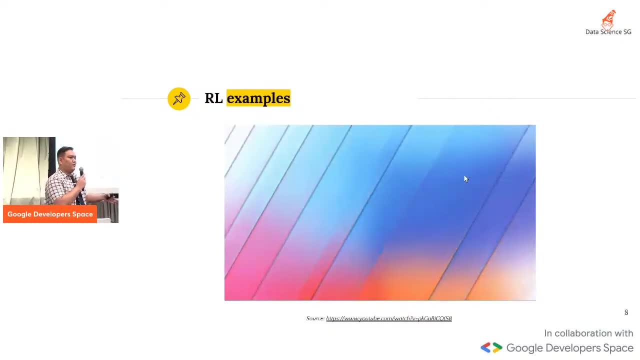 Right. So there are a few other things. There is OpenAI 5 that if you play Dota 2, you have probably heard of it before- This is totally run by AI and try to beat the world champion of Dota players And they are sort of like coordinating each other to get the maximize their rewards to. 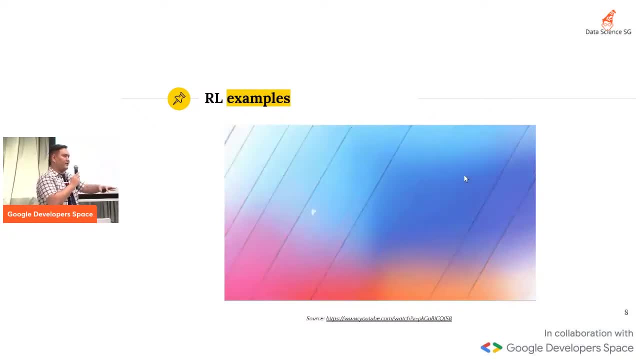 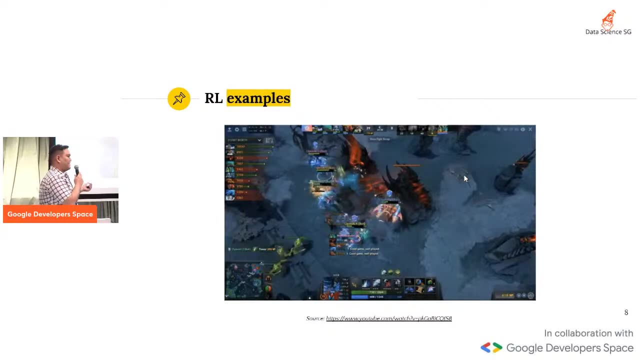 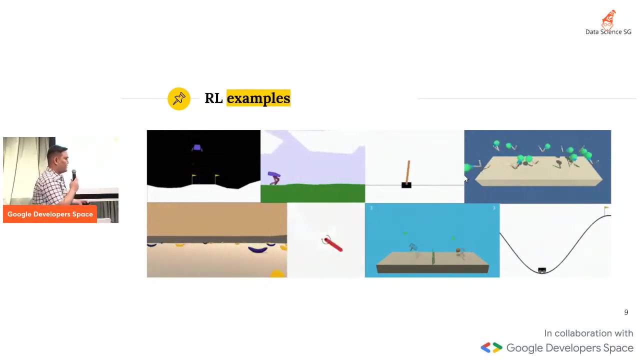 win the game. So there are like five agents interacting as a team to win other five players. So those are like very long time ago, Like when I started learning reinforcement learning. it was already there. So, and there is, of course, if you are a beginner, you want to get started on it there. 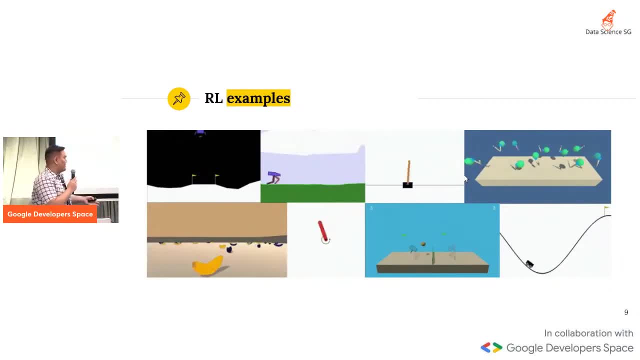 are some others games or gym environment that you can test it on. So in this example, like you are trying to land the spacecraft by just learning from the experience And make it go straight. So there are some tension. you know how much force you need and things like that. 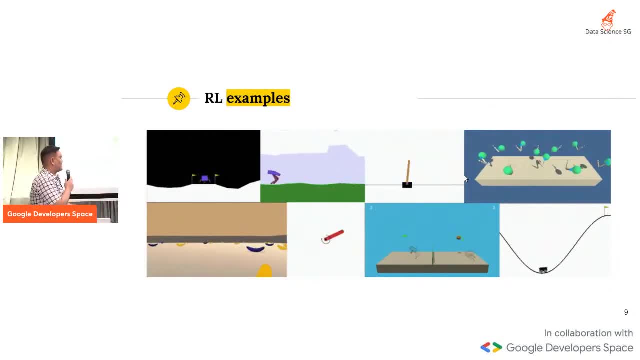 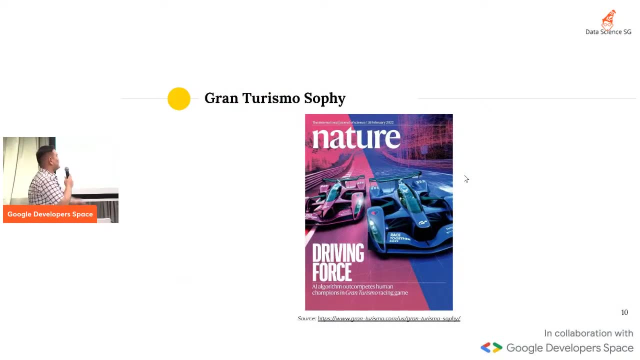 How do you drive the car all the way past to the edge of the slope and things like that. So those are like early days reinforcement learning Right. And recently there is this AI that can drive car really well And it beats the. it is in the game, by the way. 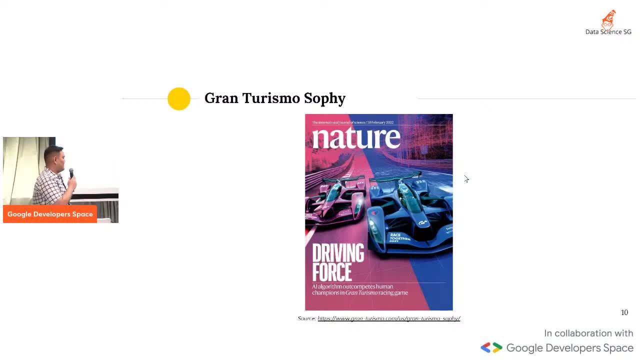 So they try to beat the human. that racing against the AI And the AI beat the human. So the human was not like someone who just thought that he is a champion in the game. Also, there is agent 57 that came out. 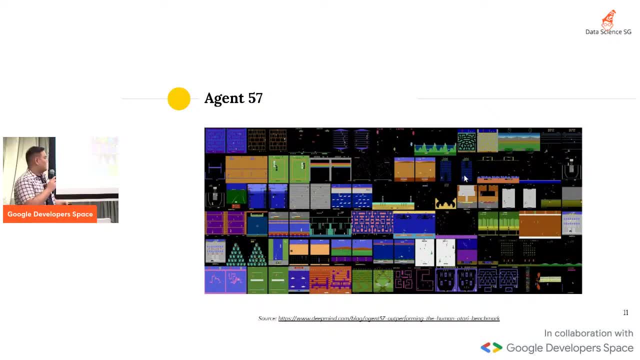 The agent that can play 57 games really well. Right, It is not just one game. So then they are even saying that this is like approach to the general intelligence, because you are trying to have this one agent that do 57 tasks very well. 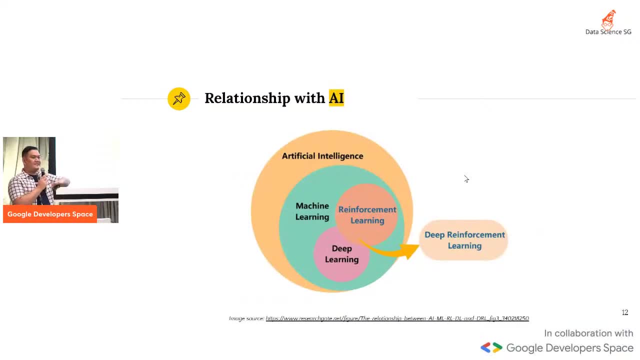 So enough of all the example, right? So how did this tie back to the AI scope? So, as we know, AI is like a big thing. Then inside of it, there is machine learning. So inside the machine learning, we have deep learning that we all love and adore and try to use it as much as possible. 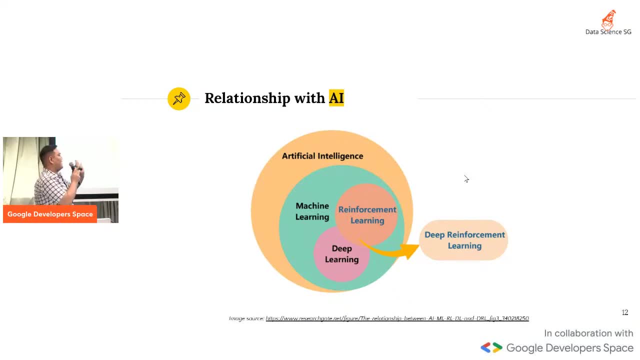 So then there is reinforcement learning, which is slightly out from the deep learning, But there is some overlap. So the overlap portion we call it deep reinforcement learning. So there are traditional reinforcement learning And there is like using deep learning to solve some of the reinforcement learning task, which we call deep reinforcement learning. 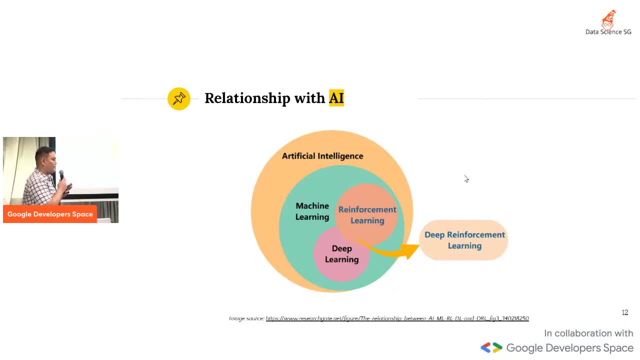 And for this talk specifically, I will cover the traditional aspect. So the next session probably cover that deep reinforcement learning. Okay, So for reinforcement learning, instead of having, like you know, colonial data, what we have is environment agent, the state of each of the agents. 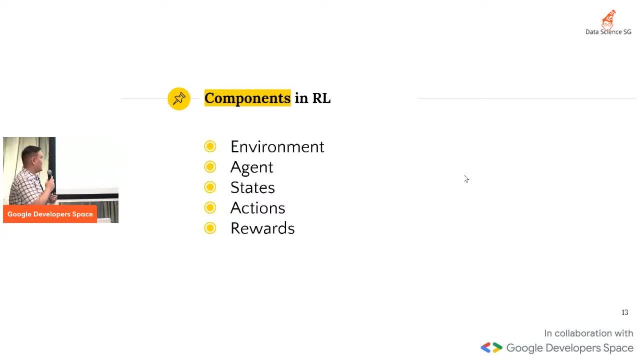 the environment, also the actions that agent can take and some rewards. So you do action A, you get some reward. You do action B, you get some rewards. Then you learn from the experience and then you improve yourself. Also, there is one important aspect, which is time. 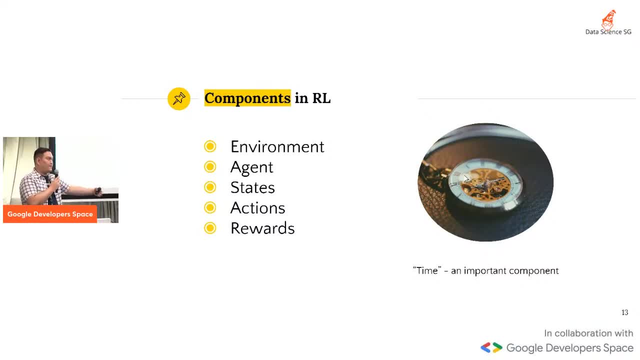 So, like you have to do certain task in a certain amount of time, So if your time is limited, then you might not be able to do the optimal solution. So you have to be just, you know, like you are studying for A. 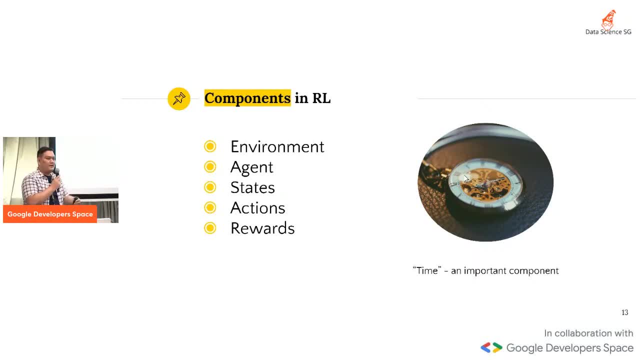 Like you are studying for exams. If you have unlimited amount of time, you probably score an A+, But if you have limited amount of time, you have to just dish some of the an important chapter. you will just focus on that important chapter and then you move on, right. 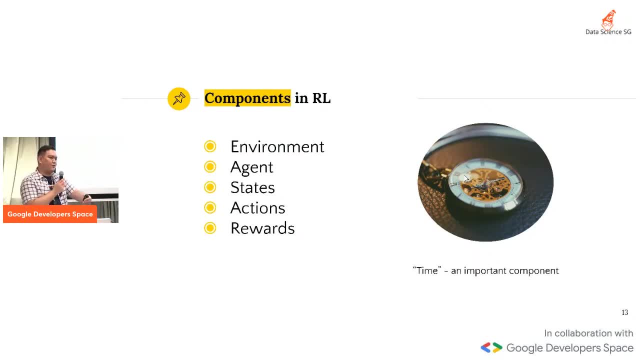 So, whichever grade, you get satisfied with it, because this is optimal solution, the best that you can do within the given time frame. So this is some of the things that we are exploring. So if I have to give you an example, right. 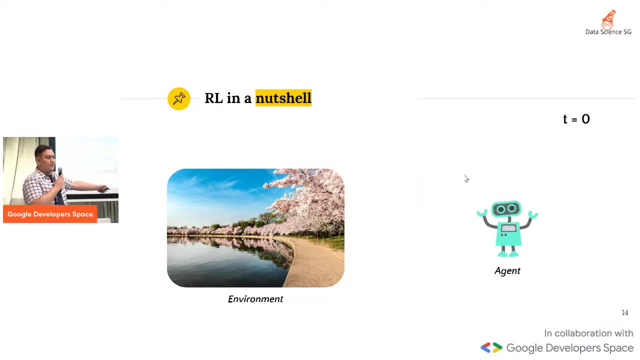 Let us say we have an environment here And we have an agent here which try to interact with the environment And we have, like time is zero at the time, right, So agent can query, state and reward from the environment. Then the environment can give them. okay, this is your current state. 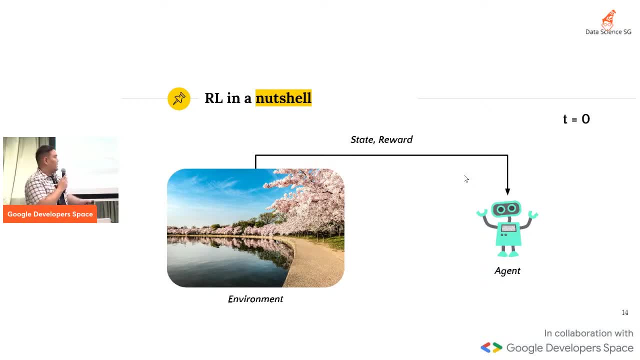 If you are here, your reward is this right? Then the agent can use this information, try to come up with the actions that give them like the best reward. So, once the action has been executed, back to the environment, it changed something in the environment, right? 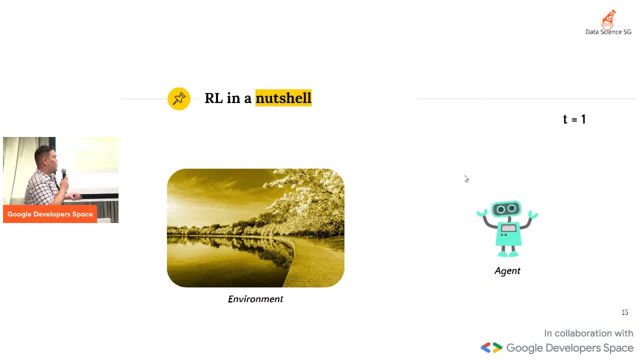 It may or may not change, but in this case it changed. And then it gives a new state and reward back to the agent. The agent then can decide what to do again, right, So the actions keep coming back. So that is how they interact with the environment. 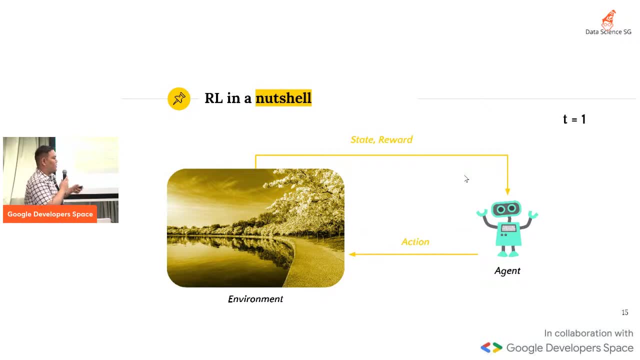 And also by using that you sort of learn it right. So every time you interact with the environment, you do something. You get it wrong, you get minus reward. You get it right, you get positive reward. Then you sort of adjust your actions based on that. 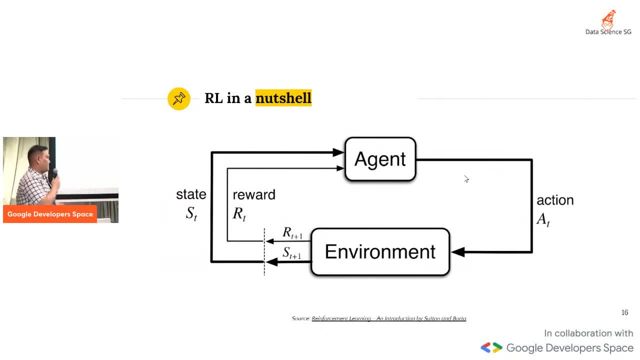 So this is in a nutshell diagram that I copied from Sutan Bhatua. So this is like a very good book if you are interested to read Reinforceable Learning by Sutan Bhatua. So this basically turns down two slides into one. 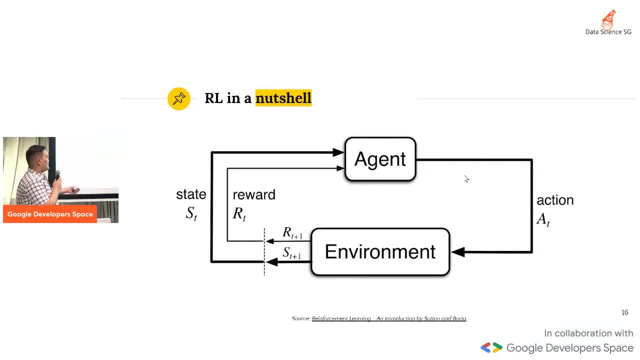 like very nicely drawn diagram. So it is the same thing, right, Like environment. So the agent gives you state and rewards And then agent performs an action. Then, once the action is performed, you have new state and new rewards for the agent. 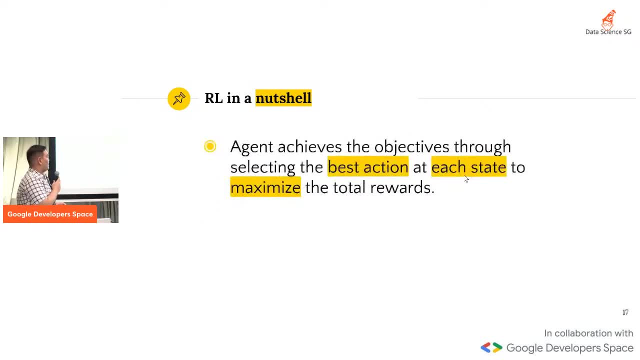 So the circle repeats. So, in a nutshell, agents achieve the objective that you want to do by selecting the best action possible with given the states right. So these states, I do this, I get this reward, But I want to get the best possible rewards. 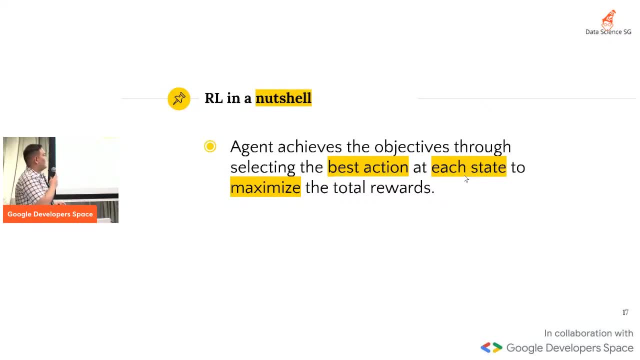 Not just any rewards, Any rewards that I can do. So this is pretty much summarized, everything that I will be explaining throughout this entire talk. But if you notice the best action right, How do the agent know the best right? So it can be any action. 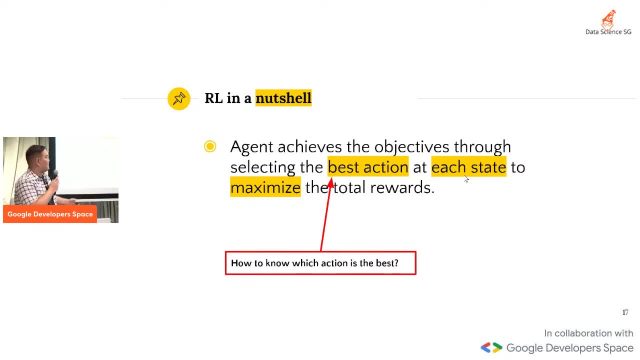 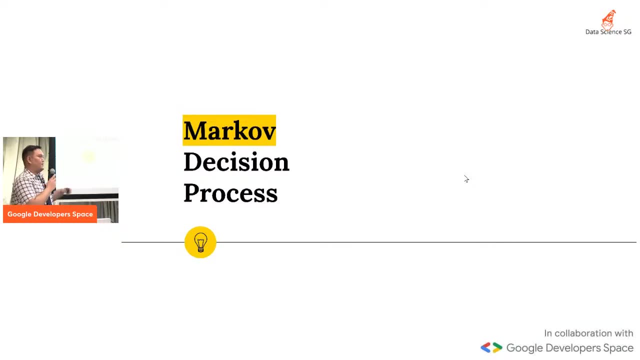 But what does it mean to be the best action to take? And a lot of scientists have come up with this idea of macro decision process. So it was done. We have our time And this is like simple idea of you know. 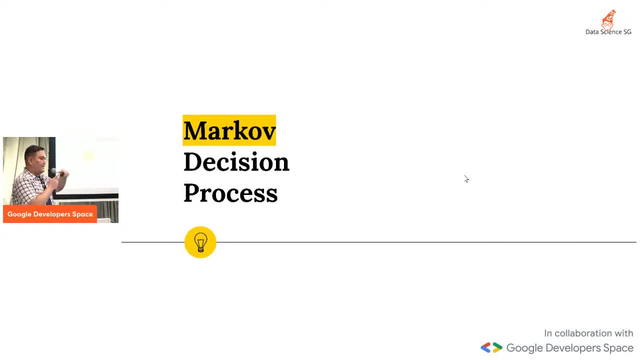 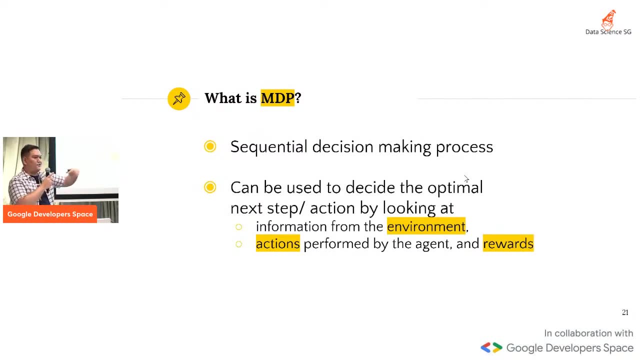 try to frame that problems into state environment And then you try to chain it up. So the idea is pretty much simple. So this is like a sequential decision-making process, So it is like a loop, right. So in this state I do this. 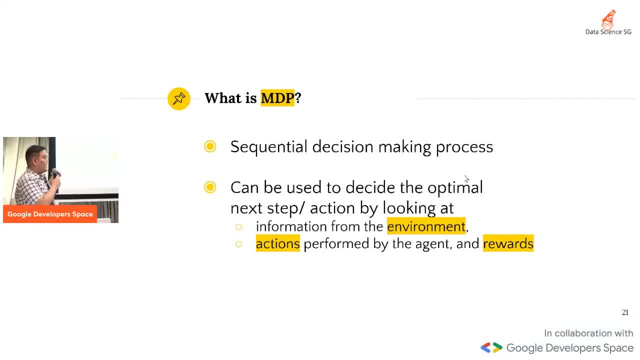 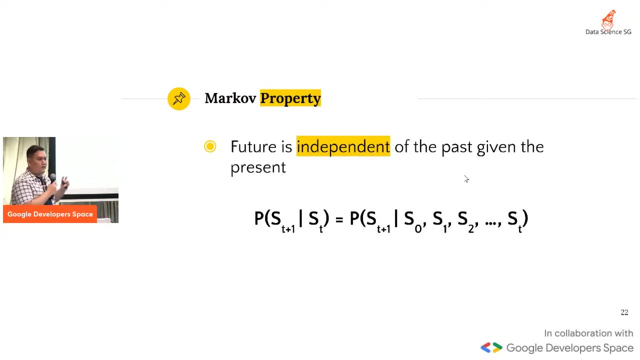 In this state. I do that And it can be used to decide the optical or optimal next steps based on the environment states and the action performed by the agent Right. And it does using one assumption: It is called Markov property. 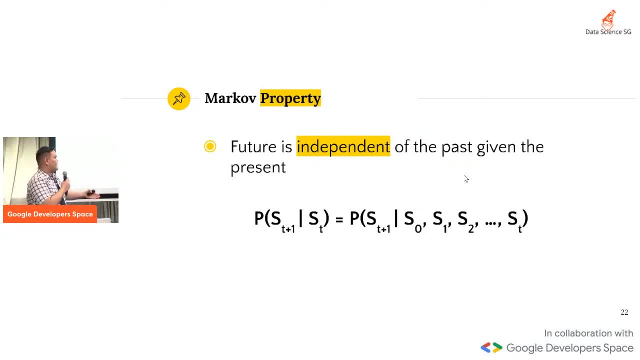 So we are only assuming the next states is only dependent on the previous states and not the others. So I will give you some example about this, But hopefully after the example probably give you a better idea of what it means. So if you are from math or background, 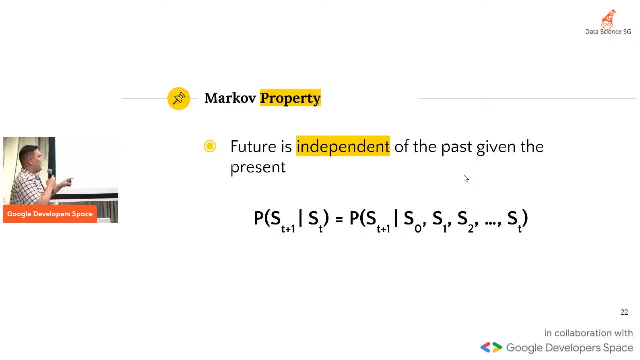 you probably can read this formula. So pretty much the next states is only reliant on the previous states, not the entire history of the states from all the way to the start. So your decision to what you want to eat next it does not depend on whether you are born in Singapore or some other country. 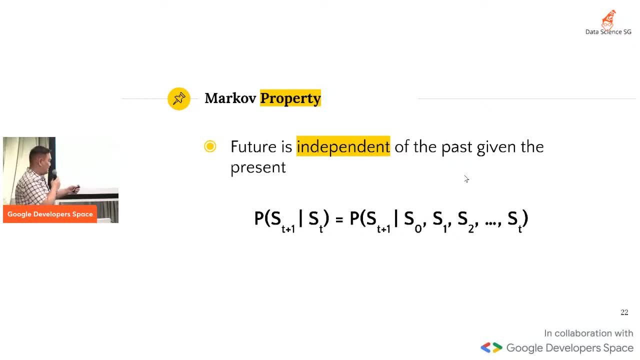 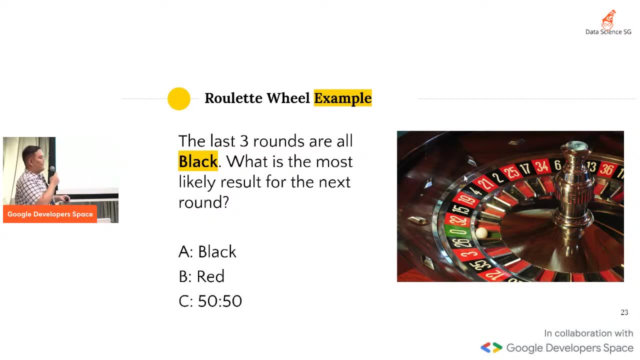 So it only depends on your mood at the time, Something like that. Yeah, So this is some example. Imagine you are in a casino, right, And you try to see the history of this ferret wheel. The ferret wheel. if you do not know. 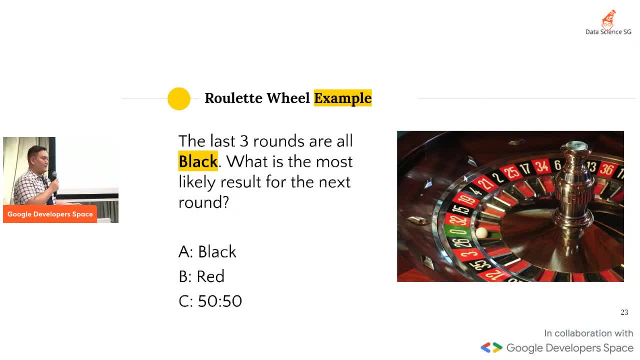 there is like red and black that you can bet on. So if the ball rolls and then hit the black and then you sort of bet for the black, you get the money, something like that. But imagine that the first three rounds is already black. 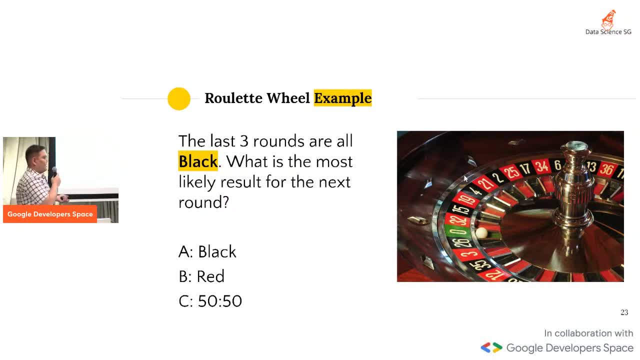 What do you think will be the next round results? Anyone think it will be black. You can raise your hands. Anyone thinks it will be red, Because you know, due to the randomness, already three black and the next one has to be red. 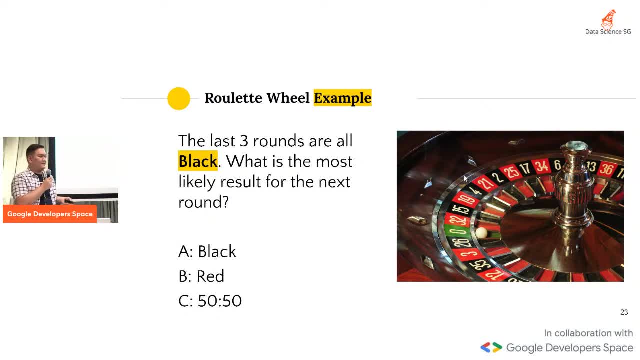 Or people think it is just 50-50.. It does not care, It does not matter whether it is yeah. So most of the participants are correct. I did not get this right the first time So I was like, no, it has to be black because you know. 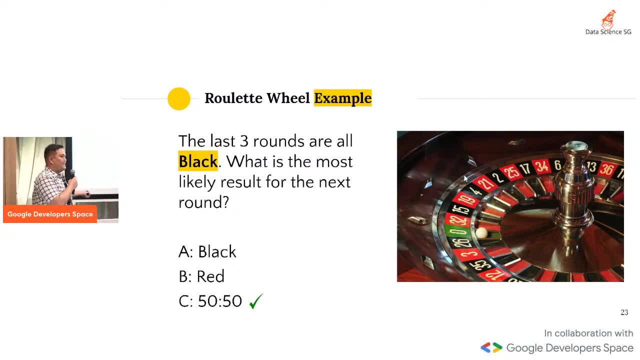 it is a rig or something right, But it does not matter whether the history of it shows you that a lot of black or a lot of red, it stays 50-50 every time you spin the game, Unless it is temper anyhow, right. 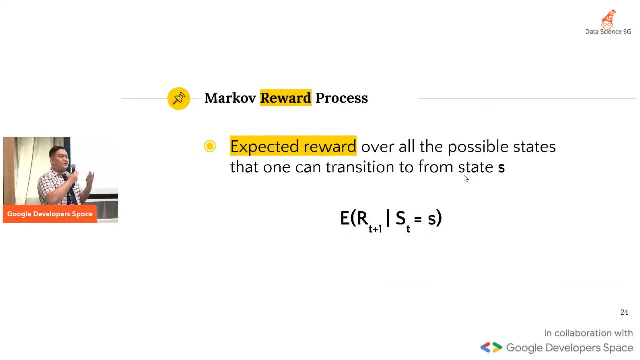 So that sort of gives you some- you know- intuition behind the Markov decision, Markov property right. It does not have to depend on all the previous states, It only depends on the current states and we are good with that. 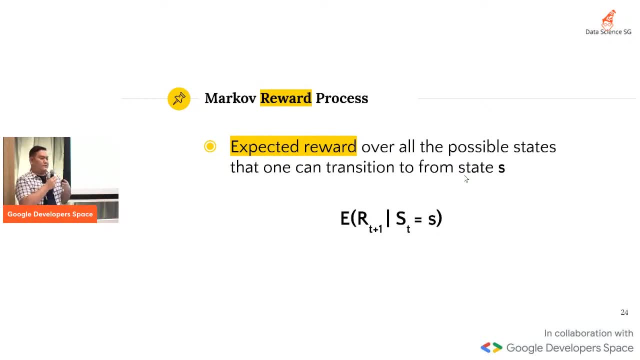 So and of course you need to work with reward right. Do not just environment and states, So rewards. it sort of gives you like expected rewards. So if you do action A, your expected reward is 10.. Action B is 5, something like that. 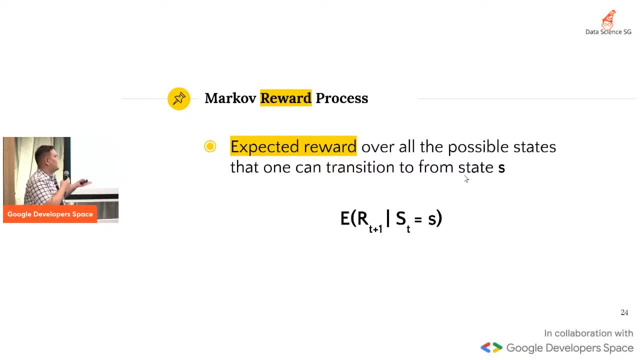 So how do you calculate that? So you have to use some formula to calculate and then every possible, like possible, stakes that you can transit to should have tied to a reward. If not, you cannot decide right, So you have to agent have to decide the best possible rewards. 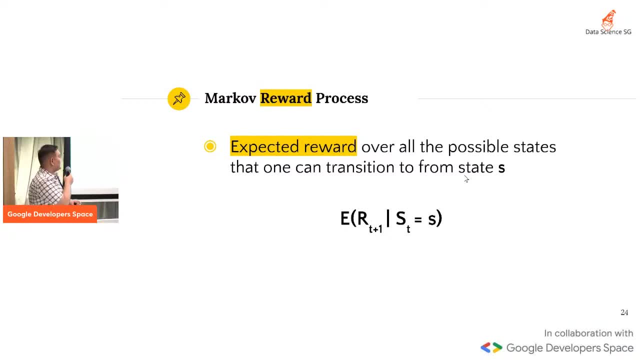 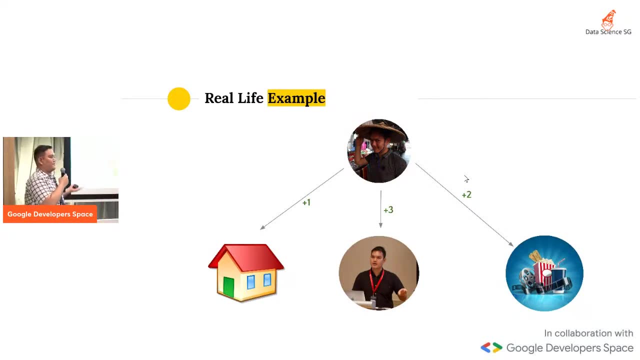 stakes or action to do that. So, for example, right, I could be at home and I could be watching a movie at the cinema, but I could be here talking to you guys. So, and the rewards for me is sort of give me three points, in a way. 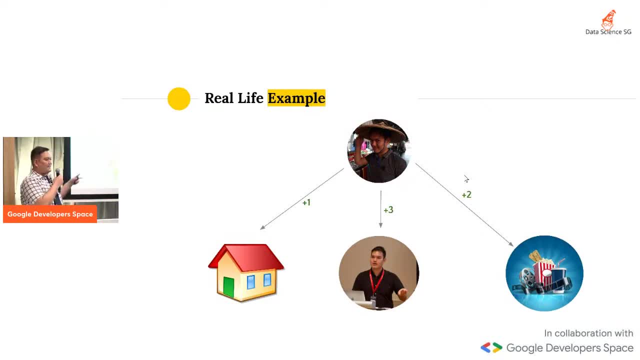 It is arbitrary, by the way. So I like to talk to people, connect with people. That is why I am here, right? If my rewards systems are, otherwise, I would probably be at home watching a movie, right? So if this is my agent, I choose the middle one. 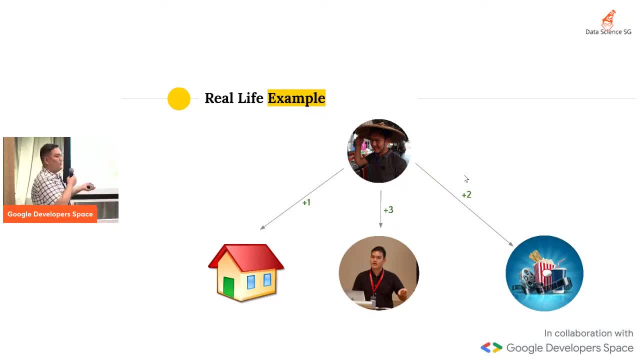 because it gives me the best reward. So that is how we frame the problems and rewards and the stakes all tied together. So generally it is that. So you have a state, what state you transit to, how much reward do you get from it? 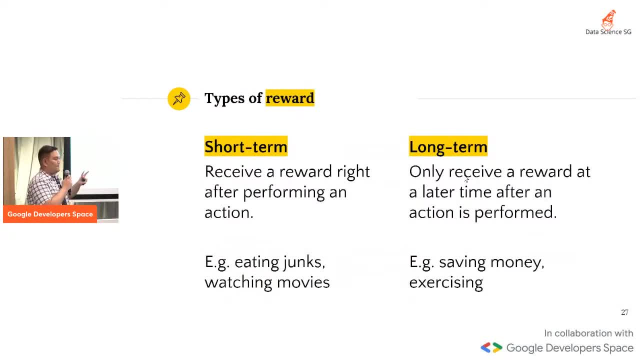 So there are two types of rewards. It is applicable for our real life as well, right? You have short-term rewards, which you definitely get after you have done it, And there is long-term reward, which you can only get it after a while, right? 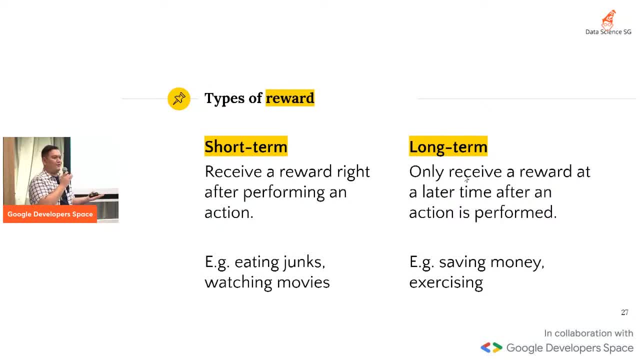 Example can be: eating junk food gives you like satisfaction right after you finish it, but after a while sort of give you like more health problems and things like that. For watching movie may you fall asleep better, and you know, sometimes you cannot really sleep. 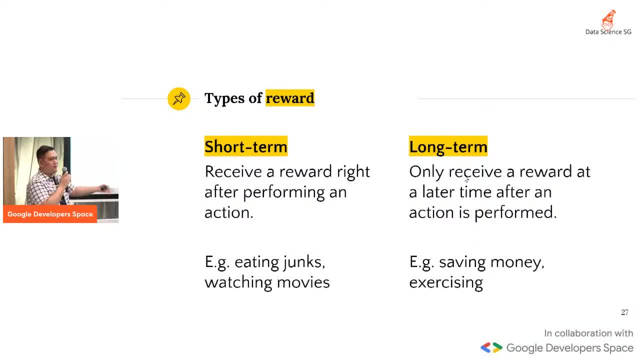 because you have been watching some of the episode and sort of give you health problems from there. But for long-term, like saving money, exercising, sort of give you like, do not give you the intermediate rewards, but in the long run it is better for you. 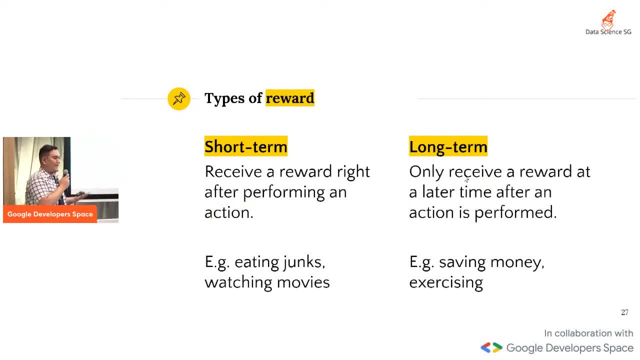 So we need to like frame this in that sense, so that the agent is not greedy to just pick whatever rewards that give him the best for that state. It has to consider as a whole, right Like what is the task, And then I need to consider the long-term effect. 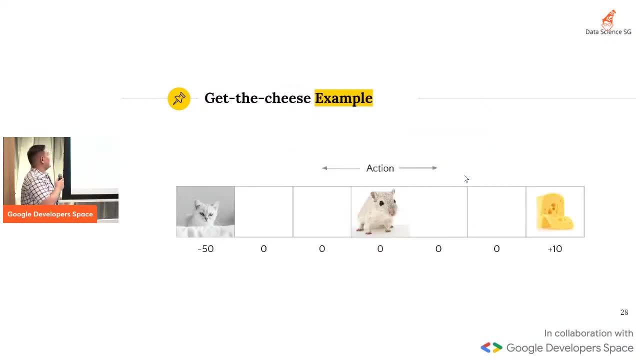 not just the short-term effect. So, yeah, I came up with this example, sort of similar like. so our agent in this example is the mouse, and the mouse has two choices to make. Our goal is to reach to the cheese, right. 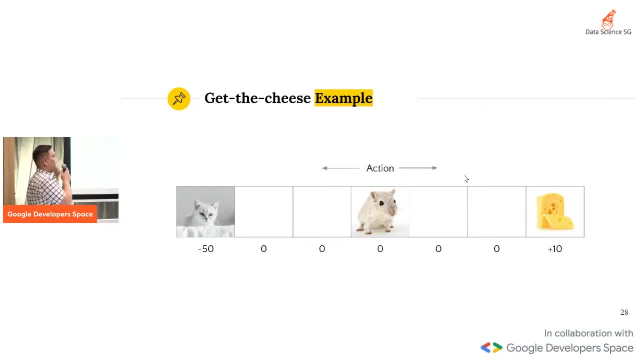 And if we do wrong action, it reached to the cats and then your agent died, right? So that is pretty much what I want to say. So I frame the thing so: we have the environment, which is the grid, and the agent is moving left and right. 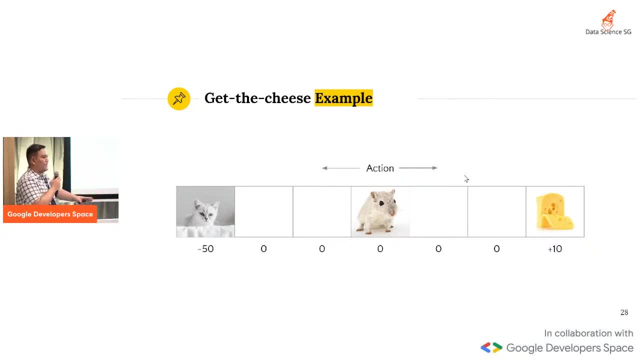 You have rewards for each state, right? If you reach to the cheese, you get 10 points. If you reach to the cat, it is pretty much 50. So you sort of like, do not get anything and you probably die from it. 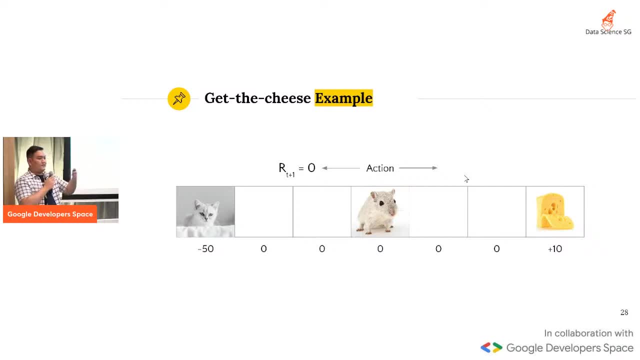 So from here, if I am going to take the agent to the right, it only gives me zero rewards. Or if I take to the right or the left or right, it gives me the same rewards, right? So we need to come up with better problem framing. 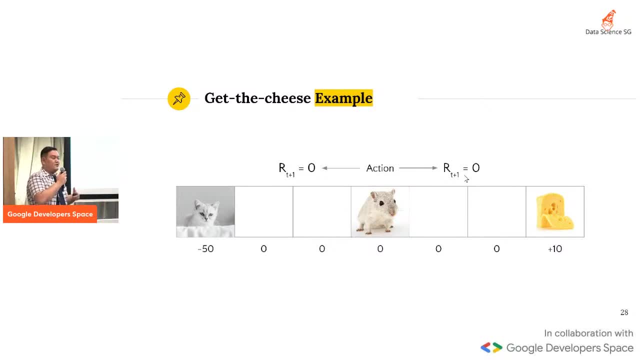 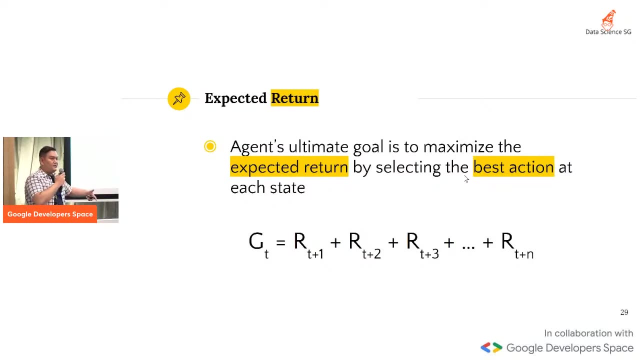 because this does not take me anywhere, because whichever action I choose, it just gives me zero right. So they come up with this thing called expected return. So, using that long-term reward in mind, they frame it into that. So this basically tries to maximize your return. 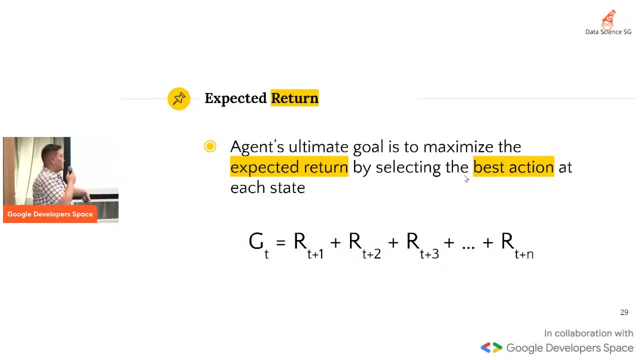 by combining all the rewards as possible. So, until you, from the position that you are in, the position that you have, all the way to the goal, how much are you getting it from? How much are you getting it from? So, if I go left all the way, how much reward do I get? 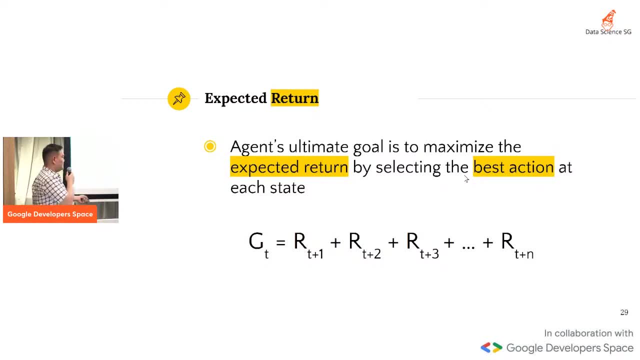 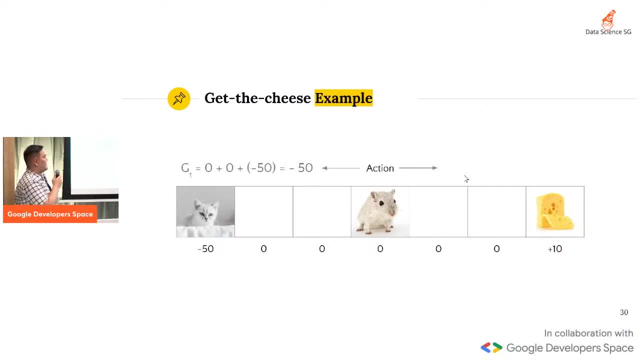 If I go right all the way, how much reward do I get? So this is the formula for that. It is pretty much just a summation of it. And then if we do that right, So if I am going to the right, 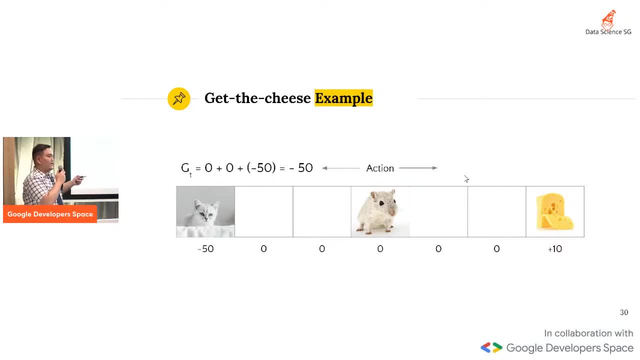 I sum up all the way and it gives me minus 50. So I choose not to go there. compared to my left, Which is giving me 10 rewards. So as an agent in that environment, I know where to go, So I will choose the left option. 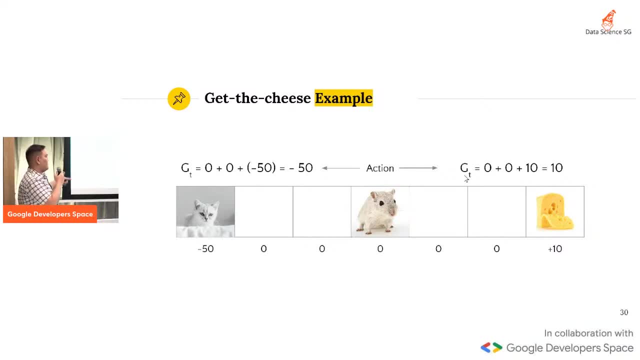 But this is only transparent to us because we know from like you know, we are 3D beings, So we see the 2D world is like this way. But as an agent, as a 2D, you can't see right. 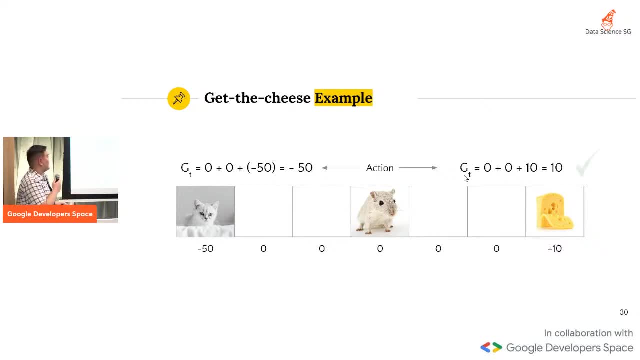 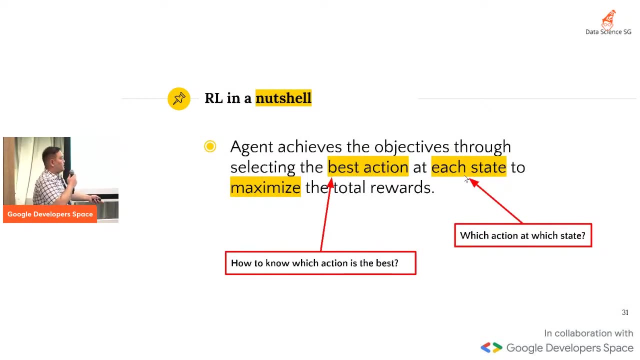 You can't see that kind of thing. So how do we model that? Okay, So remember this slide. So how do we know the best action? But we don't only need to know the best action at that stage, We need to know best action at every possible stage. 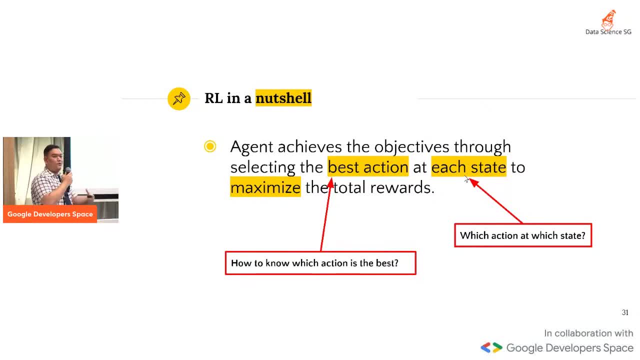 So that if I ever get into one position, I know where to go. Not just for like as of now. I need to know my future right, So that if I move here, where do I go next. So they came up with this term called policy. 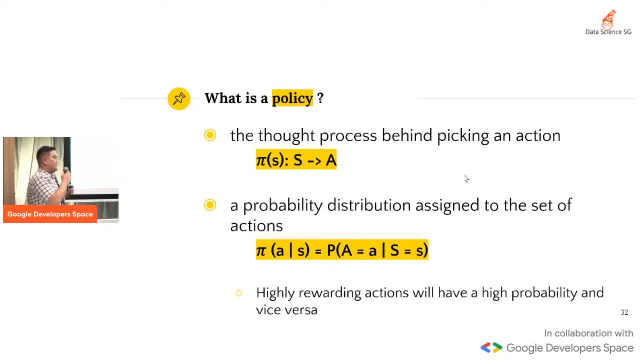 So this is something like distribution assigned to your action. So, like every stage- let's say in this case, to get the cheese example- it has two possible actions that you can take And then, based on the rewards it assigns, the probability of the agent. 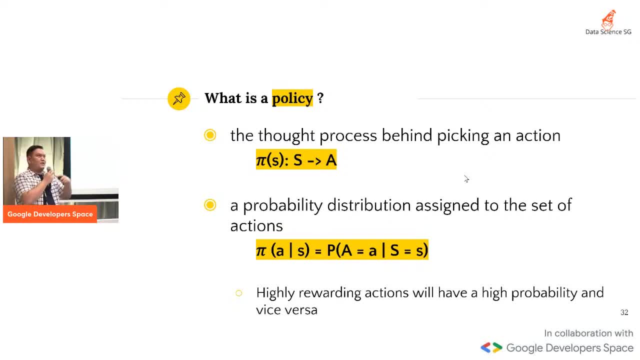 that should take the action. So left side has positive rewards. So my probability of taking the action for the agent should be higher than the right side, because the right side is diminishing return. So there is something like that. So the highly rewarding actions. 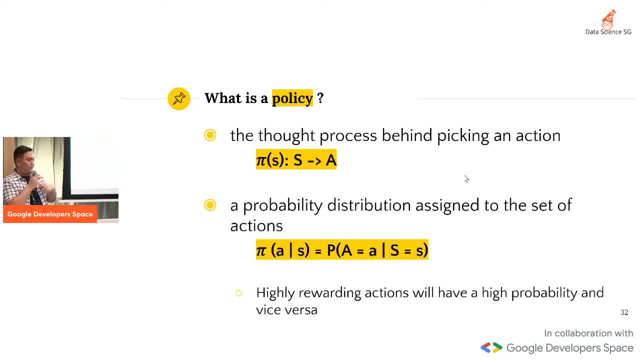 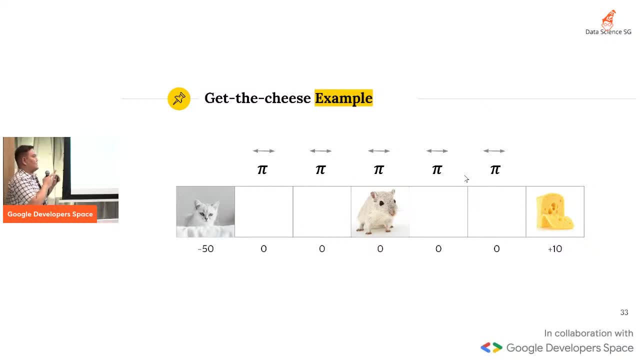 will have higher probability compared to the right side one which gave me the low rewards. So we use policy as pi in the mathematical or symbol way And the pi initially. you can be choosing left and right, So these are like action table in a way. 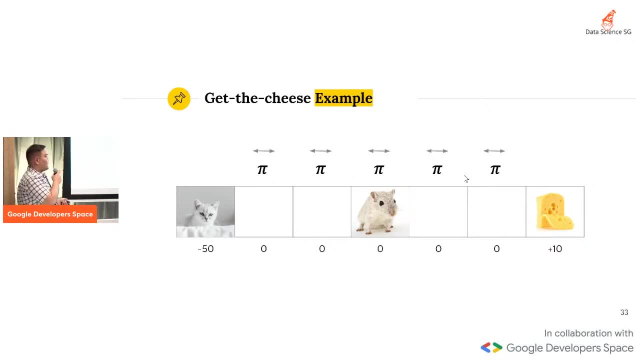 So you could choose left and right from these states. But after we have done that, but after we have done some calculations or trained the agent, then the optimal policy should be always to go right. It does not matter where you end up. 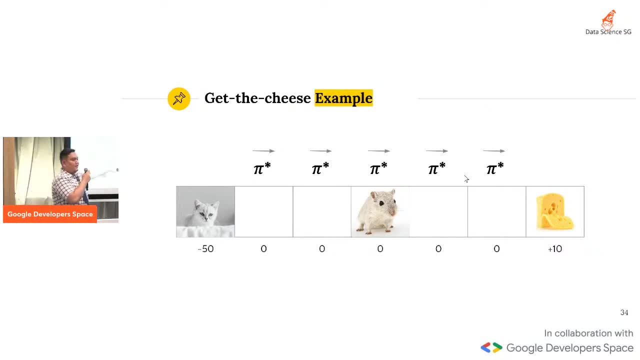 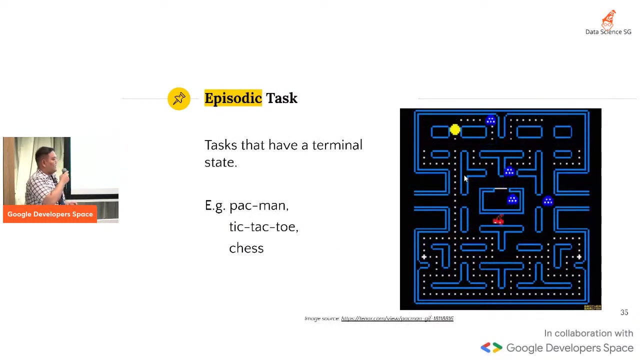 So the agent could be here, but the policy should tell the agent to just go left. You should never go right, because right has the enemy that will kill you. So that is something that we have to work on And the task itself. 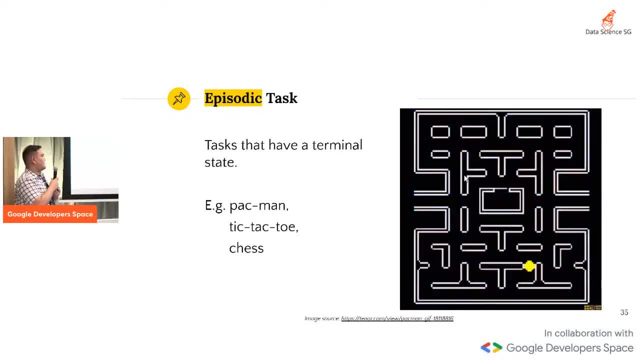 the task that I gave you just now, the get the cheese task, is pretty much episodic task. So once it is done, it is done. There is no continuous right. You reach the cheese, the task is complete. So these tasks are called episodic tasks. 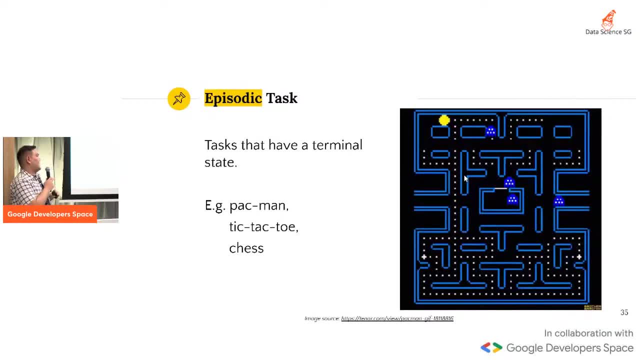 It has the terminal states and pretty much similar to like Pac-Man chess tic-tac-toe. So all the games are like. most of the games are episodic tasks, But there are other tasks. They are just continuous tasks, right. 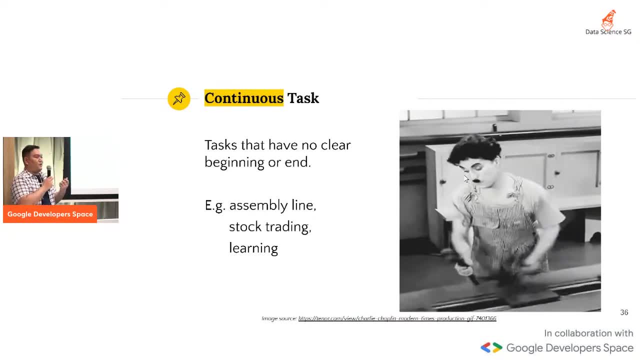 So if you are building a robot in a factory, the task does not really end. It is keep on going right. So it is like assembly line stock trading never ends. It is go up, go down And, of course, learning right. 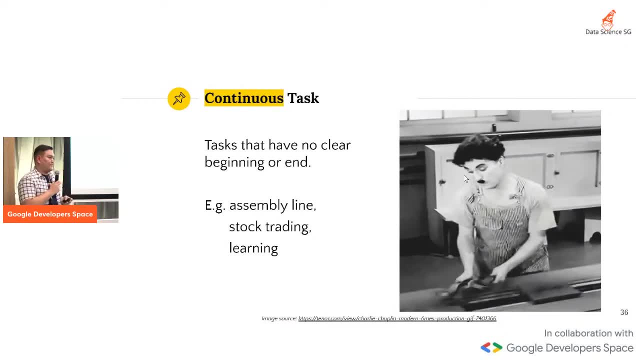 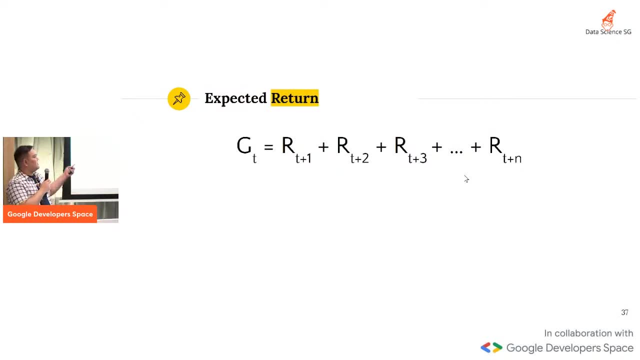 That is why you guys are here spending your time on the evening to learn. So learning never ends. Keep on going, right? So we cannot just use this formula for continuous tasks, because you never know. You do not know when it is going to end, right? 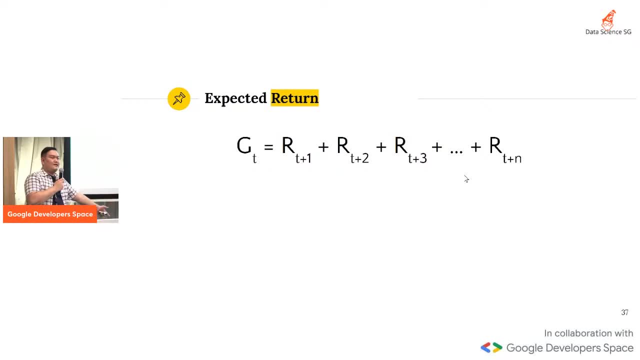 You do not know the t plus n, So it keep on going to infinity right. So you got to do something about this, And one way to fix it is by adding this discount factor, So they call it gamma, And discount factor is ranging from like 0 to 1.. 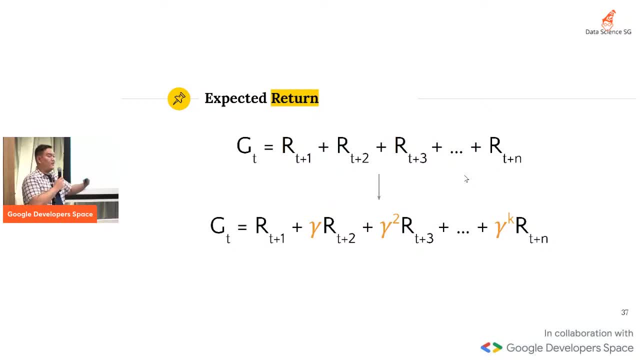 So if you are putting a 0,, then you are very greedy. You only take out the max reward at one states. If you are putting 1,, then you are considering all the possible future rewards right. So you have to balance that in the aspect. 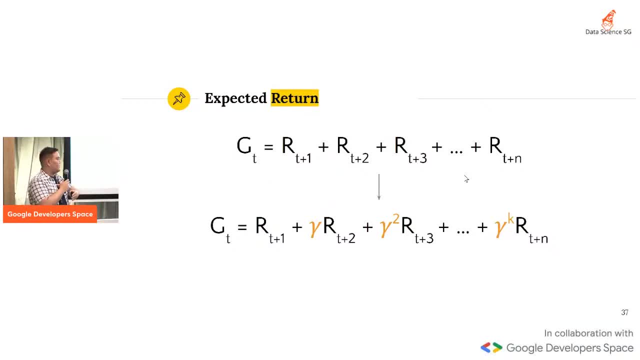 So if you are going to the infinity, the infinity part will be like very much to 0 and you sort of like do not care about that. So this is like very beautifully done in the mathematic formula. So the gamma value is like 0 to 1. 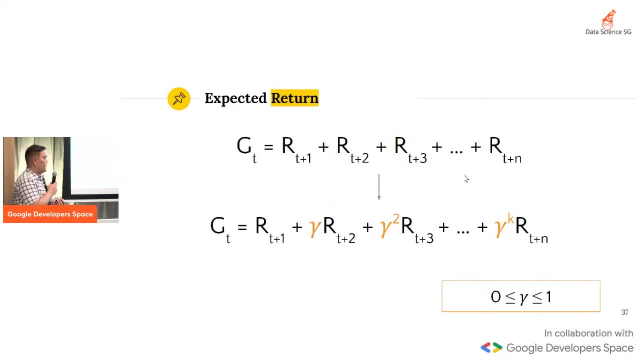 and anything in between, So you can just choose whichever that works for you. So it is like hyperparameter tuning here. right, Try to tune that gamma so that you have the best reward policy and your model train faster. So in reinforcement learning, 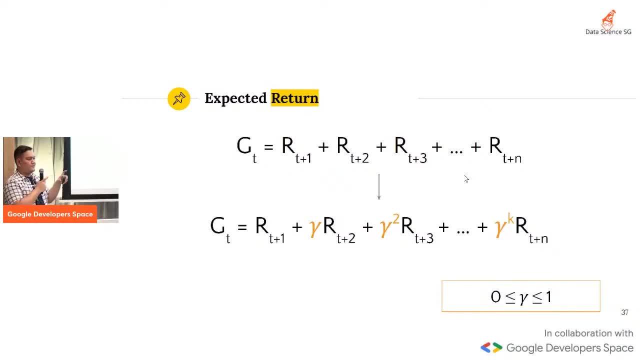 we train the agent, not the model, And the model terms in here is used for something else, not for the agent, So there is something that will confuse you if you are from like machine learning or, like you know, like supervised learning, expert learning. 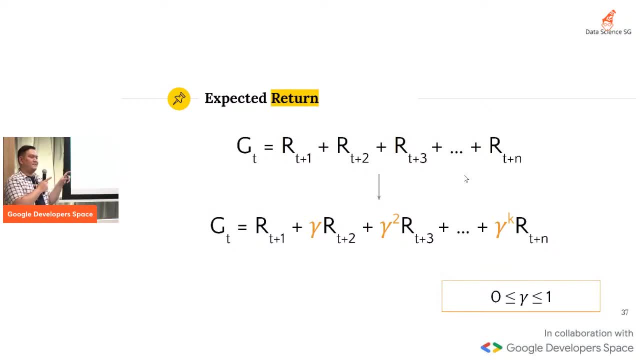 The model means the function, but here is model. Model does not mean the agent, So agent is agent, The model is different. Okay, So I talked about policy before, but the policy is only the table right. But how do we evaluate which policy is the best? 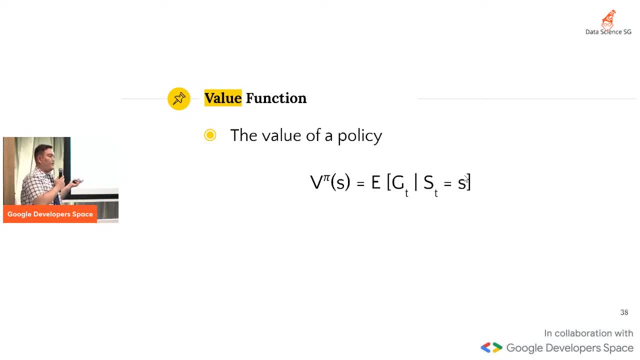 So imagine you are the mouse in the story and you need to know the map right. Where do I go? The optimal policy is always go left, So that policy is optimal. but how do we know that is optimal right? 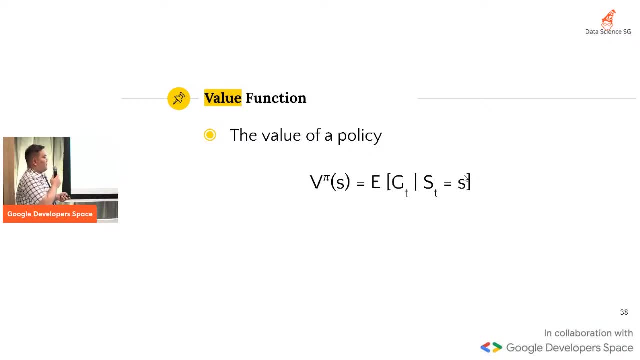 So we cannot know for sure. So they come out with, like this formula to come out and like: evaluate the policy between them so that we know the optimal policy. So the optimal policy is value function that we calculated and whichever give you the highest return right. 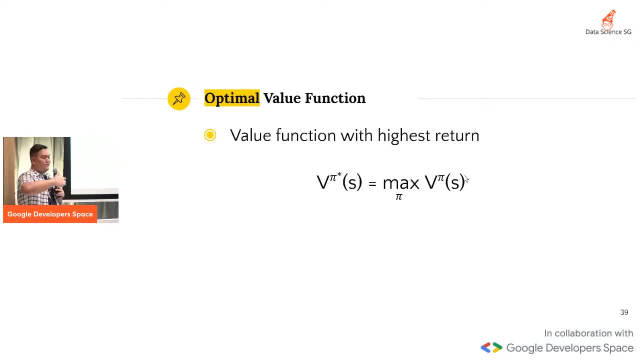 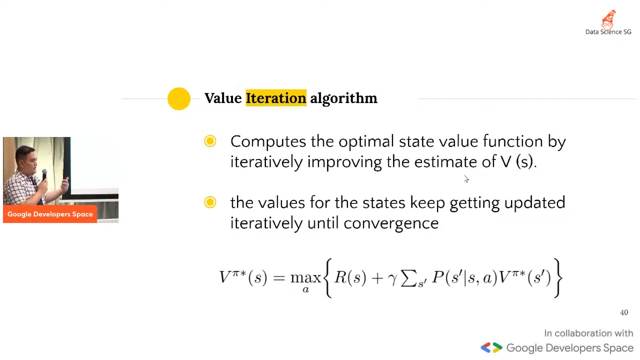 So I calculate the discounted value over every states from my current states. whichever give me the max return, I will choose that path. So yeah, So there is these algorithms that we use. It is called value iteration algorithms, As its name sounds. 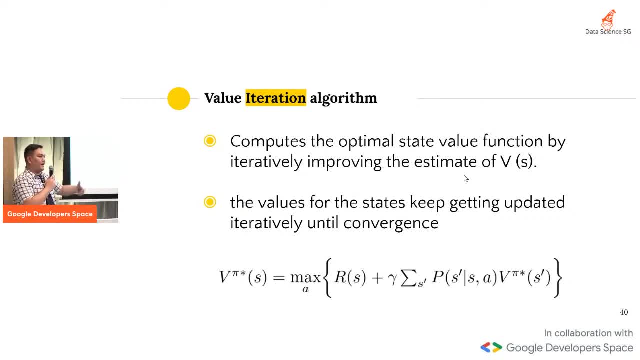 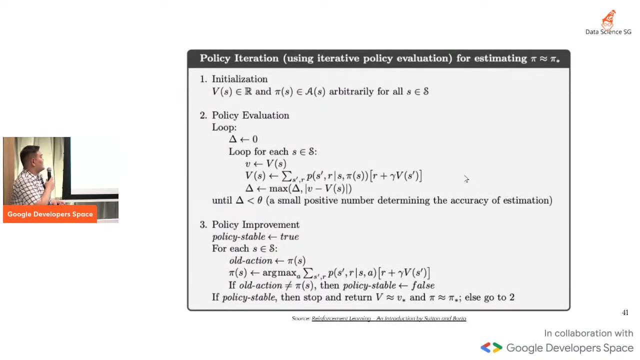 it is key on iterating until you find the best or the optimal policy. That is like every iteration. the values of this policy will get updated until it converges into like very small difference that we define. So this is how it looks like. 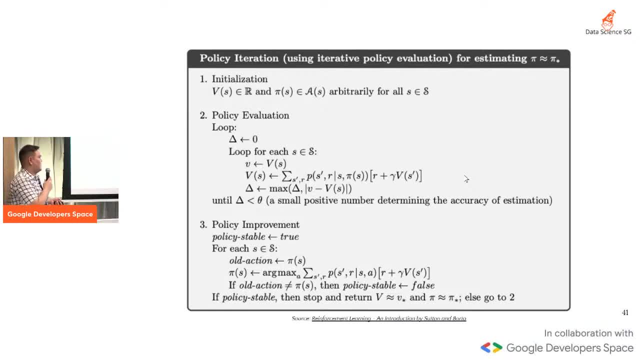 Although it looks very complex, but if you really read it it is not that complex. And all these terms that I use here is reference to the slides that I just list down. right, We have the rewards. We have the reward for the next states. 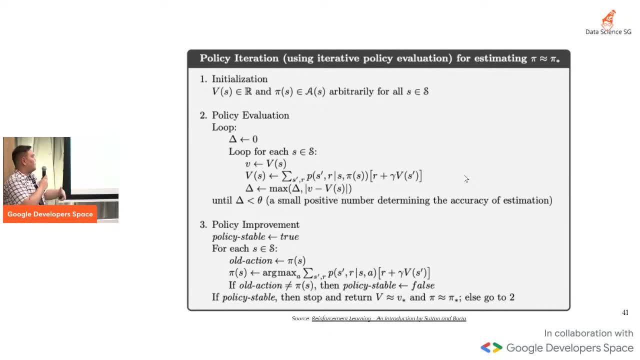 with the probability of it. We are summing them up. So every policy you will have an action table. So these states, state 1, 10 left, state 2, 10 left, etc. You just sum up all the rewards for each states. 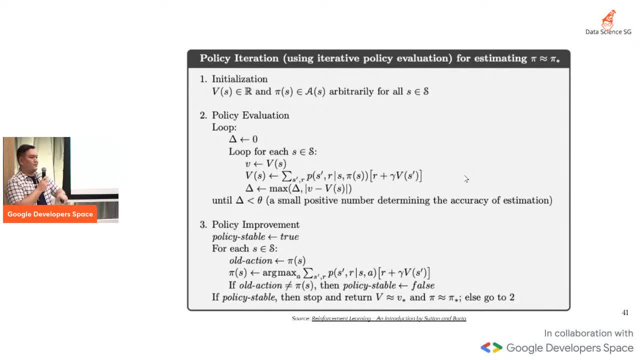 and then you have the policy value. You try other policy- maybe 10 left, 10 right, 10 left, 10 right- and compare their value, See which one is better And whichever gives you the highest rewards, because we work with rewards. 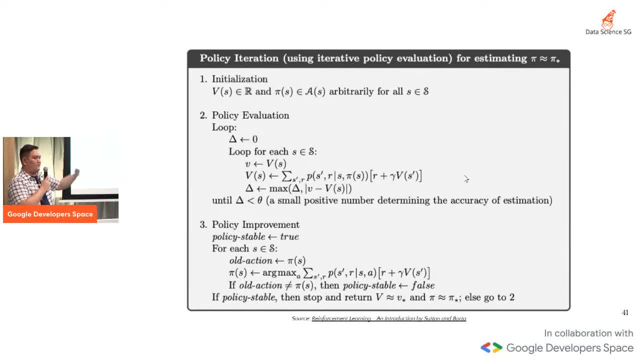 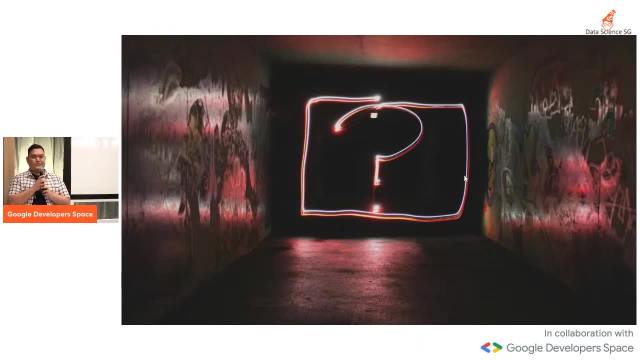 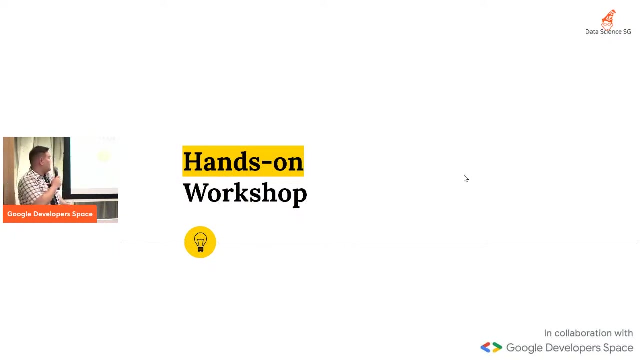 then you win. So the policy will be the one that gives you the highest Right. So, before I go any further, anyone has any questions Time? Is it time yet? Okay, Okay, So the next one will be the hands-on. 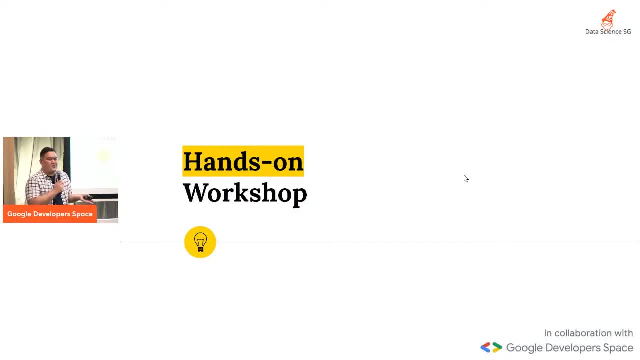 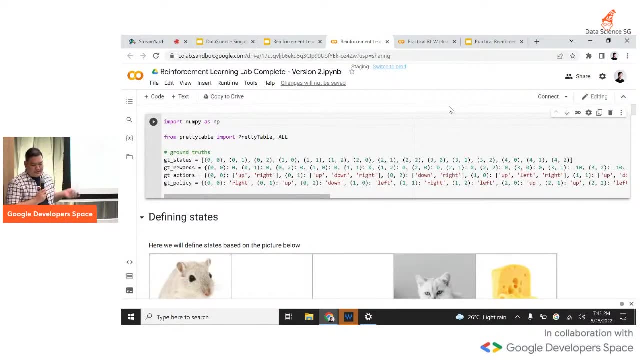 So I can't keep talking and never show you the code. So I also wrote some code to show you. You can. yep, I will send you a link of this one. It is pretty much quite simple to write. for this example only. 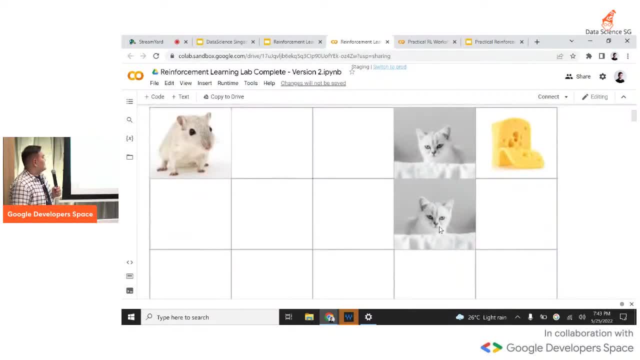 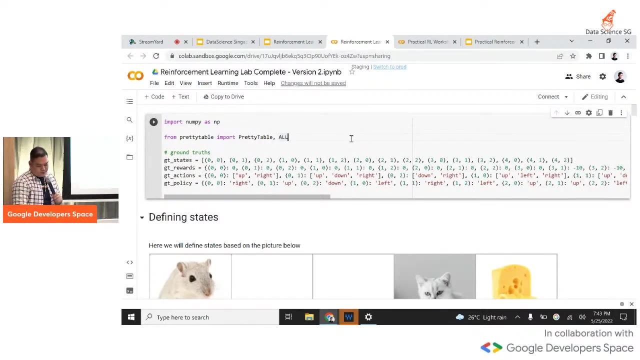 So what we are trying to do is: I expanded the formula, or the environment, into a grid So we can move up down left, right, And this is pretty much just ground proof, so that I know if I ever do some mistakes. 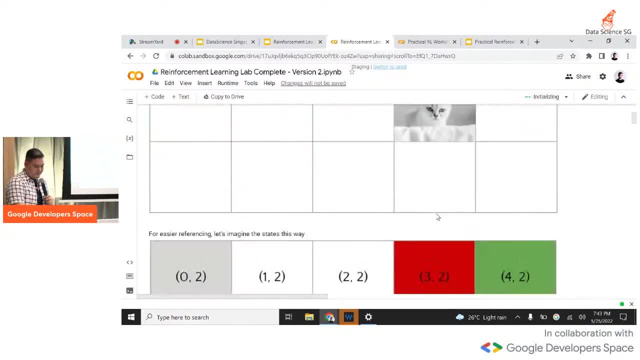 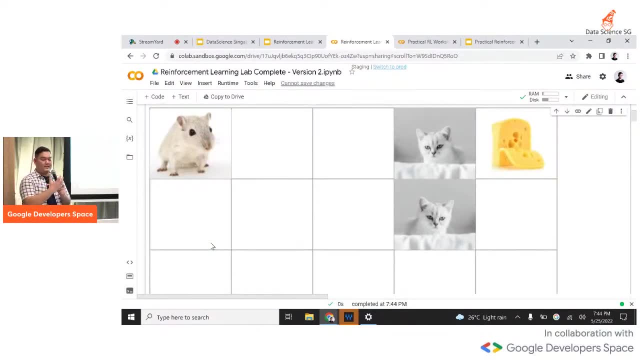 it will alert me, So don't have to worry about that one. So the first thing: first we need to define an environment and the states Right Before we start training the agent. we have to build the environment. We have to define the states. 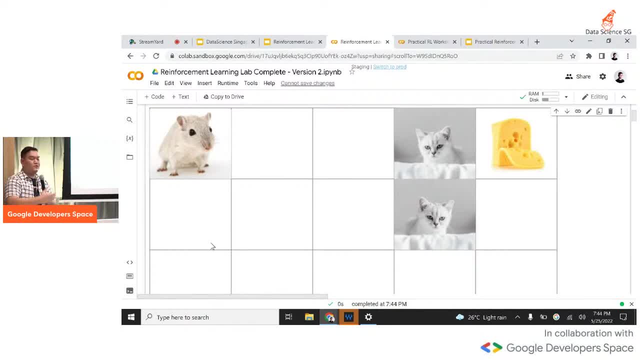 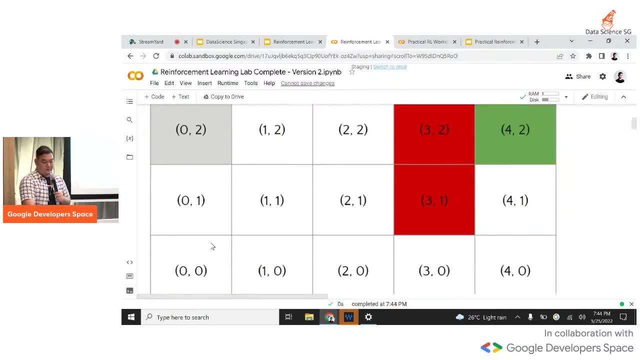 and we have to define all the rewards and the action so that agent can use the action in the environment to get rewards and learn. So that's what we will do, Right? So, if you are familiar with grid systems, so from this, 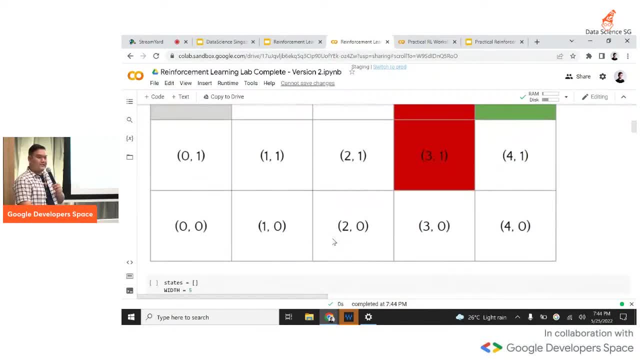 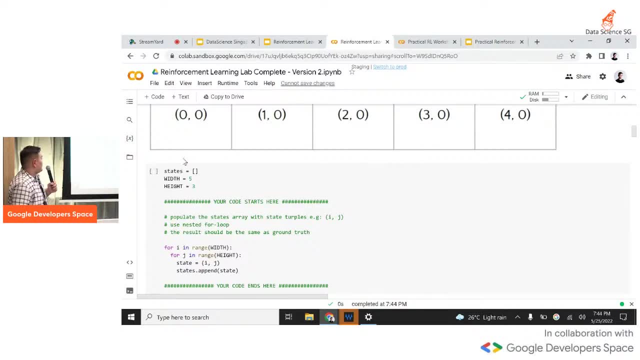 we convert into this, So just a coordinate like 0,, 0,, 1,, 0,, 1,, 2,, etc. So what I will do is I just do that right from my code is the states: 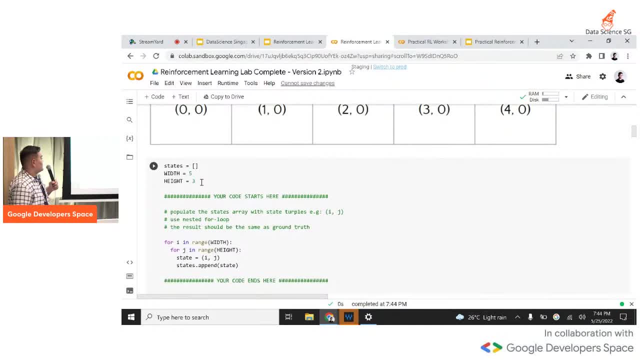 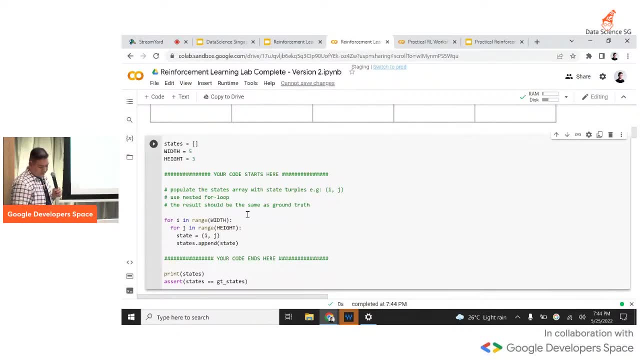 I define width as 5, then height is 3.. Pretty much, I create a tuple of those the states and append to the list, Right? So if I run this code, it should give me all the states, which is just a coordinate of the system. 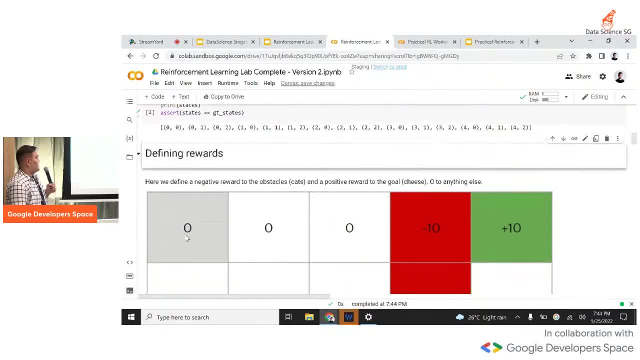 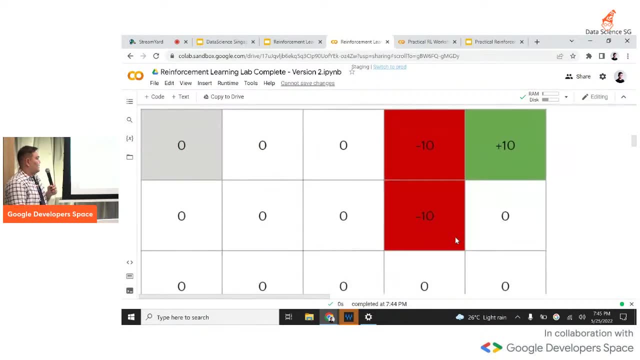 Right. And then we need to define the rewards. So I am defining cheese as plus 10 and the two cats as minus 10, to just make it easier. It can be arbitrary, It can be anything, It can be 1, 2.. 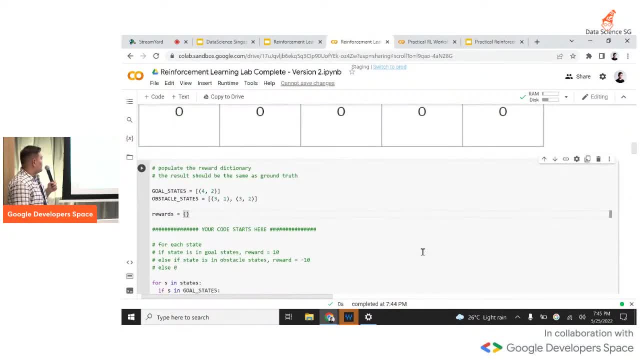 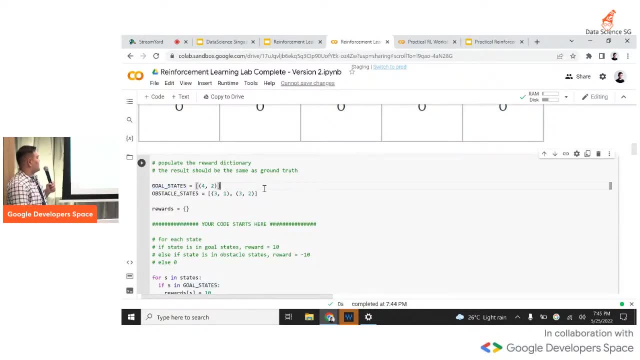 It is up to you to define it, And so this is the reward that I will do. I define my goal state, which is 4, 2.. I define my obstacle state, which is 3, 1 and 3, 2.. 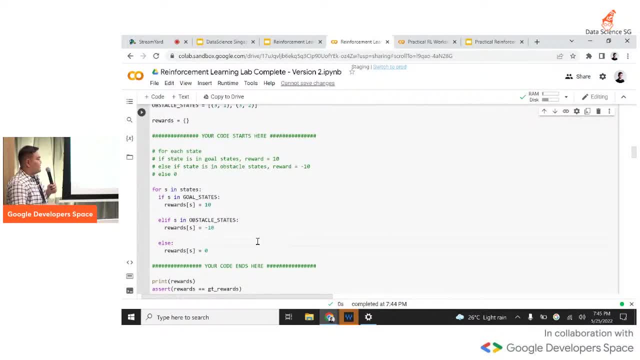 These are two cats, Then I just loop through and then assign Right. If this is equal to goal state, I give them 10.. If not equal to goal state, if equal to the obstacle states, I give them minus 10.. 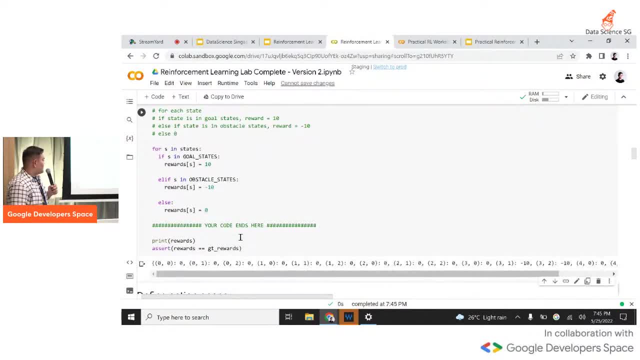 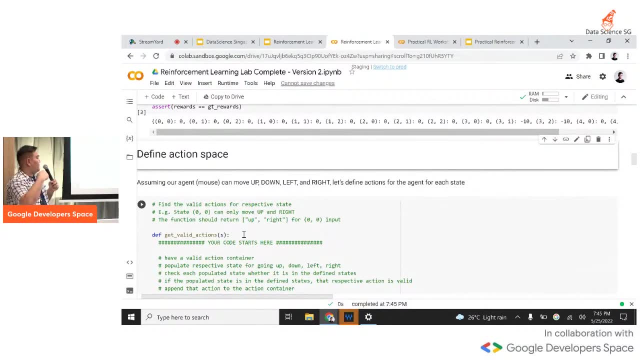 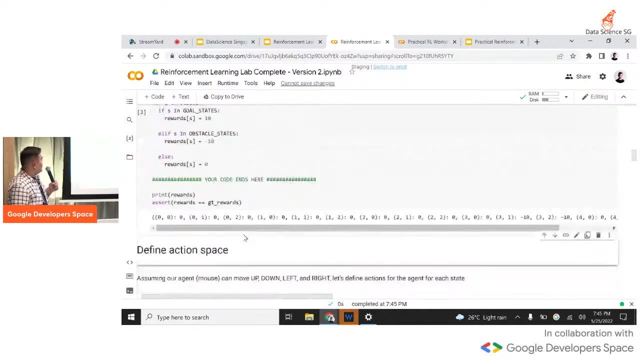 The rest is pretty much 0. Right, So I define that. So now we have done environment states and also we need to do actions Right. So for actions is just upright Right. But if you notice, if our agents is here, 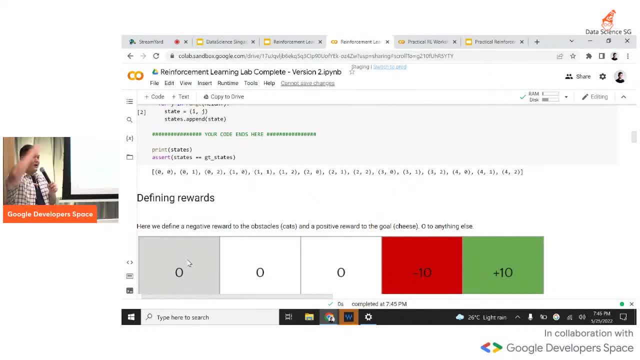 only goal can go left and down, cannot go up Right, Because it is the wall Right And if we do not define it well, it might get stuck, keep going up And never come down. But not that it is really necessary. 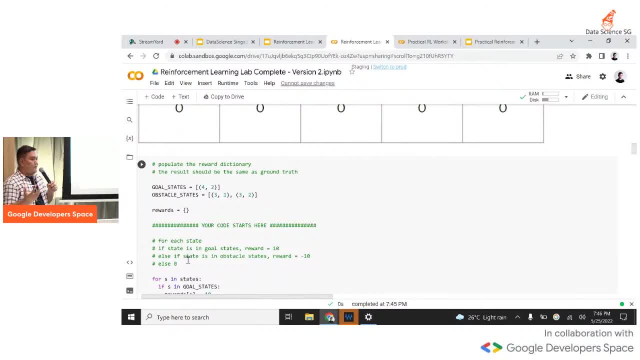 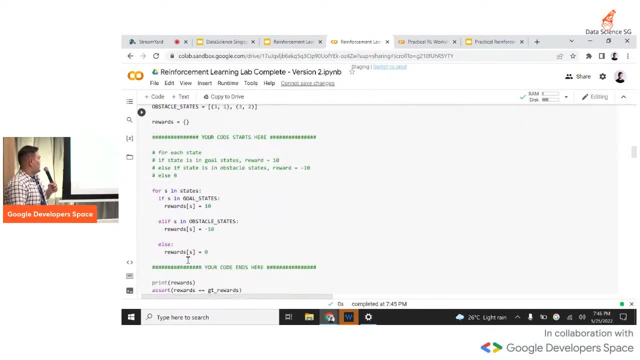 but to speed up the process. in real life you probably do not know where the wall and surroundings are, So you probably just keep trying until you get it right. But in this case I know where exactly it is, So I just define all the possible actions. 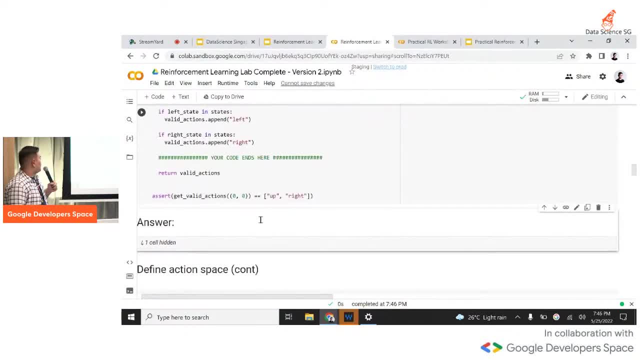 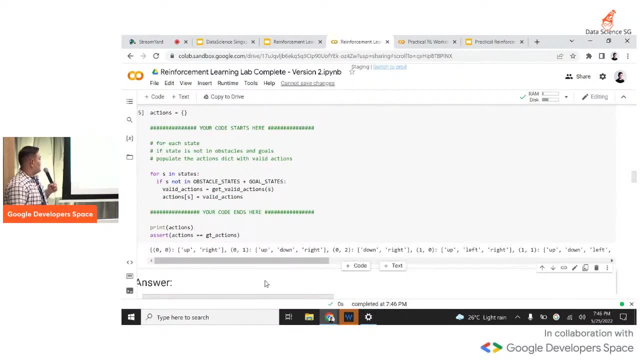 that agent can take Right. So now I have all the actions, All the environment rewards actions, Right. Then I pair them up. So policy is still pairing them up. Pairing them up is basically just to define at which states what are the valid actions. 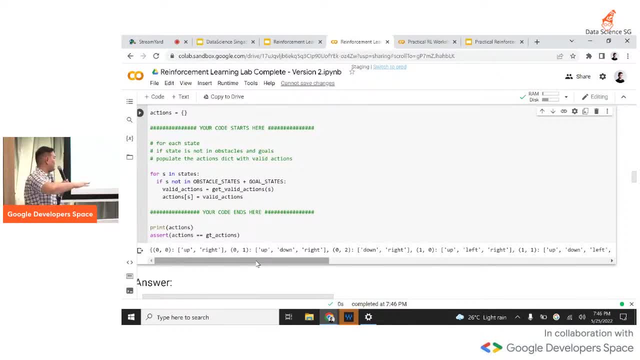 that you can take Right. So 0,, 0, you can only take up down, or upright 0, 1 is up down, right, etc. So I am just limiting it so that it is trained faster, in a way. 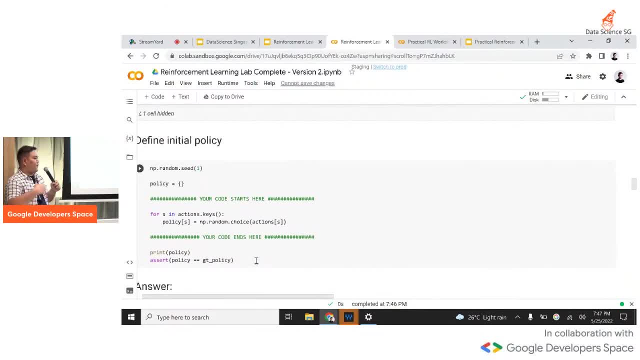 So before we send the agent to the environment, the agent has to know something, Right? I need to know what to do first before I can learn, Right? So we have to define the initial policy, or like action plan in a sense. 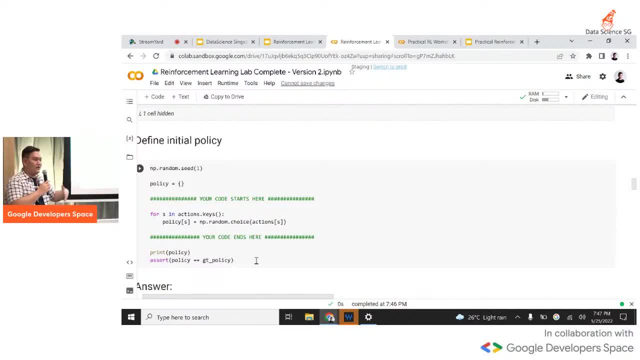 So you have to give them some action plan so that they will execute the action plan. learn from it. Maybe there are some mistakes. I bump into the cat and I die. So the next iteration, I learn from that. I do not go to that. 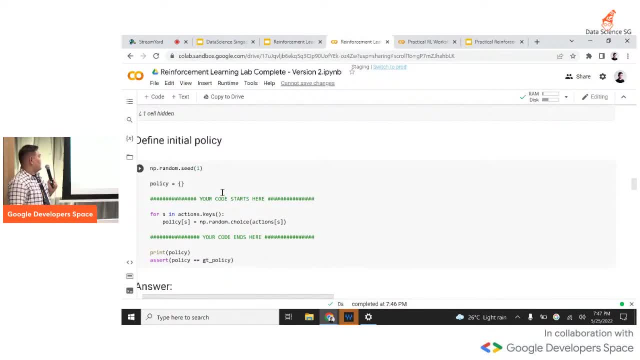 I do not take any more Something like that. So the first initial one: we are just using random Right, So we do not really know what works and what does not, So we just random twice from all the actions possible. 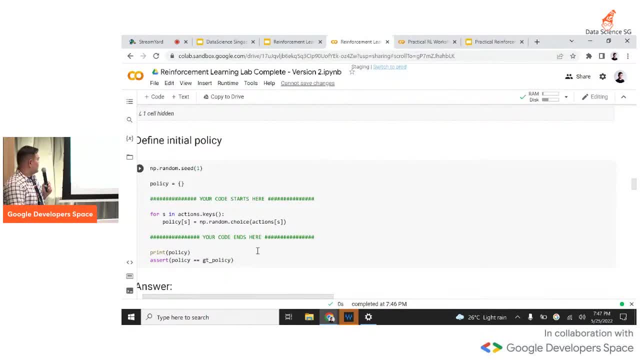 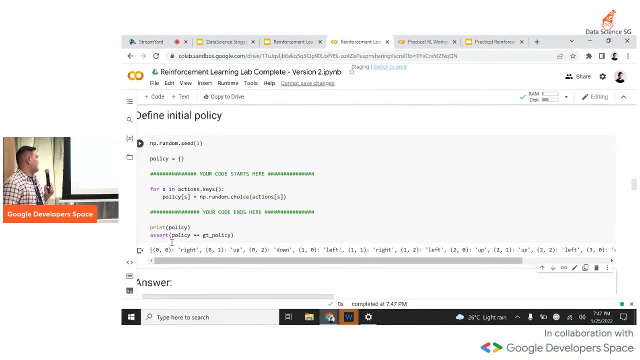 for all the states. So it looks like this Right. So like if 0, 0, go right, 0, 1, you go up down. This is not optimal at all. It is just randomized. 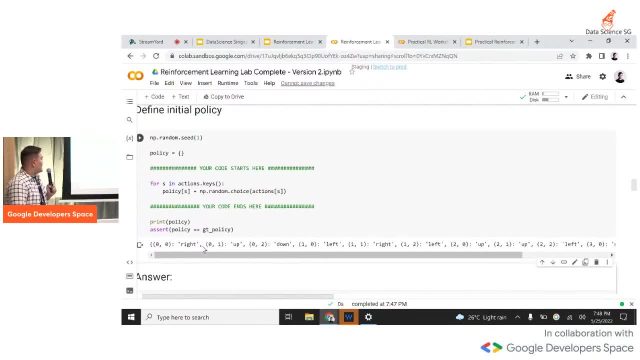 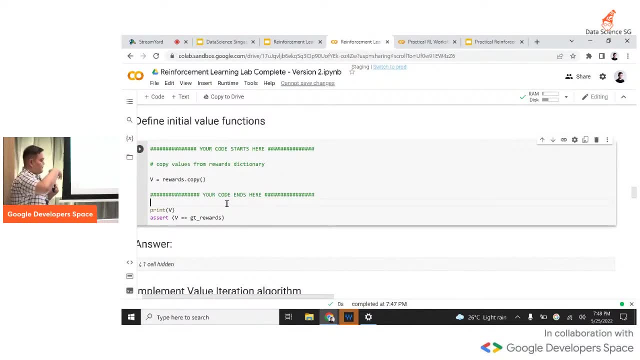 So once it is randomized, we sort of have to define our value function in this way. So value functions are pretty much from one state to the goal state. If I take this path, what is my expected return from it? So 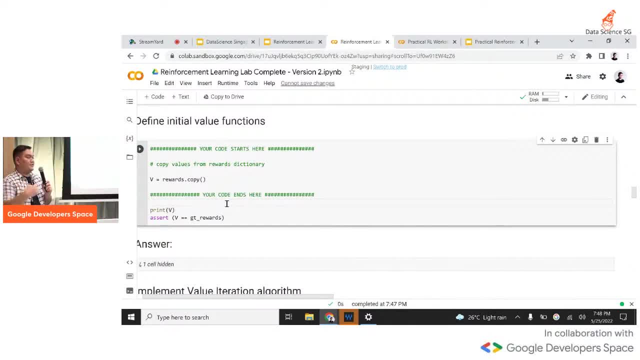 I could be taking straight, I could be taking curve, I could be taking, like you know, zigzag. What is my expected return? So for now, I just copy the reward states, because we do not know any rewards yet. 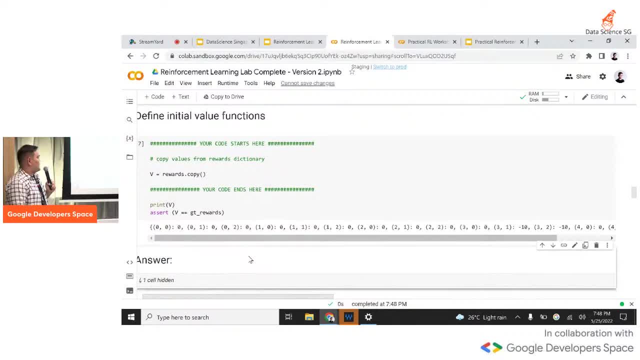 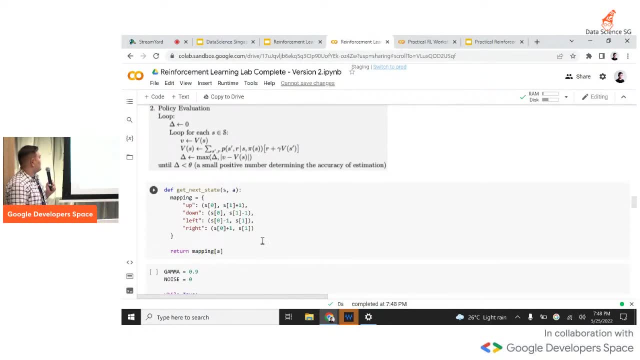 But for this part I basically implement it. So for now I just copy the reward states because we do not know any rewards yet. But for this part I just implement it into the value iteration functions And I am choosing. 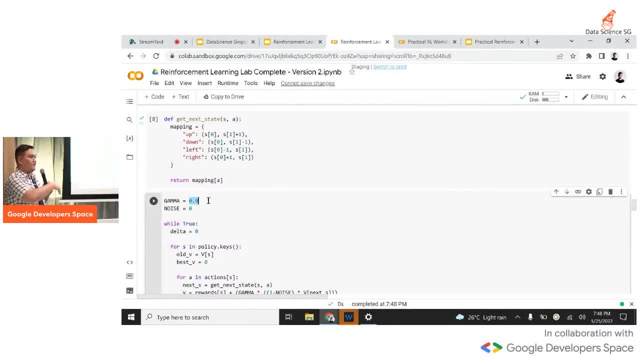 gamma as 0.9.. If you remember, gamma is the discount factor And I am not putting any noise, But sometimes you probably need some noise to counter-react for your environment, For example, if you are programming a robot like 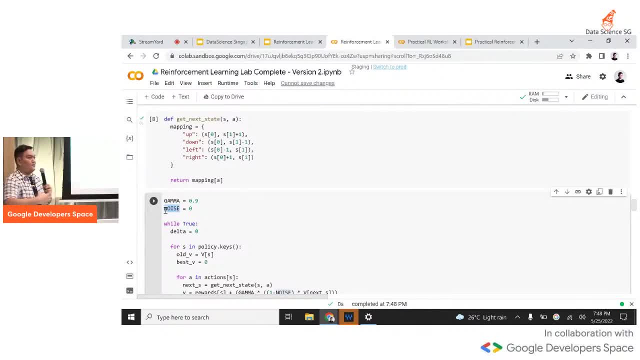 a cleaner robot, your floor might be slippery So you need to cater for that noise in your program. the motor function. So sometimes it might have some constraint in your wheel or something like that. Then you probably need to cater for that noise in building or training that agent. 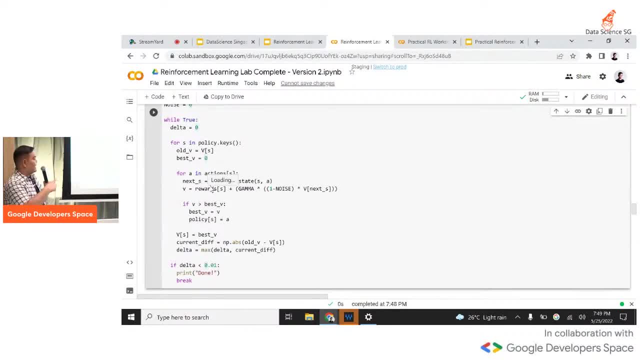 So this is actually the formula that I just shown you from the slide, And then pretty much what I'm doing now is I will just keep iterating through all the policy key is a state, So every state. I will choose random actions and see if there is something that is better. So I took action like 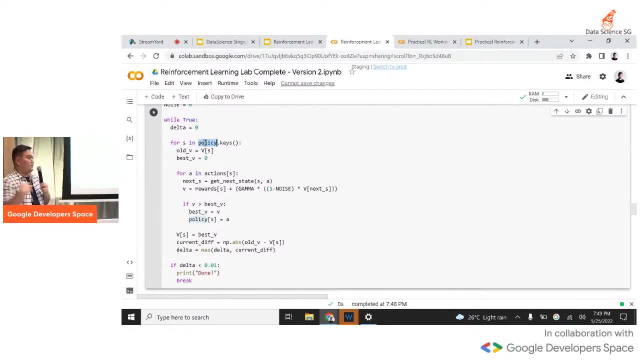 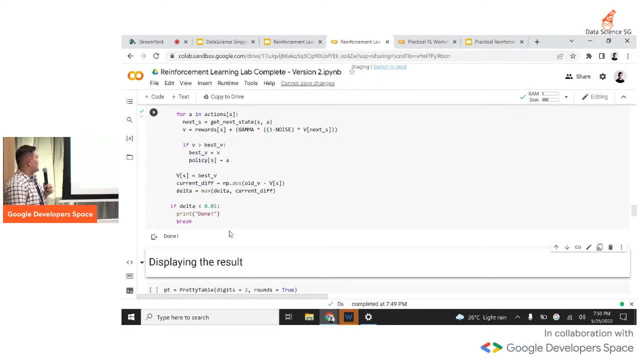 take left. I will compare the next time with take right, see which one gave me better expected return. I will choose that. So I will keep doing that for all the states until they don't change anymore. So that's pretty much it. So, because this is quite open, so it's pretty much very fast. 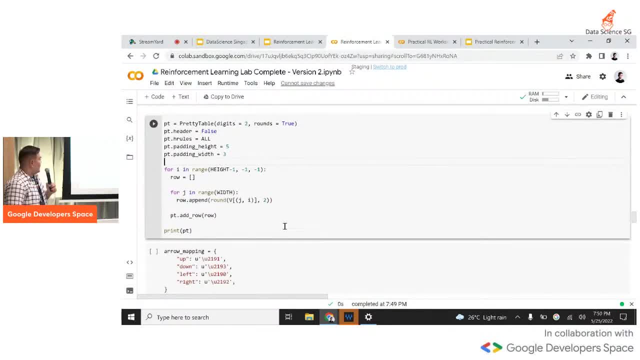 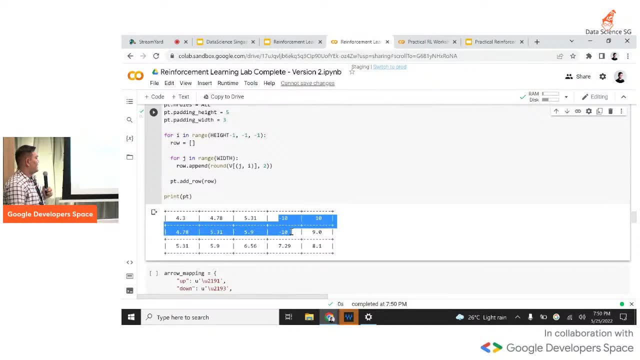 And after I have done, I could print out the value. So remember, we defined the value of cat as minus 10 and the cheese as 10.. But after this iteration of all the calculating the expected returns for each states, we sort of get this kind of value for the empty state which we have: zero. 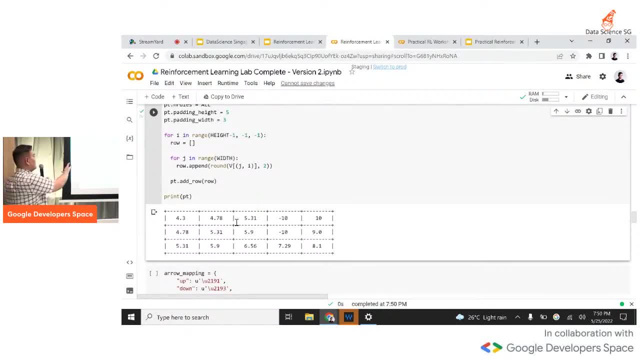 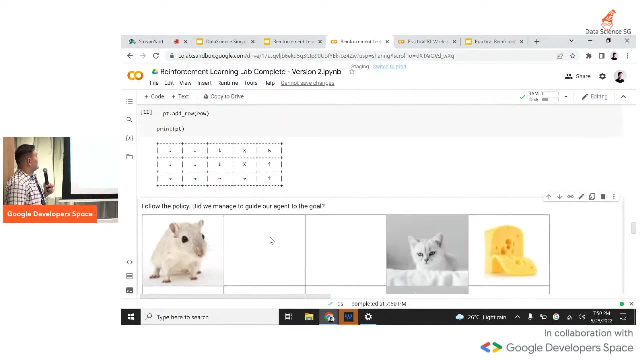 initially. So the agent will have learned this value. So we are going through again and again and again and again to update the best possible rewards. So after that we can come up with this kind of action plan. So the action plan for the agent at this stage is: if you are in this stage, you have to go down. If you 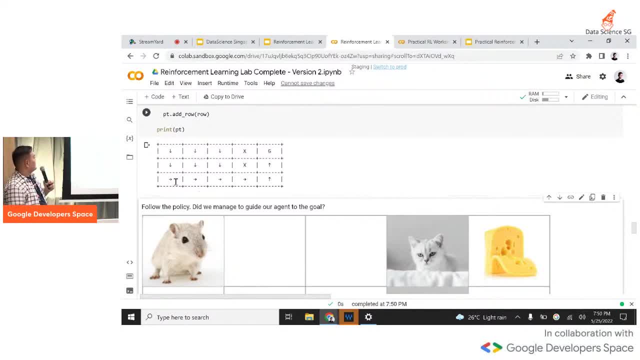 are in this state, you have to go down as well. If you are in this state, you should go left. If you are in this state, you should go left. If you are in this state, you should go up. So by guiding, by going through this action plan, the agent can arrive to the cheese. 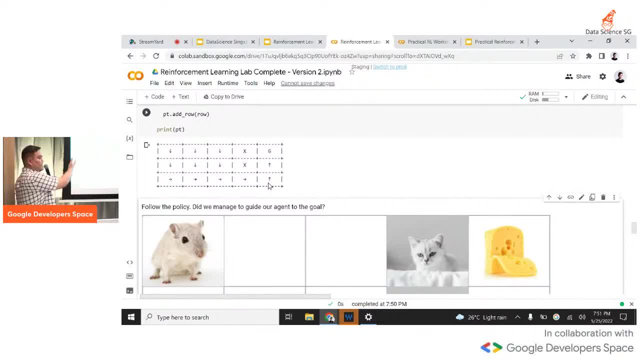 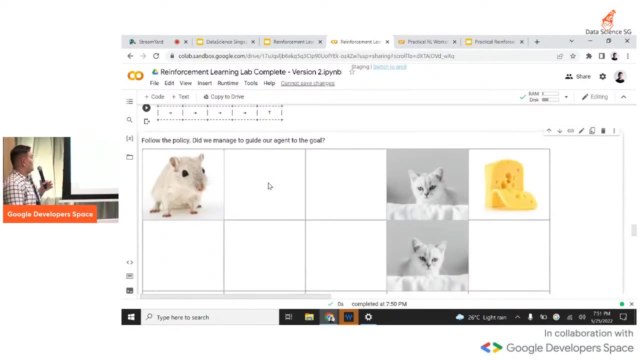 successfully. So our goal is to come up with this. So once you get this, you can just use this as a map to travel around. So our goal is to find this And the agent will have remembered this in their brain so that they know where to go. Yep, So if you are up to the challenge, 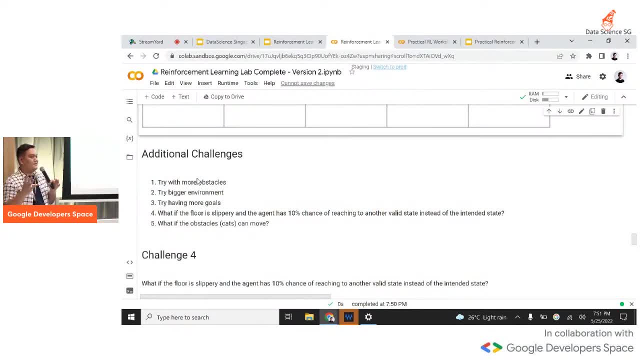 you could try More obstacles and try to block the cheese and see whether the agent can arrive at the cheese without having to, you know, go through the cats. You could try with bigger environment. Currently it's just five by three, But you could try 1,000 and 2,000 or whichever one. 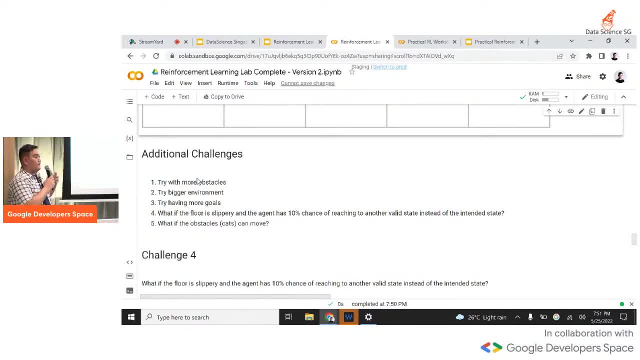 you want to try. You can also try with having more goals, right, So I talk about the time being the important factor. What if the goal is too far away, right, And you are mouse so you can't be going around? 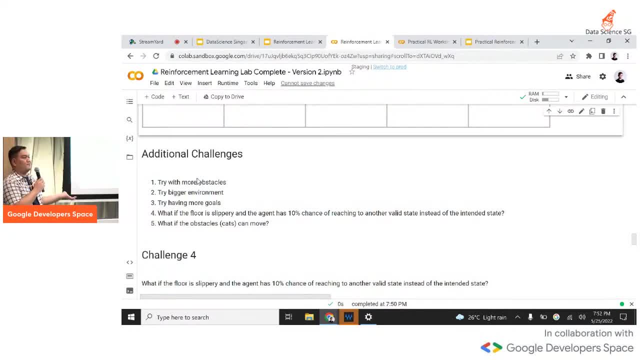 You can't be around infinitely trying to find the cheese So you probably have to find something else. So if you are having like time constraint, you could add that right. You can add immediate goals to that, And I talk about the noise, the floor being slippery If the agent has. 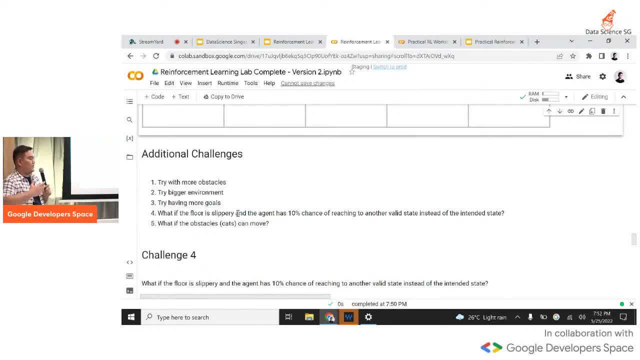 10% chance of reaching to the United States right. So if you go left, it's only 90% of the agent reaching to the left, but it might slip out and reach the other states, that which you didn't intend to do. So how do you do that? 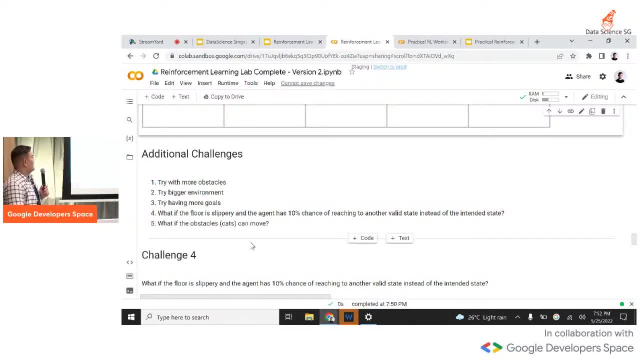 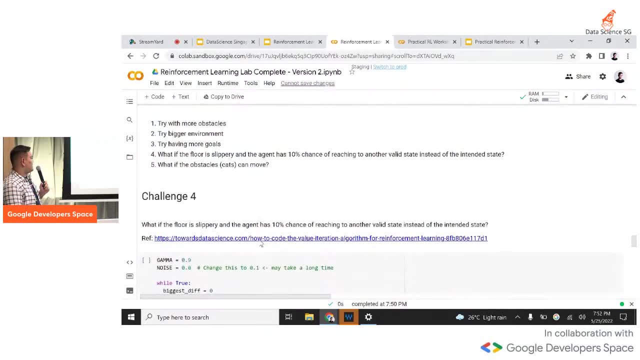 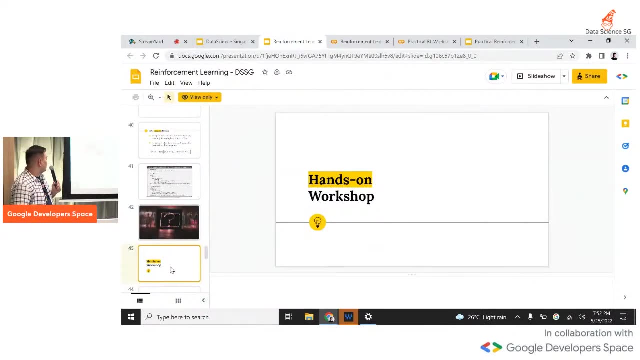 How do you frame that into our problems? And also, like, if the cats can move, So how do we do that right? So this is something that you can try it out. if you are interested, I will send this link or you can access the link from here. Let me just quickly go through. 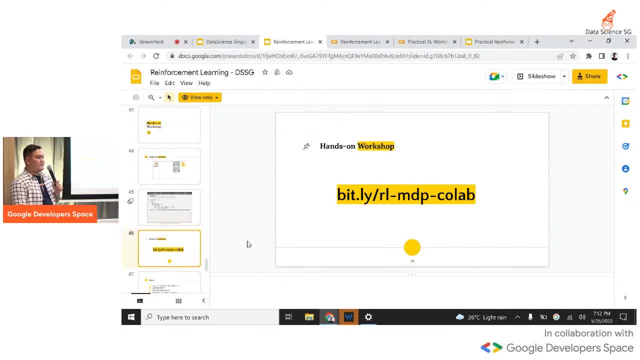 So maybe take a screenshot of this if you are interested. This RNMDB collapse And you can find that: Okay, Okay, All right, Okay, so that's pretty much it. We have learned all this: Reinforcement, learning, MDB, reward, action, return, episode, date, continuous policy value, function. 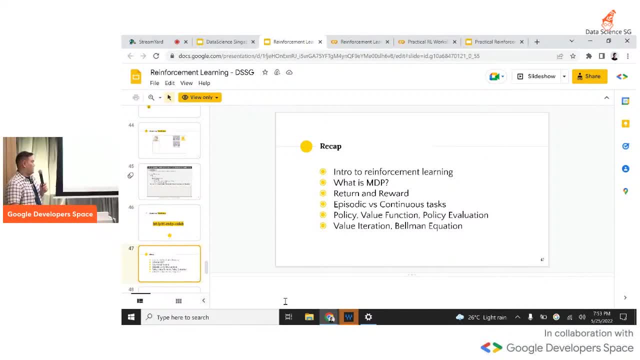 policy evaluation, Value iteration and Bellman equation. So pretty much this is like two weeks in university lecture, But you have learned in 30 seconds, 30 minutes, I think, Yeah, So that's pretty much it, And like where we are now we are. 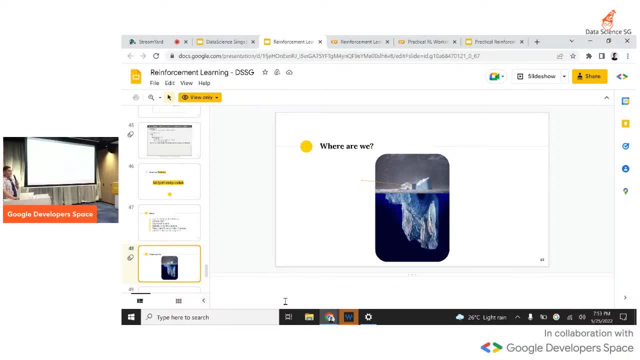 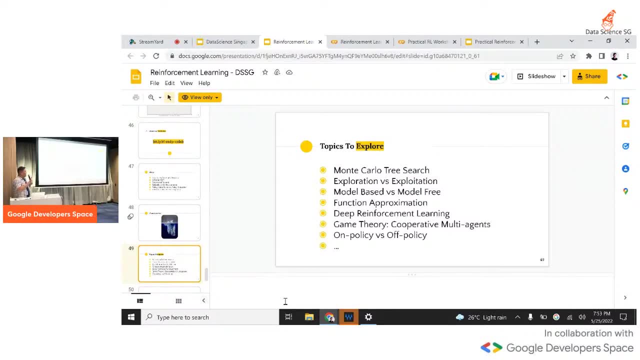 We're just the small tips of the iceberg in reinforcement learning, which we will be exposing in the future or later session, And if you are interested to learn more, there's a lot of things that you can explore right: Multicolored tree search, model-based, model-free function approximation, game theory on-policy. 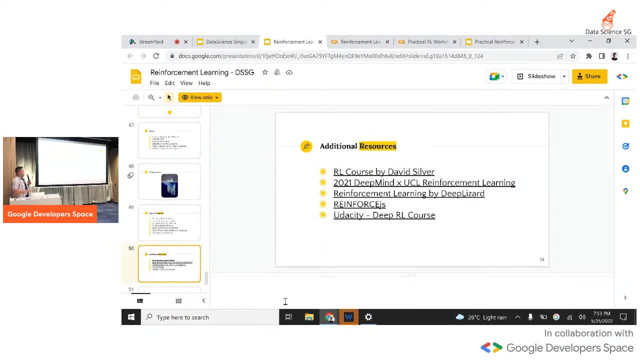 off-policy, all these things, And these are the resources. I think the organizing team will share this slide with you guys, So don't worry so much about this. And yeah, thanks so much. And if you can reach out, you can reach out. 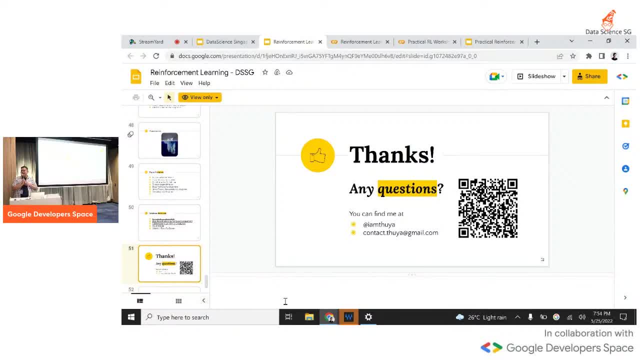 I think the questions. there should be a pigeonhole somewhere. The pigeonhole links in the question. We will do Q&A later together. Yeah, OK, Yeah, Thanks, so much for your time And I hope it's useful for you. 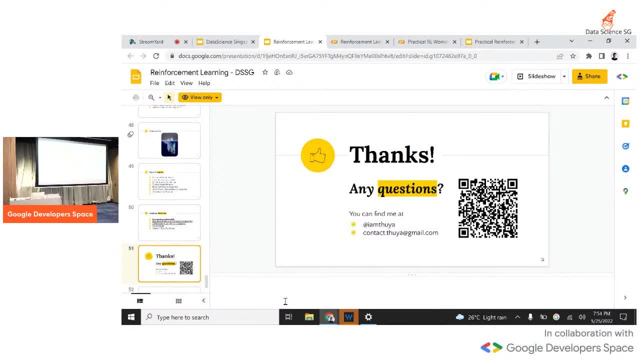 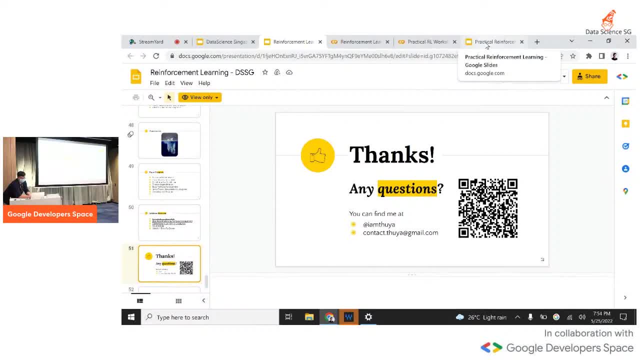 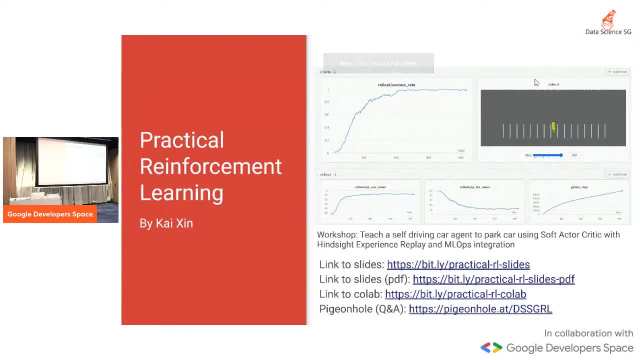 Thank you everyone for joining us today. So I'm Kai-Singh, So we have been running Data Science SG for eight years, So it's very nice that we can see everyone back, both old and new faces. The last two years has been quite a tough time, right for everybody. 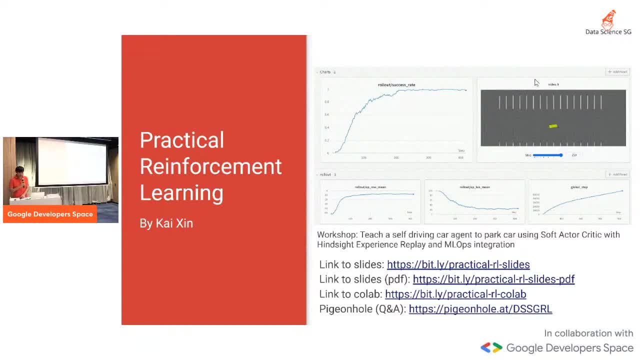 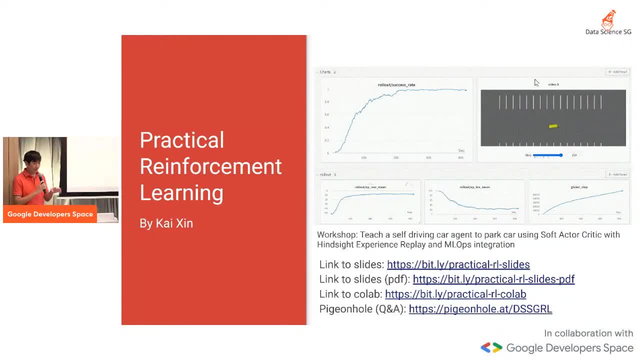 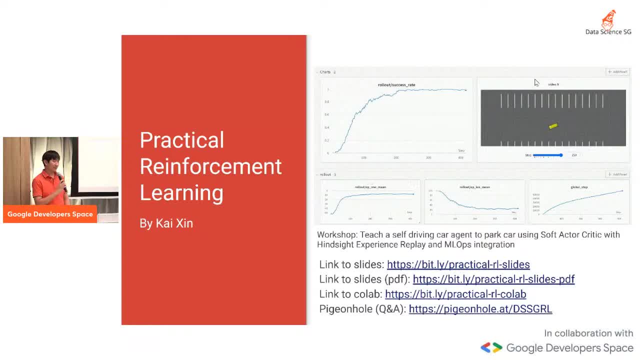 how do we actually use it in the industry, to what extent that we can Reason being practical reinforcement, learning itself is about five, 10 years away. That's what I tell my boss and everyone that ask me as well to be really usable by. 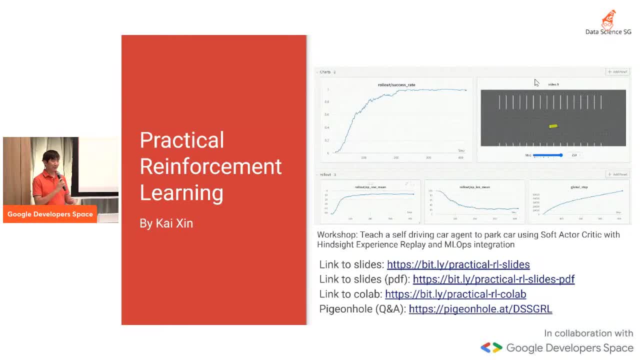 the masses. Think about XGBoost, Venom Forest, all these things that you're familiar with. or even now there's language models, models or this right. This is probably at the maturity. If you think of S-curve, it's probably. 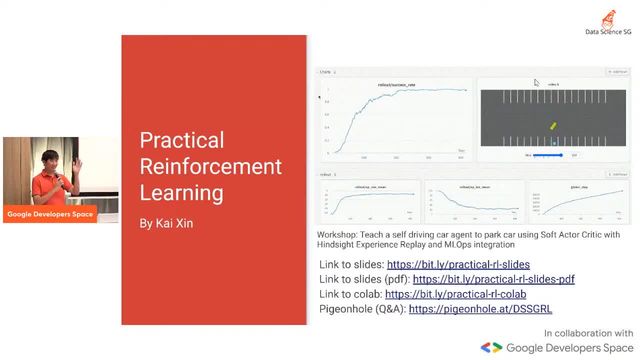 at the maturity stage. Reinforcement learning is not near the S-curve yet. It's really at the bottom where we're exploring a lot. So some of the questions, you can see some of the links there and then also pigeonhole, you can post question. So some of the practical things is what it can. 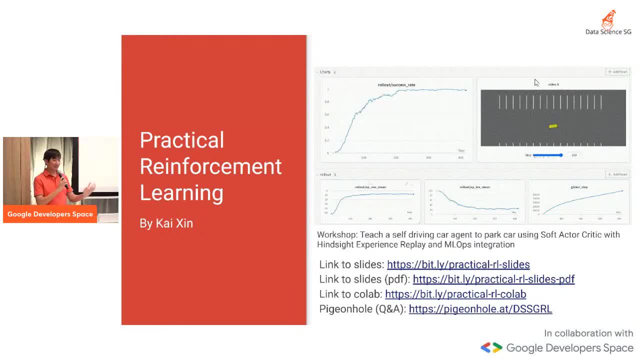 be used for At the back of my deck. we'll have some examples, mostly in robotics. So what we see here, mostly in factories, robotics processes, And the reason we will go through, as you go through with us, this example here, you start to realize that for things that you can control in 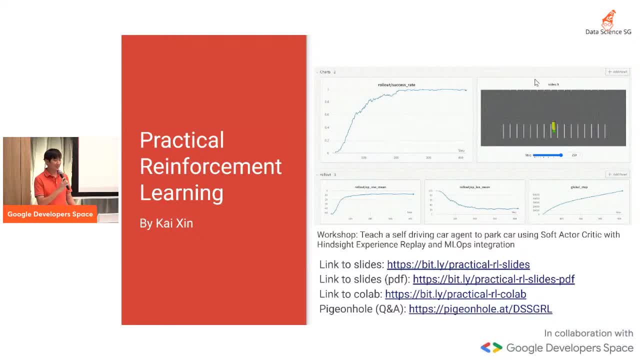 an environment like a factory floor, a very defined process possible to do some reinforcement learning. you need to create an environment for you to create this state action reward, like what Tuya mentioned, If you want to do something like an investment, which a lot of 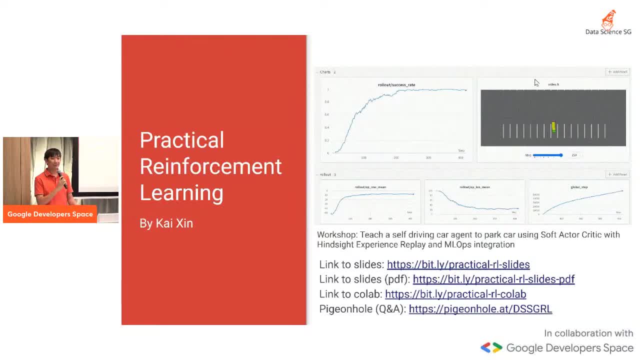 like I work in finance right. So a lot of the boss are like: can you create a reinforcement learning portfolio? I can. I will not invest in it. I can give it to you. I will never want to look at it again. 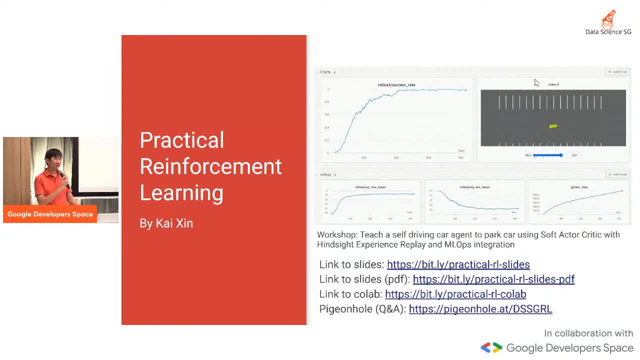 because you'll lose money? Because there are a few factors. Number one is you need the entire team of reinforcement learning- PhD scientists, engineers- to maintain it. And number two is creating this environment of state action reward, like you see here, driving car games right. 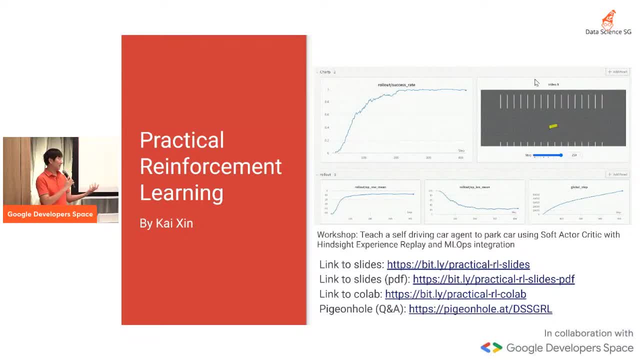 It's very hard. So there are two branches: There's one team that focus on building the environment and there's one team in building the environment. You need both. So this beautiful environment. we're going to talk about parking a car. It. 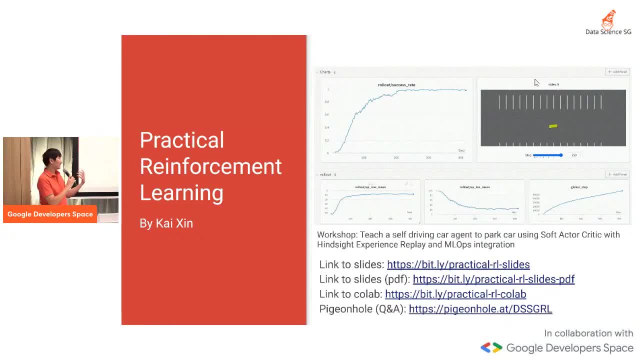 needs to be created first and it needs to be able to factor in the entire state action, reward the training thing and be able to kind of grow together the algorithm. Imagine doing this kind of thing for investment. You need to build an entire simulator first before. 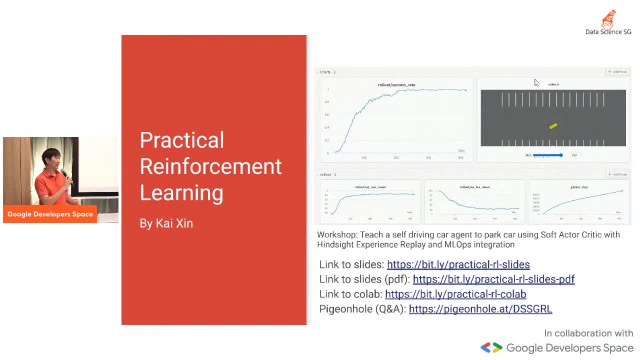 you can have a nice reinforcement learning agent, That simulator. if you can build one, then you don't need a reinforcement learning agent. You can simulate a market for some reason. If you've got an algorithm that you have to build a simulator in that scale, then you don't. 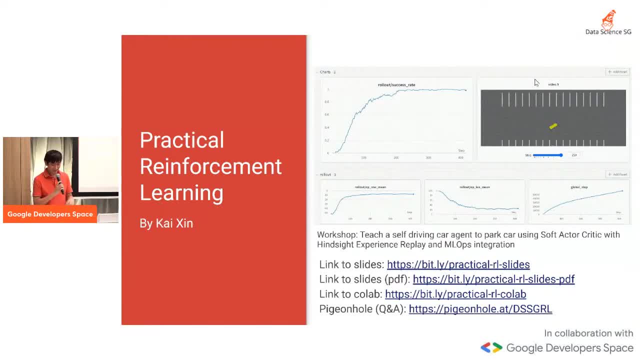 need reinforcement learning. You just own the market, So there's a lot of things to it. So there's also a question from Pigeonhole about poisoning. So the practical aspect of reinforcement learning agent we hear so far is very dependent on the reward function And poisoning means that. 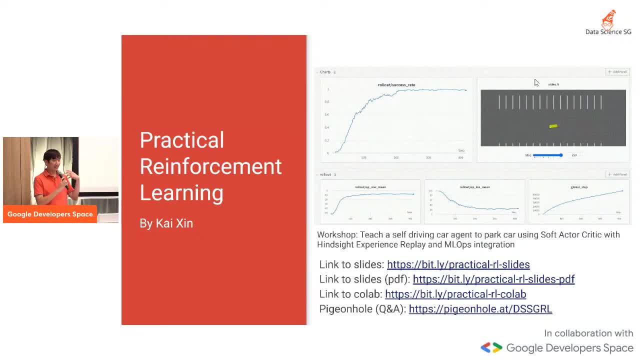 you purposefully, adversarially, add a fake reward to the entire reward function, thus poisoning the outcome, The defence of that. we will talk about some of the things clipping and some of the overseer things. actor credibility might come into play to solve it. So, as we go along, we'll cover. 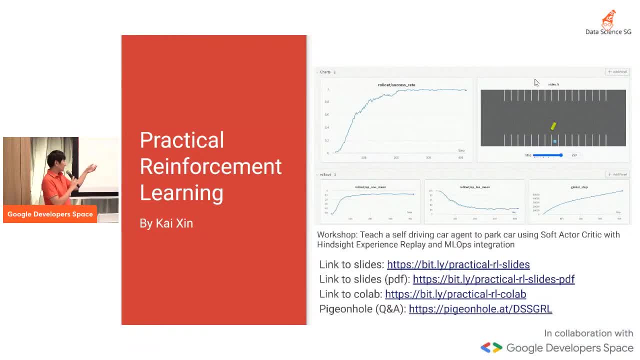 some of these practical aspects of it as well. So this is meant as a one and a half hour workshop. I will speed run it a lot of it, But the idea is we'll talk about soft-actor critic with hindsight experience. we play in ML Ops. 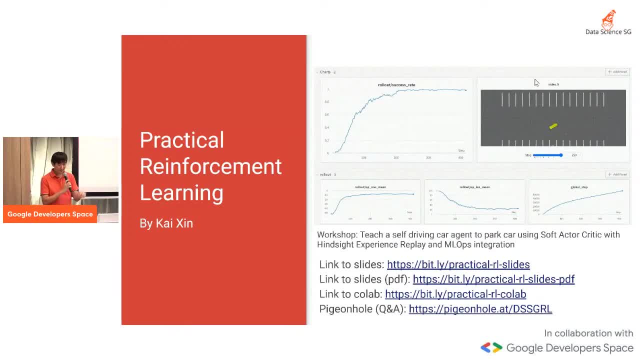 So actor critic. So this is a parking example. So I want to park a car. So if I want to build, If I want to build, park a car model, if I tell you, go and build one using supervised learning method, big data technology. one way is to go gather a lot of data about parking. 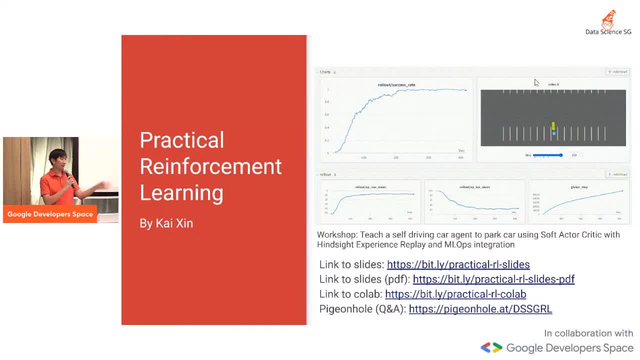 You go to Europe and take a whole bunch of videos about how to park car in Europe. You take a whole bunch of way to park car in Singapore, all over the world because parking car under different conditions. you take three months to gather all the data you can about. 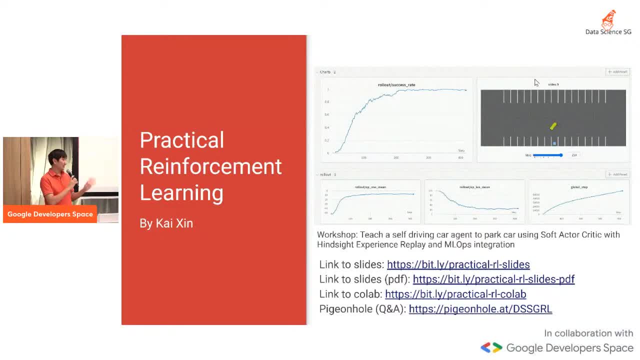 parking car because you want to build a giant supervised learning model using big data. That might work, but that's not how anyone learns how to drive. Anyone learns how to drive by number one, driving Number two. you go to attend a school or a trainer with you, and then the uncle will. 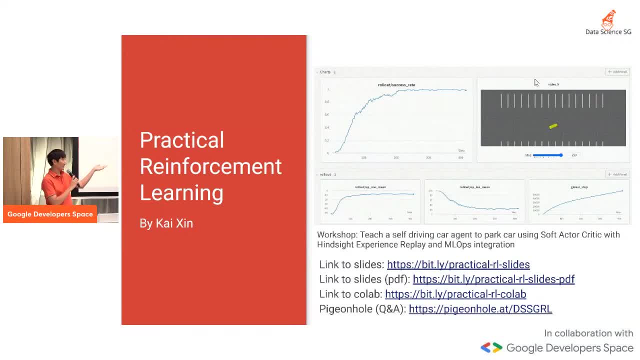 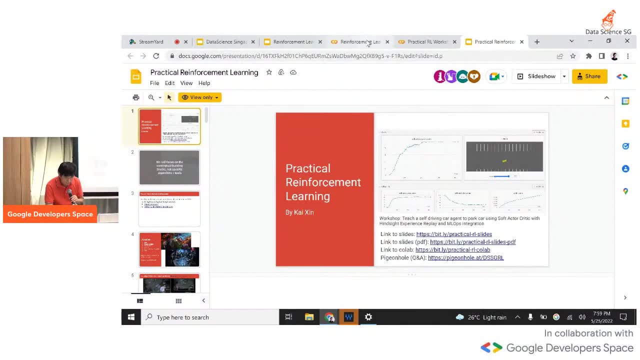 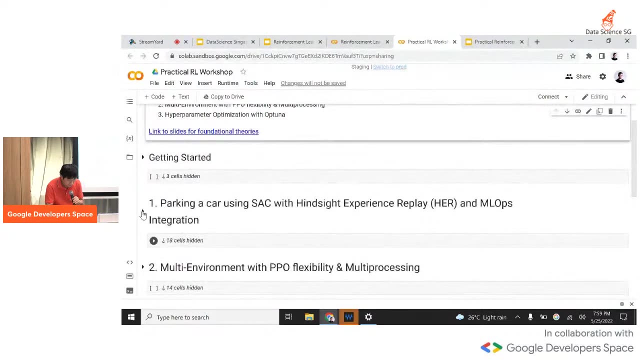 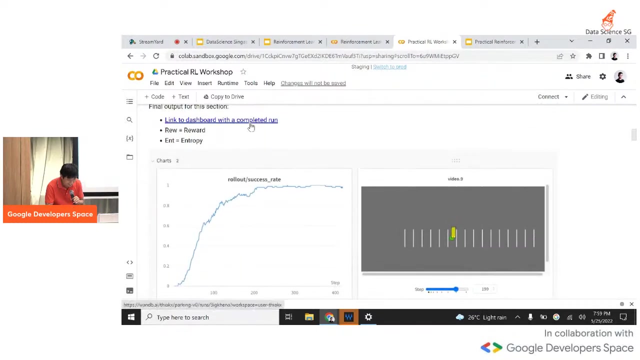 scream at you like what are you doing? And you'll park the car. So let me show you some examples of this particular agent in work. Okay, Parking car. So we'll go into the need to go find a dashboard. you may say: 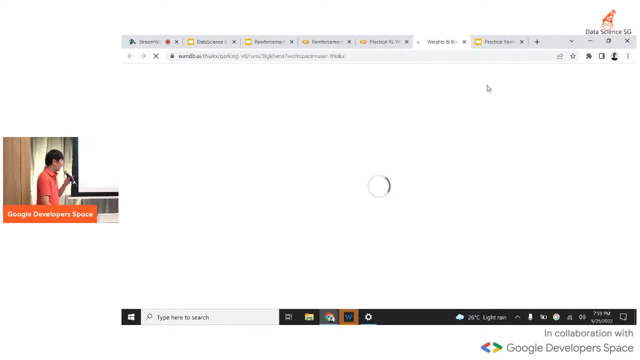 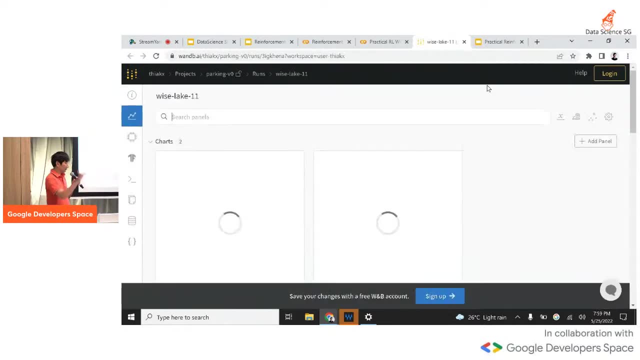 This is too sensitive. So we're going to do a dashboard and we'll go through this parking example. So this is a simulator for parking and the whole goal is, of course, to park into the box. You have some physics in it and stuff. 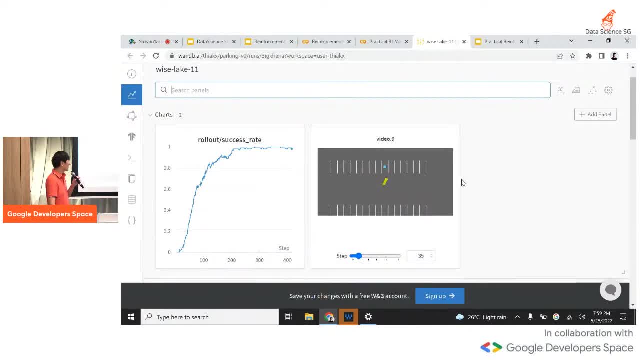 But it's not like. It's not like a perfect simulator, because you see it's an empty car park, view all the other cars and stuff. But let's go through and see how the agent learns and we'll talk about how the various 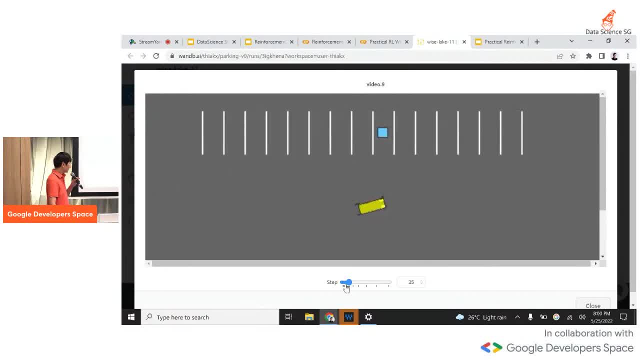 pieces come together before we go on to the theory of it. So step zero, Each The size will be weird. So we define steps. Each episode has multiple steps, So some keywords we will learn. also, Episode is basically a training. So this is one episode, one complete episode. 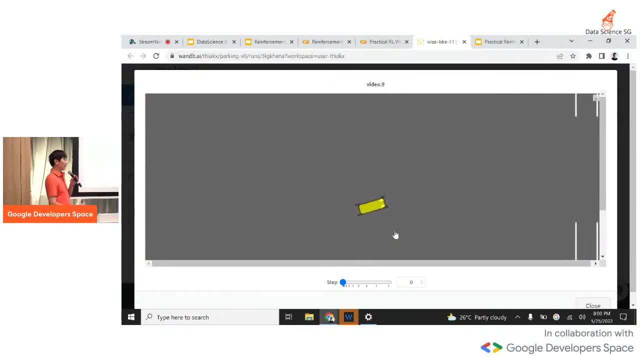 The car drive parking. The car drive all the way. This is Initially. the car has no idea what they're doing. So imagine you're driving like that. Your instructor will be like: what on earth are you doing? 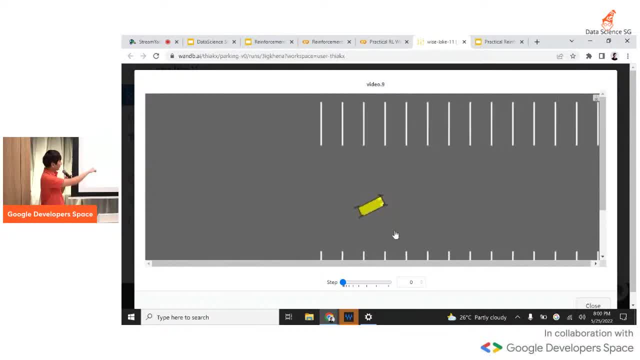 Where is your eyeball? You look at the thing You want to go to the blue box. Why are you going all the way off-screen? So, actor critic, I'm the driver, The agent is the driver. There's a critic layer. 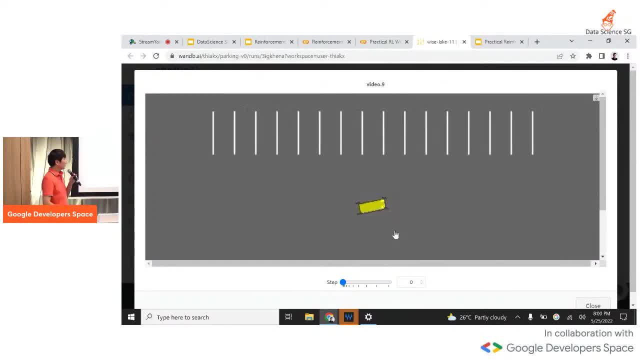 A critic: the instructor scolding you. What are you doing here? Look at the eyeball on the blue log. Go towards that thing there. So actor critic is two layers of deep learning network working together. So the first layer: the instructor scolding you. 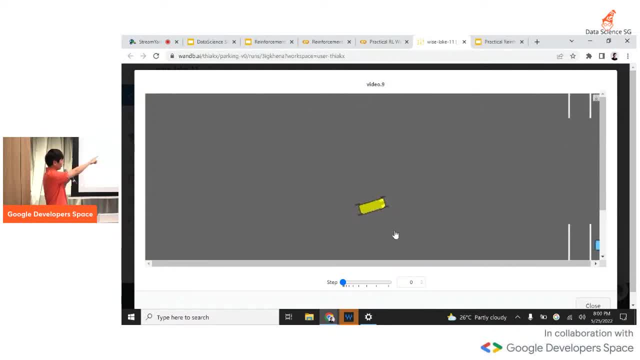 The second layer, the instructor scolding you. The third layer, the instructor scolding you And the critic will validate what the actor's score is. So you see, as we go further through the episodes, it's getting a bit better. 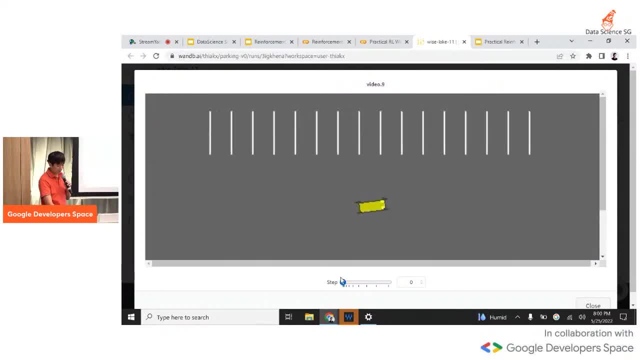 I mean, it's still going off-screen, but it's pretty stupid, still Nowhere near where we want it to go. But let's slowly see as you step through. Okay, No, Okay, Okay, Okay, Okay Okay. 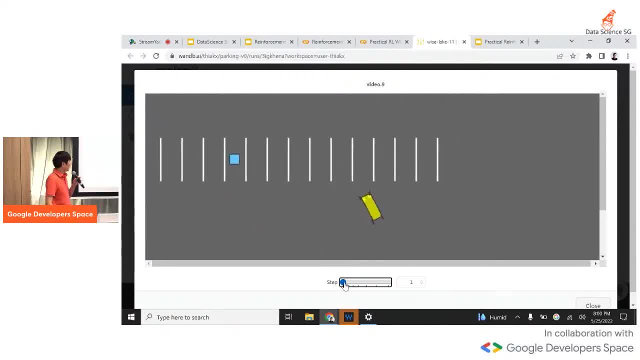 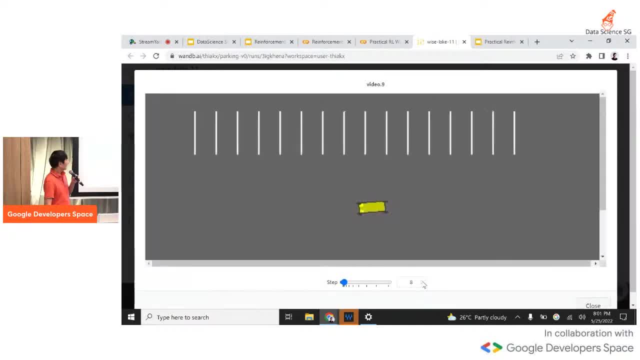 At least it's trying to stay within a carpet area. Let's see this one. This one is still driving like a wild man. one bad example: Okay, Let's go, Okay, Okay, You're getting there, Getting there. So it's getting some sort of reverse. 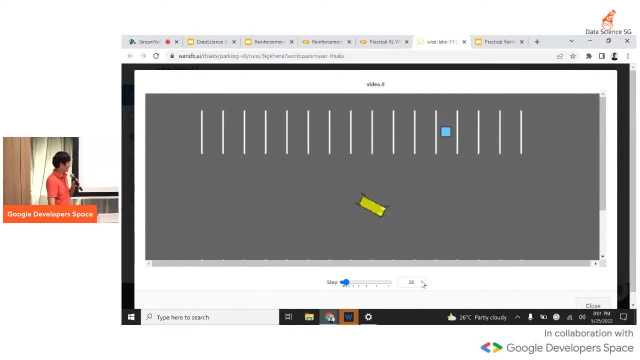 He's trying to reverse so badly. So he went out of the screen and he's trying to reverse so badly. That's something we don't want, but it's timing out because it's taking too long. So what we see. so for the first time, it succeeded. 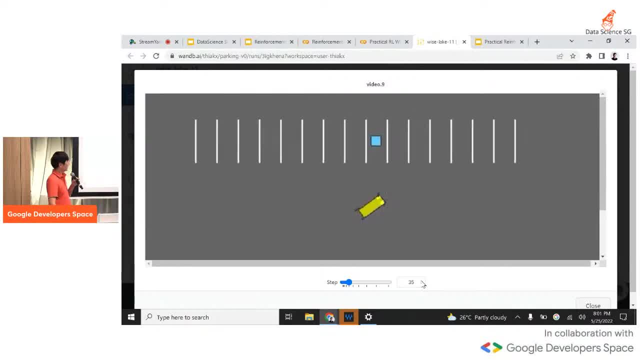 First time it succeeded, it managed to reverse in, So it's learning from its mistake. The actor-critic is playing along with each other, So there are two layers talking to each other And as we simulate this process, it gets somewhat better and better. 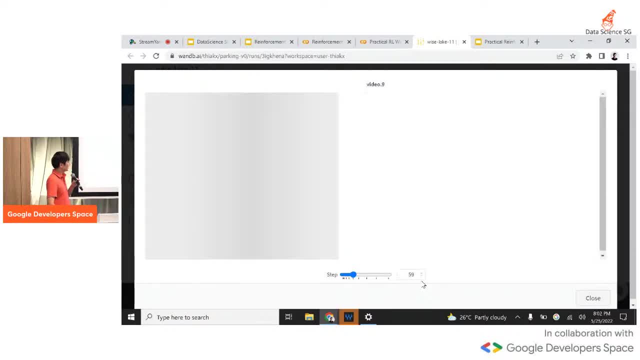 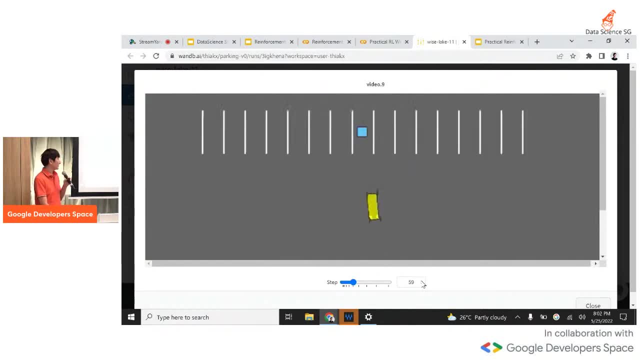 That's what I'd like to share, Basically based on the score and policy. the policy is getting better and better And you see that the car, now it learns speed because the faster it arrives, the better score we give it, Not really fewer. 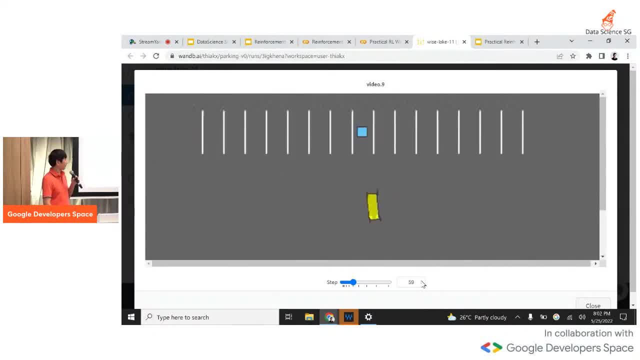 but the speed is one of the factors for good reward, So it's driving very fast to get to that point. And also take note that the blue box and the starting location of the car is always random, So it's not learning one way to drive. 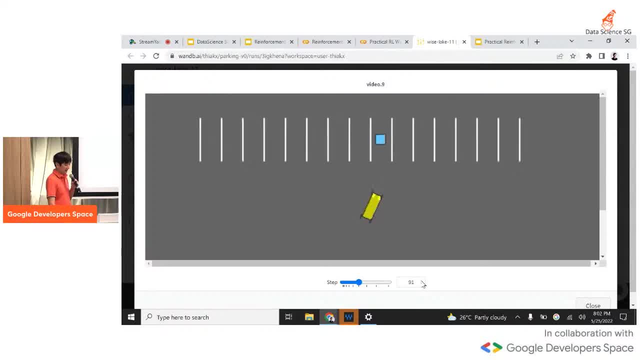 It's learning a policy to react. So that's the difference between that and a normal supervised learning agent. So now you see it's kind of doing quite well, quite fast as well, And it's able to do a variety of actions and angles. 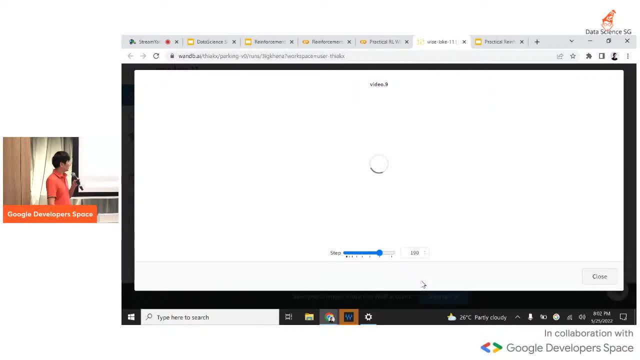 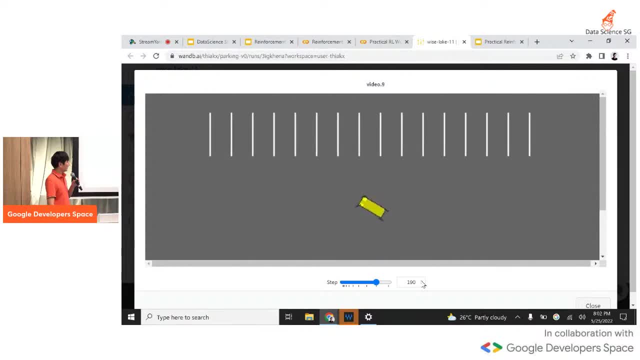 So that's quite important. So as it grows more and more mature, you start seeing that it always hits the mark quickly. So that's one of the beauty of kind of this general AI kind of like each thing right Instead of giving a bunch of rules. 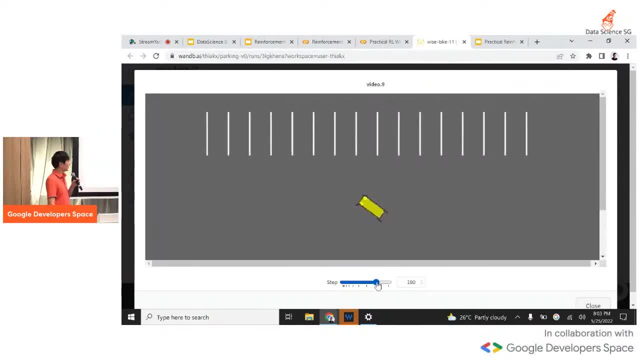 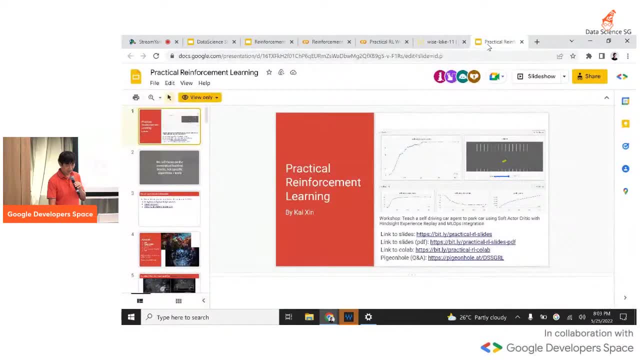 and having one model, it's reacting to the situation it's placed in, And that's very important And that's one of the key strength of reinforcement learning that cannot be easily replicated in, like supervised learning or other traditional methods. Okay, let's go. 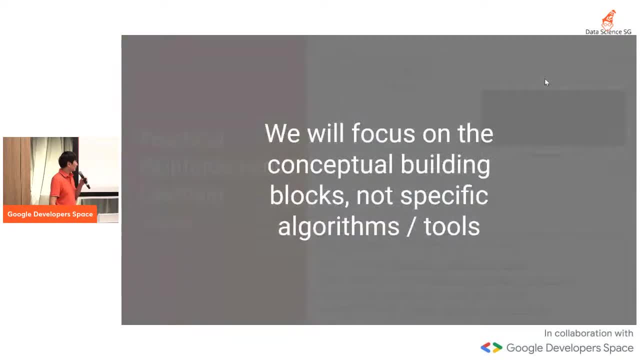 Okay, so today we'll cover a whole bunch of stuff, But so you can think to deep dive into that back later and all the code, everything is there for you to play with. But we'll focus on the conceptual building blocks. We won't be going into specific algorithms and tools. 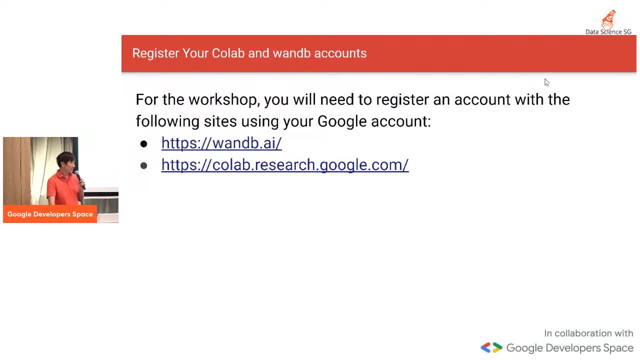 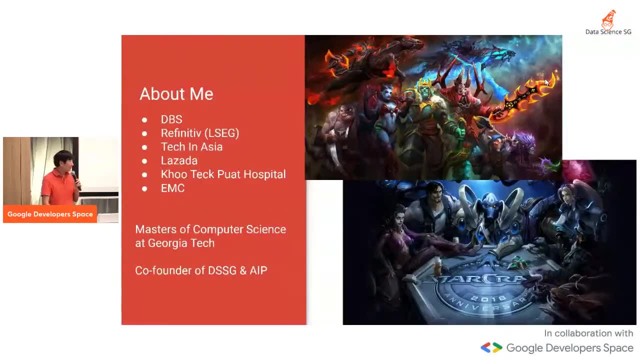 As in, we will touch the algorithms, of course, but we won't go deep dive into any specific algorithm. I want to give you the conceptual stuff And if you're interested, you can always find out more. So, about me, I managed to. 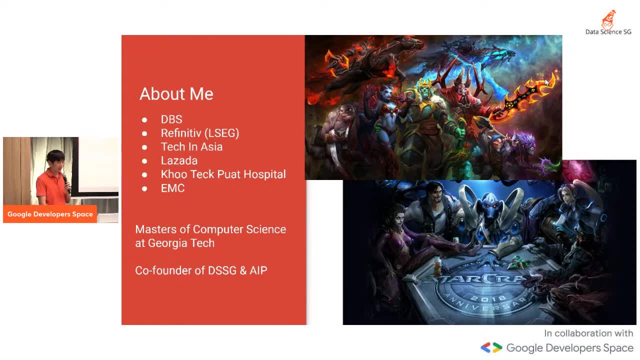 kind of my career span across a variety of different companies And I think one of the interesting thing was: okay, so I also with KUWA. we actually started AIP as well. So DSN CSG is kind of like free event for everybody. 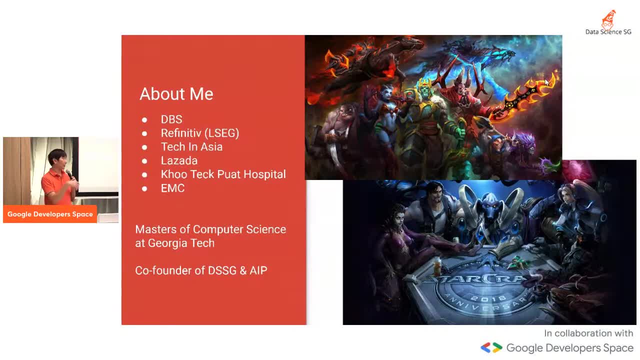 AI professional Singapore. we do certification, we do a bit of paid events, So it's more of a professional body of the DSN CSG. You can take a look at that. So what spanned me interested in reinforcement learning was the games. 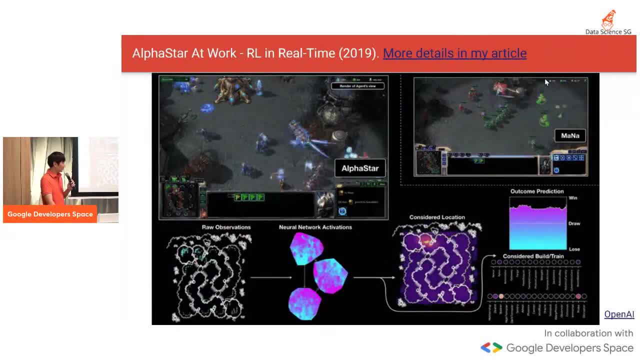 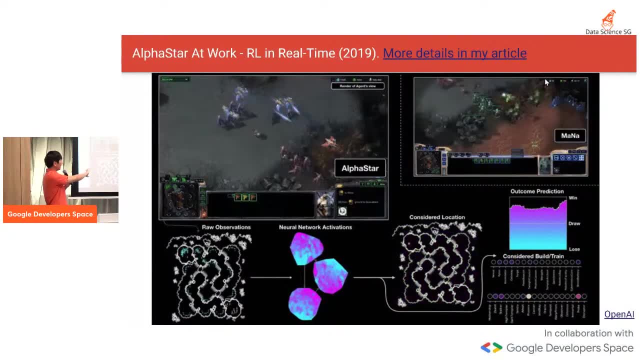 I watched Starcraft for the past 10 years And first thing that Alphastar came out in 2019, and this is the entire paper, the link there I got article talking about it- is that it's able to deal with this real-time system. 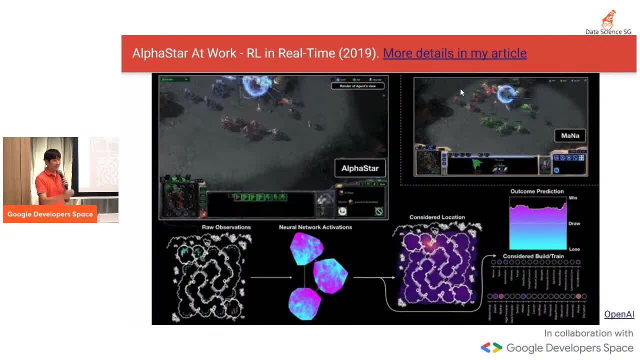 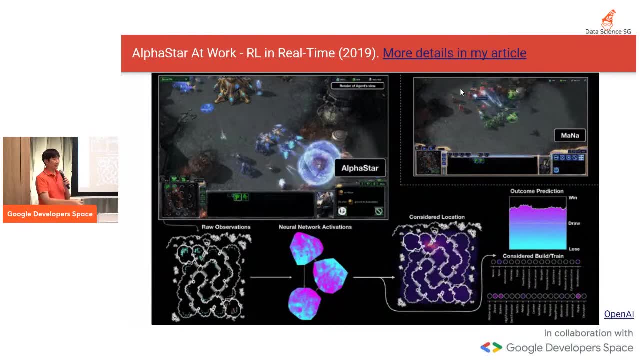 Real-time is important because a lot of our world exists in real-time, not just the MDP world. MDP is kind of like the static version of the world, A lot of things. if you want to use it in healthcare, you want to use it in robotics. 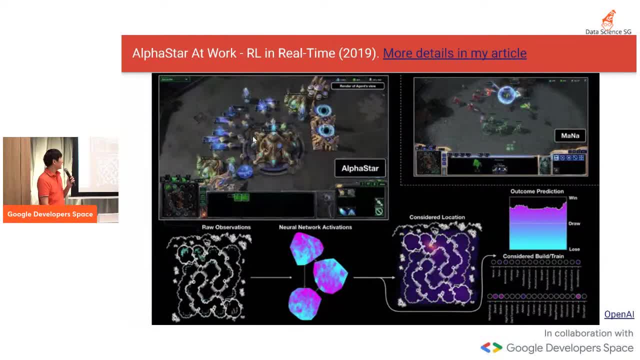 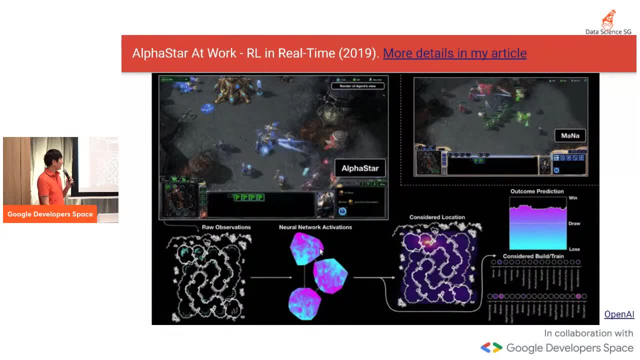 you need to deal with things that happen in real-time against the environment or against some adversary. In this case you're commanding armies and stuff. More importantly, you're looking at various neural network activation decision points and the entire kind of tree of 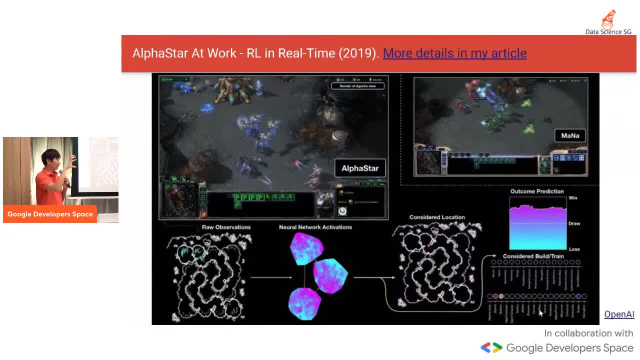 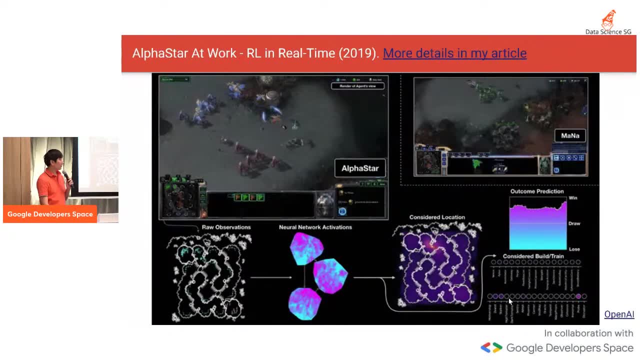 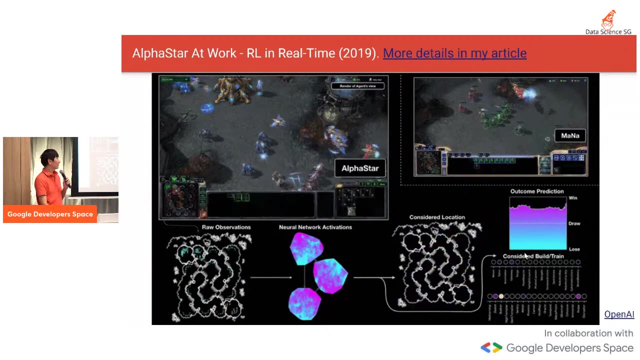 Neural network and reinforcement learning together. it's no longer a tree-like structure but we tend to kind of visualize it as various neuron layers and each neuron layer will try to kind of explain it by its targeting a specific. for example, it's a building layer. 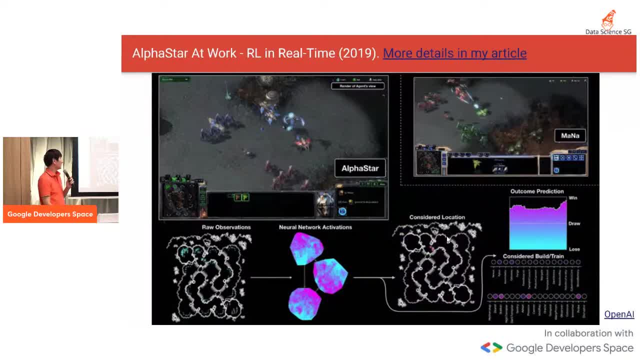 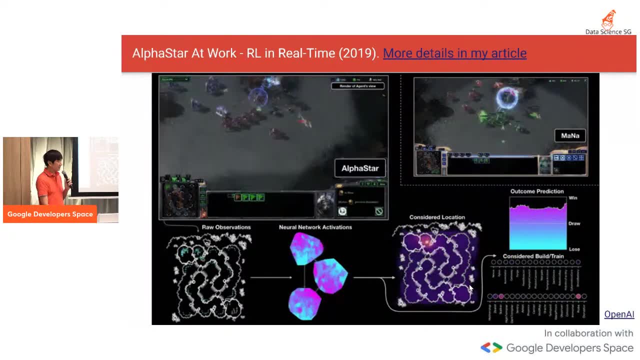 it's a unit layer controlling the unit, attacking layer, things like that. But it's not that clear-cut, But either way. so we have all these various pieces come into play, Most importantly, you see, right for supervised learning. 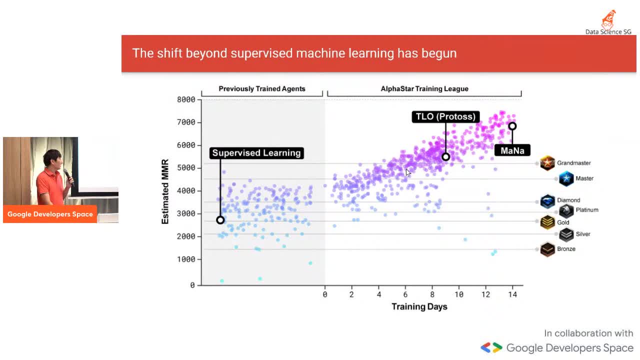 you will never reach professional level. never, Because it's a real-time strategy game because there are a lot of factors. But for reinforcement learning agent, you reach basically the top. so, grandmaster and above, for the MMR, it's basically top 1% of humans. 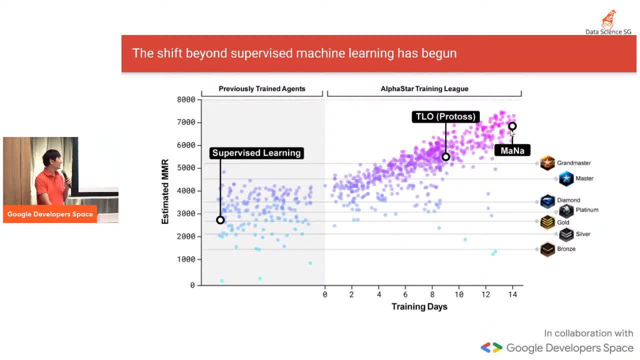 In which Mana is a player that play against the AI. it is about superhuman levels. 0.1% of the human race, The alpha star, can reach this superhuman level, And it does that by a combination of playing against itself. 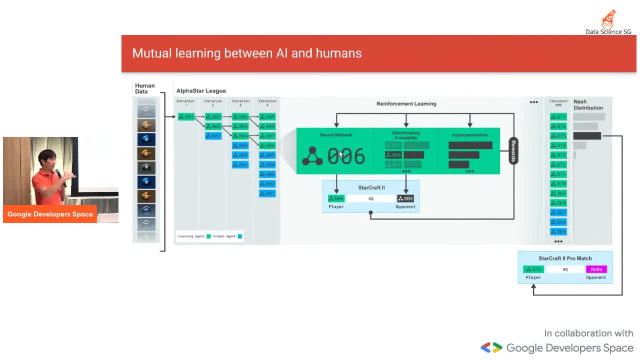 and also studying how humans climb the ladder. So humans get better by playing against himself or herself And, more importantly, learning from experience. number two And number three is to combine different strategies. You don't do the same thing. You do different things in different combinations. 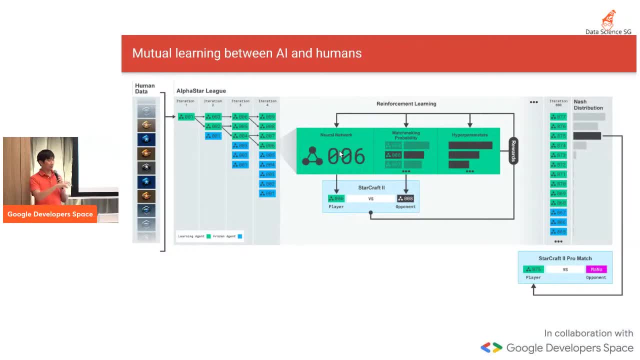 in reaction to something, And all these are reinforcement learning attributes, So you can think of it as you build. a supervised learning on this wouldn't make a lot of sense because you need all the data of all the players that ever played and you still can't match. 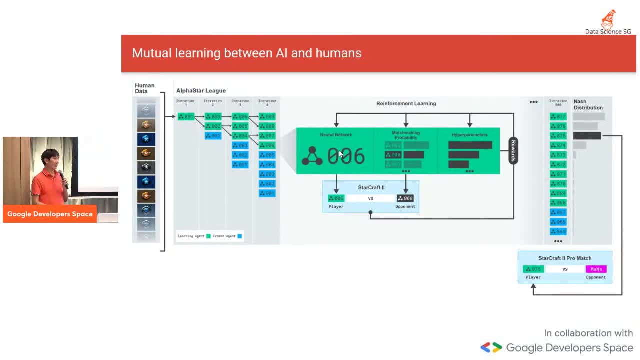 the best player in the world because they have that innovation flair. They have that particular style. You need to be able to gain that X factor. so-called And supervised learning is always looking backwards, So that's always the issue with some of this. 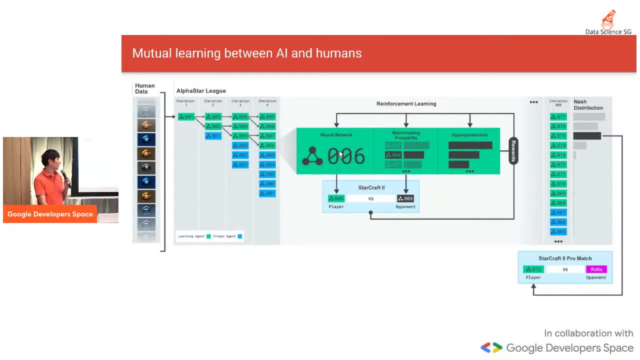 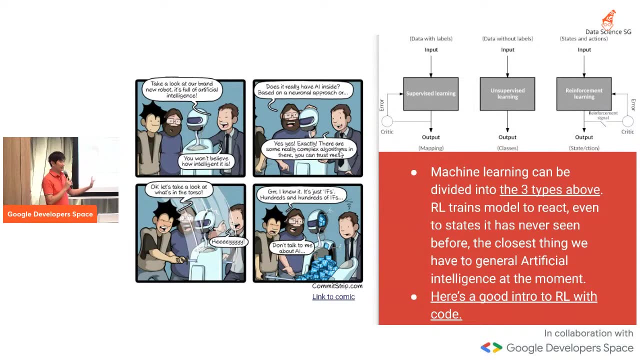 It's still a bit of rubies and a bit of hard to catch up with professionals, So hence this thing. you see a lot of AI products out there. I'm doing AI. So all these software companies, vendors behind the scenes. 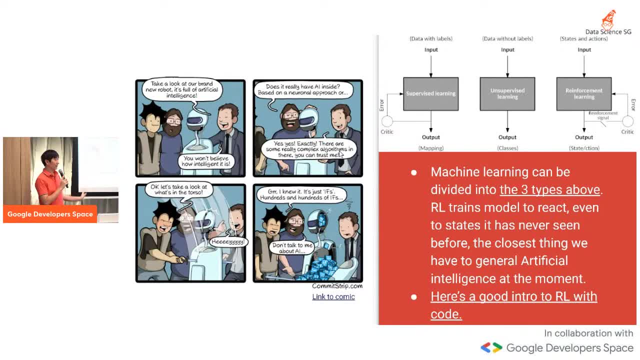 or ifs. So I am in the fraud space. We do a lot of vendor talks. All of that- AI products is all a lot of rules, a lot of if statements as foundation, because that helps to frame the problem, And then they'll do their fancy algorithm on top of it. 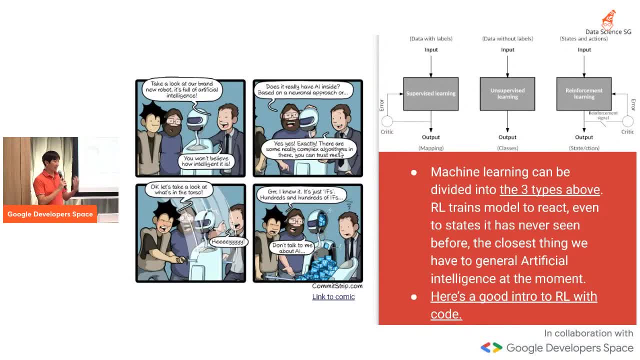 But why don't you just start Some problems? maybe you want to start just from the reinforcement learning approach, So it's kind of a third way of looking at a problem beyond supervised, unsupervised- That's the gist of it. Again, it's many, many years down the road. 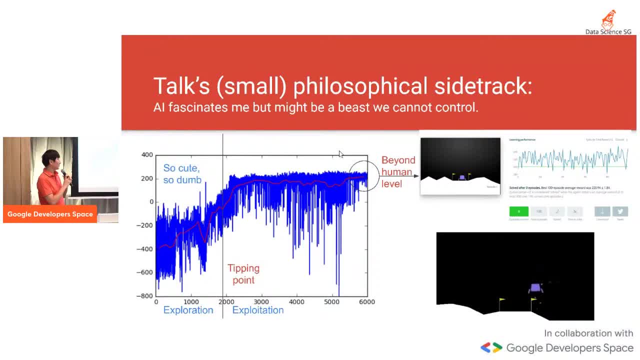 So I accelerate some of these things, But a sidetrack is basically when you see. so this was I trained when I was a student at Georgia Tech And one of the things there was the beyond human level. Now you see, all these crashes right. 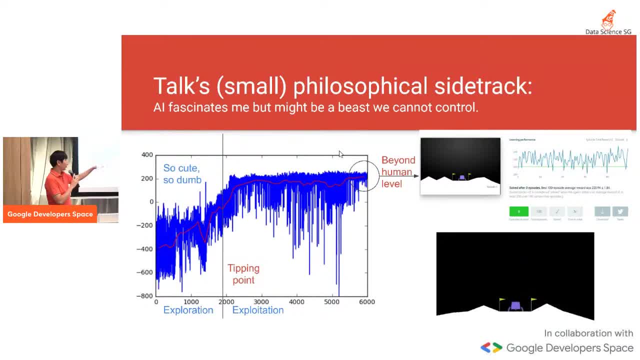 It happens a lot for DQN, But nowadays, the technique I'll share today will take away some of this instability And you will have this beyond human level plateau up there: Consistency. One of the scariest and most powerful point of reinforcement learning is once they get to that superhuman. 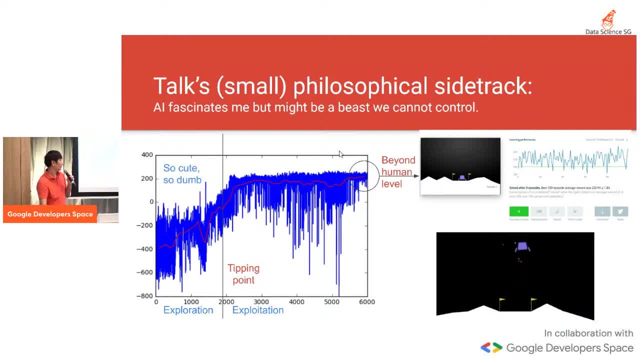 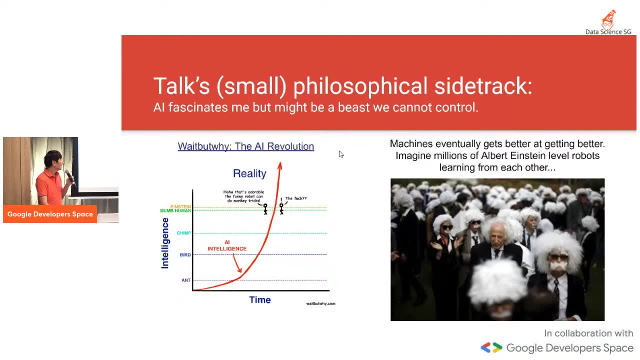 level, you'll always be superhuman. Think about all the alpha star, alpha gold, which is why it's exciting, It's radical, It's rather stable. surprisingly, once you learn how to do a certain job well, And this article is talking about, once you, 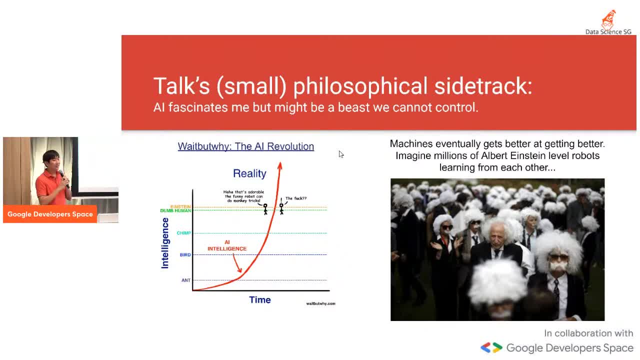 reach human level, the average human level. it doesn't take long to reach your Einstein level, And a whole bunch of Einsteins talking to each other will create this entire super AI thing. We are maybe not in our lifetime, maybe the next lifetime perhaps. 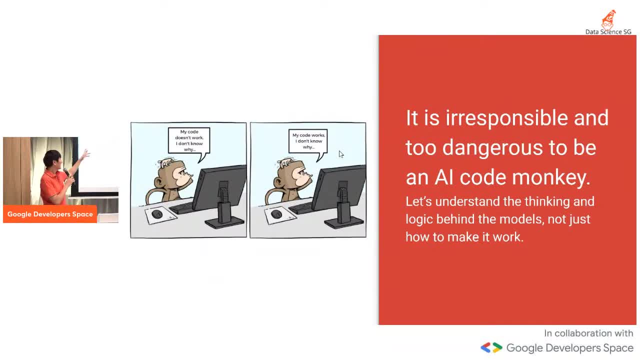 But, most importantly, when you're doing this kind of work, you will see that you have no idea why it works. You have no idea why it doesn't work, So it's very bad. So that's why we try to have more talks like this to share. 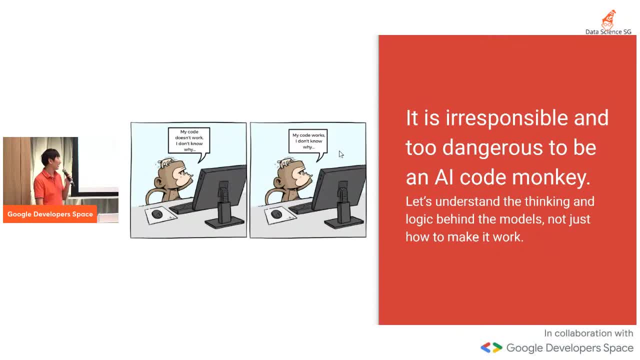 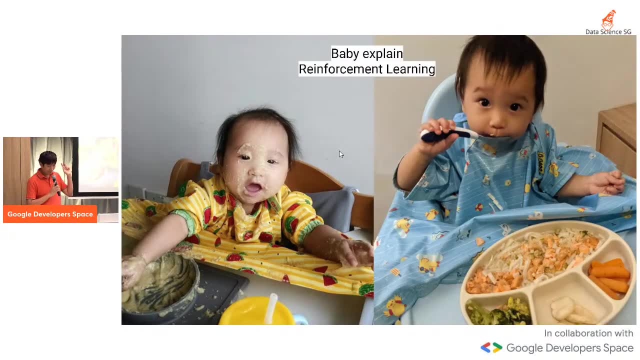 about the process of looking at it and have at least some understanding, not just being cold monkeys. So, as you see, the agenda is quite packed, but we'll just go straight. So this is my: I have a girl, so a baby girl. 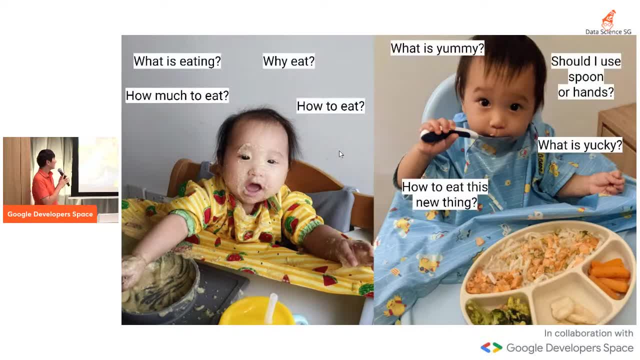 And the baby will let the baby explain to us what's reinforcement learning. So for her, when she start eating, there's no concept. So it's a very common problem of reinforcement learning: There's no concept of eating. But how do you actually get it? 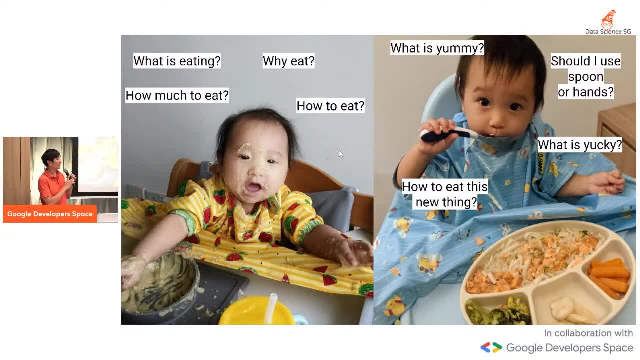 How do you get from here all these questions to a definite, more structured questions? right, What's yummy? What tools do I use? So that's what the Tuya mentioned. right, Environment, state action, This environment of eating, to that thing. on the right, 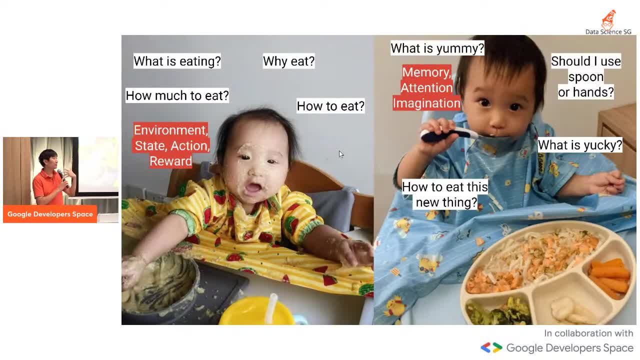 where you talk about memory, you start storing knowledge about the actions you can take, the results of it. Attention, how do you focus your attention on eating, using the tools Imagination, being able to kind of go a few steps further than what you have seen before? 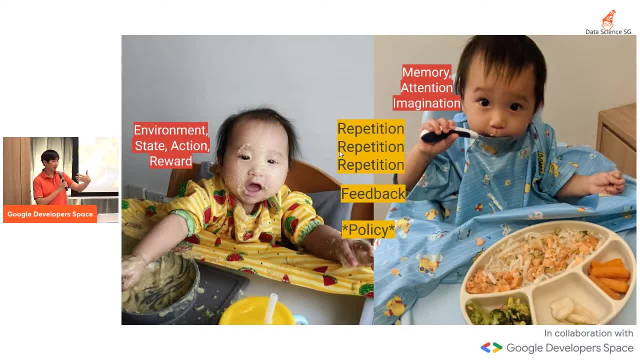 So all these are concepts that are very important for kind of practical RL. It's all about repetition, all about feedback loops and all about the policy Again what Tuya mentioned right. So those are the key of it. The Tx problem we'll skip. 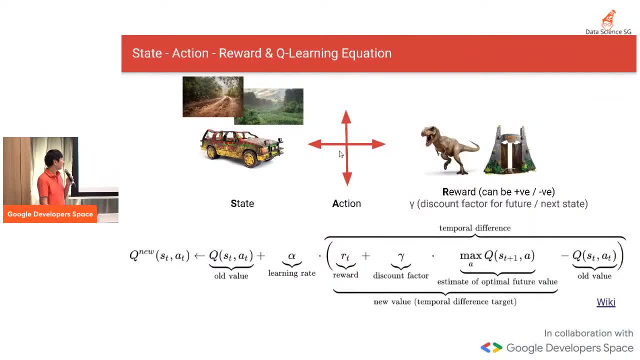 Same thing as what Tuya mentioned: have the greeting, try to have this policy. This is a formulation that for temporal, this captures the temporal difference and the state action. we want to learning Long story short right when you want to update. 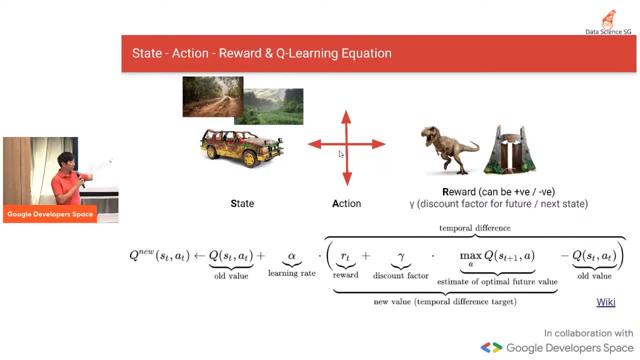 a value, so we call it a Q value. right. Reward is given at each action you take. So in this case you want to escape a T-rex. A negative reward is you get eaten. Negative 100 points reward immediately. 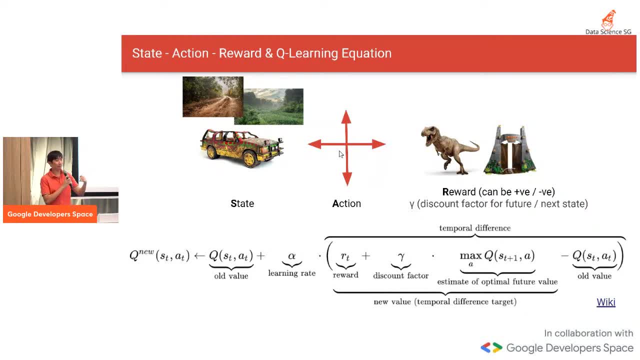 So that's bad. You escape into the safe area plus 100 points. So that's an immediate reward, But it's discounted, So that's where the temporal difference and all this come in- Discounted because you want to build an agent that will learn. 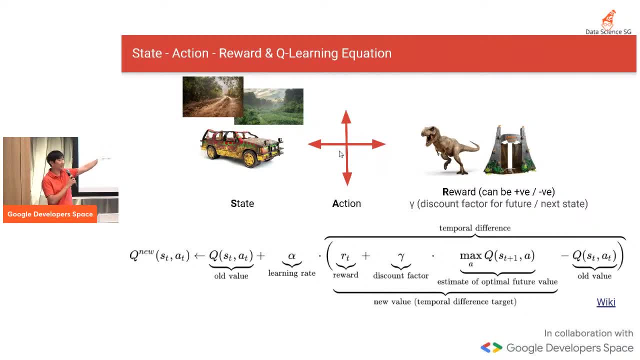 not just to avoid the T-rex, Not just to get to the exit, but the entire pathway to avoid the T-rex and get to the exit. The journey is important very much, more so than the outcome, actually more so than the learning. 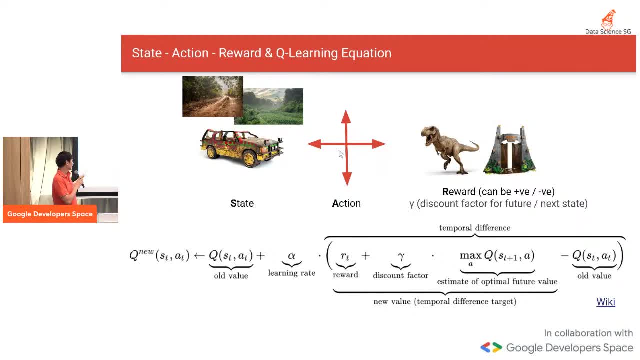 Hence this thing is crafted such that you have a learning rate where you update your value. So remember, we want to store value in the grid, right? Your O value is updated with a discount learning rate based on how fast you want to change your typical learning. 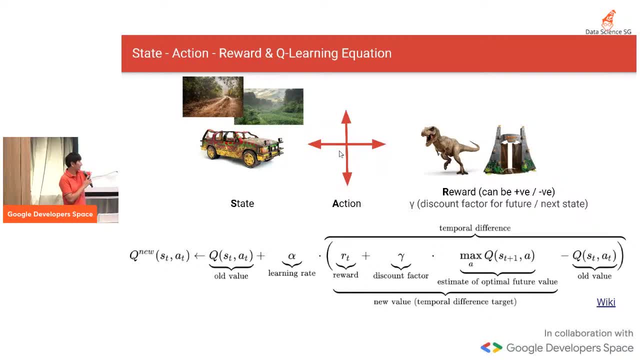 rate. So it's the same concept With a discount factor of your future value estimation. So, based on what will happen, you will get closer to T-rex- higher chance to get eaten. get closer to your exit point: higher chance to escape. 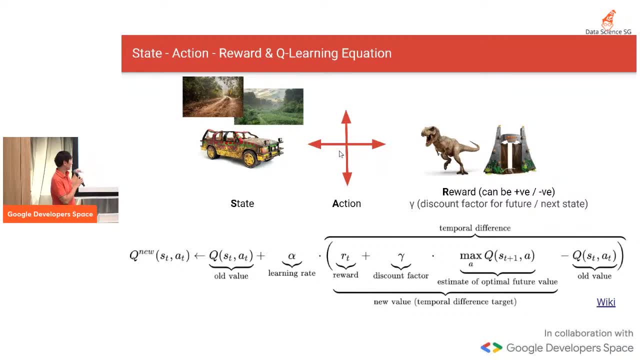 So all this will be discounted and added to the temporal part of it And this will be basically added to the Q value. So Q value is capture. It captures the reward: short-term reward, long-term reward. That's what value function means. 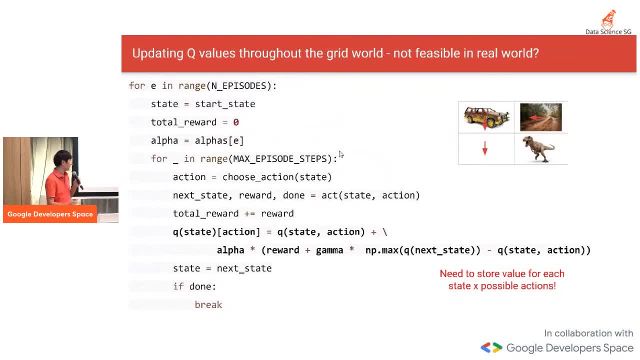 The wiki is actually very good, So you can see it's a wiki link. It explains the whole thing nicely In code. it's actually not that bad. Code is actually a literal translation of what you've just seen And nowadays- later we'll see a lot of the functions. 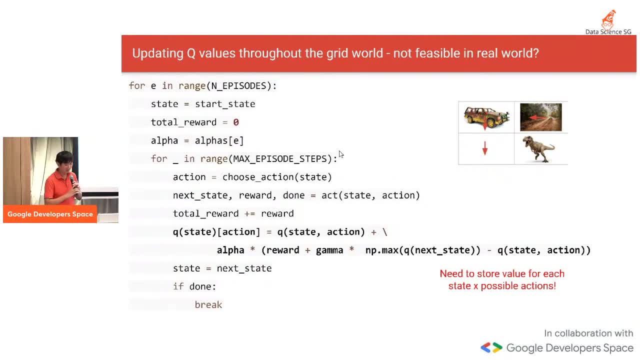 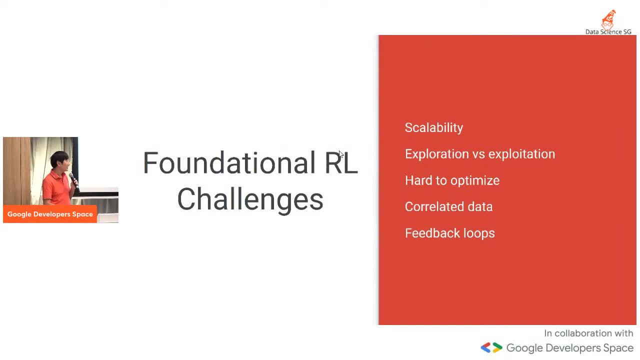 You don't even code the Q value out anymore, You just call it like a secular, like that. So we'll talk about that later. Some challenges we need to get through these pieces. These pieces will help you understand a lot of papers and a lot of the work that's being. 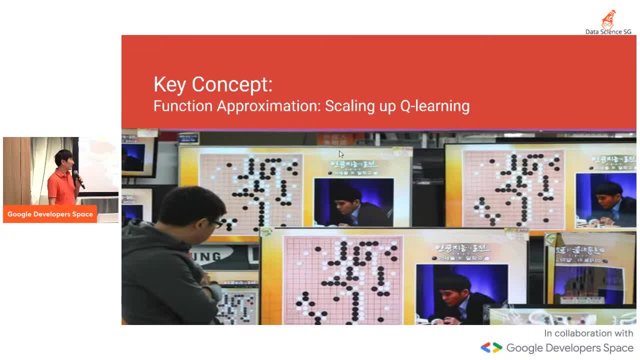 done in the modern approach. So again it's a bit It's abstract, but when you put it together in the code you'll see how all this works. Doing grid doesn't solve anything. I mean it's a very good tutorial to get started. 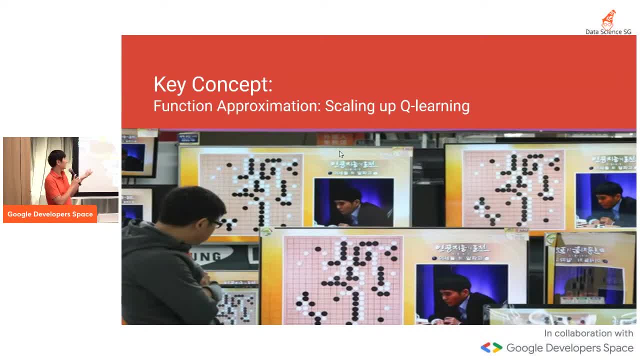 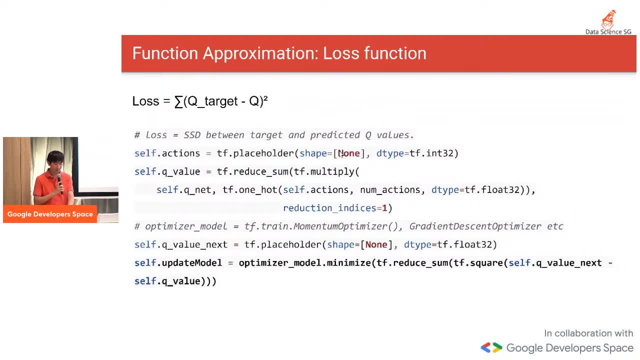 But doing grid work doesn't solve real-world problems. Hence we need functional approximation. We cannot calculate every single grid score, Not possible in the real world. For example, in gold there will be billions of stars equivalent billion upon billions of combinations. 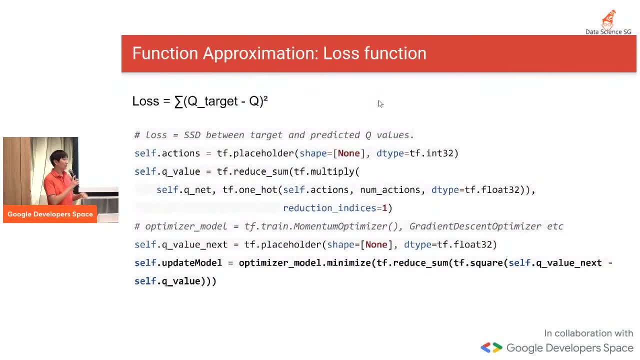 Not possible to figure out the grid, But in the super-world it's possible. In the supervised learning world we know how to solve it. We use a model to represent. Let's say we want to build a fraud system. We don't need to have fraud data for all the combination. 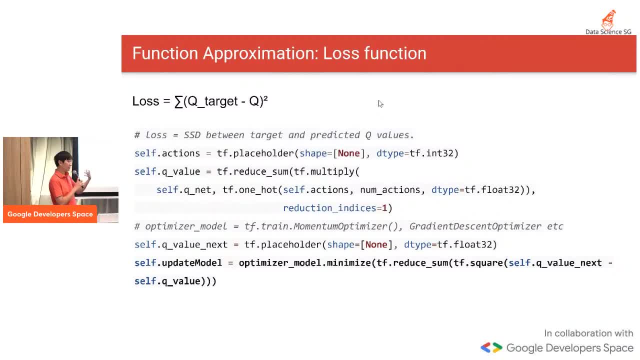 We can have a fraud model, a best fit model to represent fraud in general, for this particular kind of fraud, for example. So similar concept: we build a functional approximator to approximate what will happen if we take the action without taking the action. 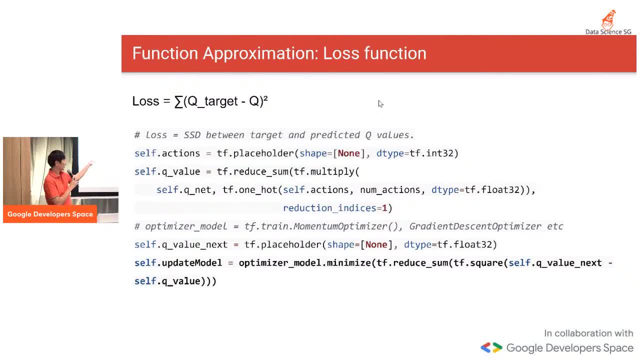 So we use some of the things that we learn along the way. So as the robot drives around, you pick up some of this reward function, things like that- the reward value up the Q value, And then we do a function- approximation. 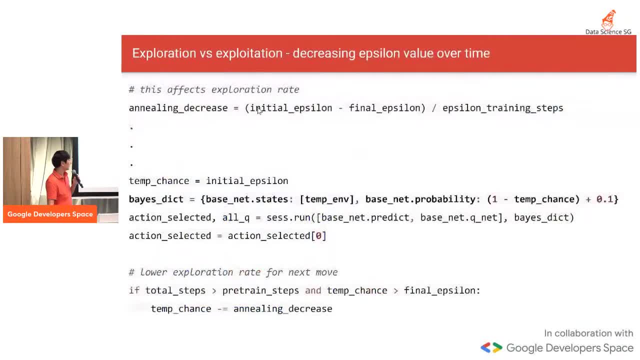 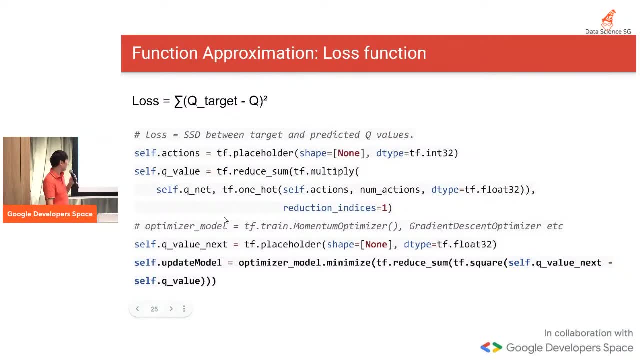 and we focus on the loss. So a large part of the models are about this loss function, how to optimize it. This is very old code. This is many, many years ago. Now there are cleaner ways to write it, But long story short, there's an optimizer. 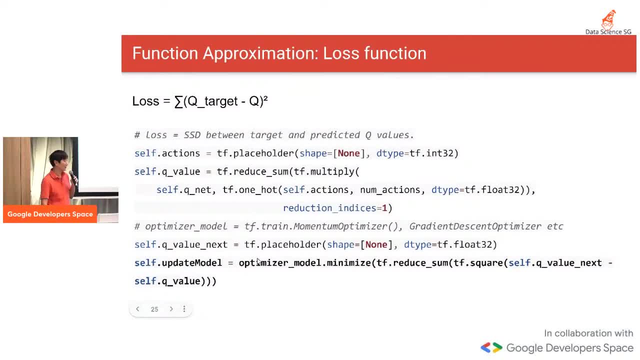 and we try to reduce, basically, the loss function based on the difference between our function, of course, and the loss function based on the loss function. So that's one of the things that we learn along the way. So that's the functional approximator model. 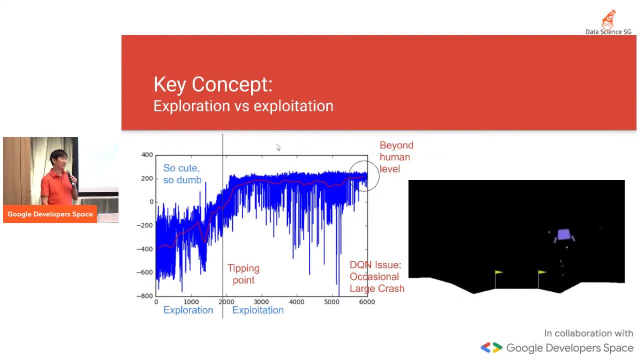 and the somewhat actual value that we can derive from VFCN. So that's one Functional approximator. helps you scale up Exploration. exploitation is nothing new. A lot of the models supervised modeling model does it. So more importantly is, how do you balance it? 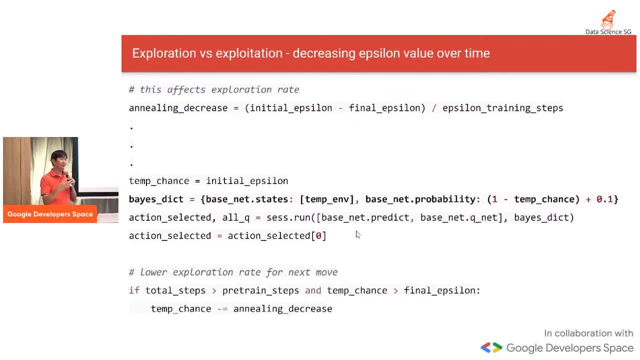 So the epsilon decay is a typical again from supervised learning world. epsilon decay, things that will have this temperature thing, So you can do this with a lot of knowledge to be able to run it. So there's this probability thing that will. 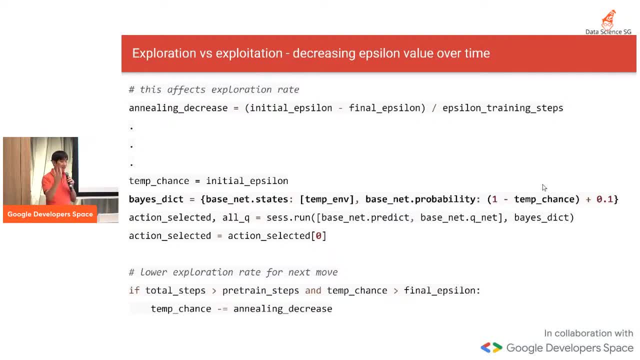 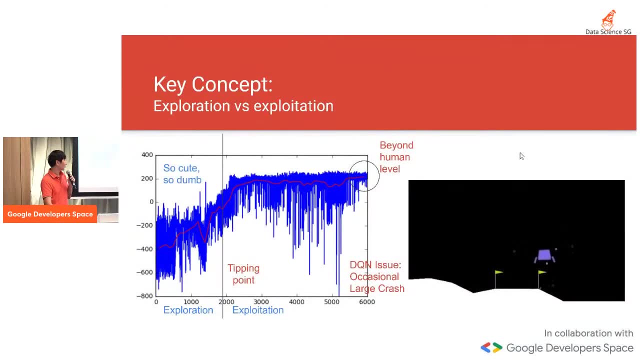 base on the change over time. So at first the probability of taking a random action to explore is very high And over time you become less and less random. You'll be able to do the actual action, the most optimal action. So this part is the so cute, so dumb phase. 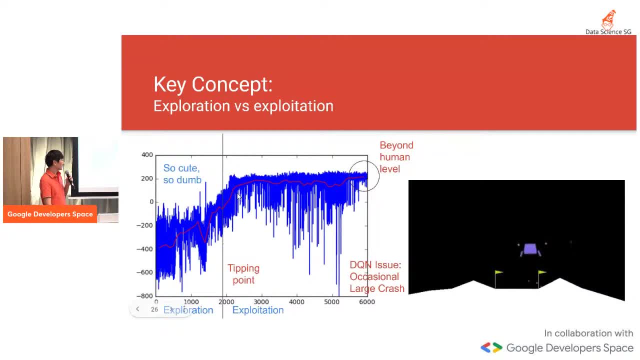 You see, it's crashing, It's flying all over the place. It's not doing anything that's useful. It's building up the ammo, building up the knowledge. Then it goes to the tipping point. You always see that, And then you have this beyond human level. 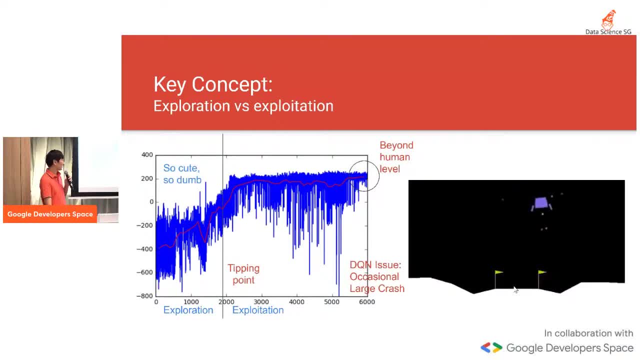 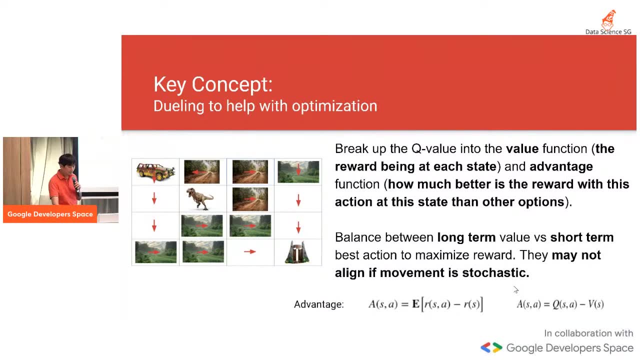 And you see, the robot is landing better and better into the thing, Same as the driving it gets better and better. So that's the exploration. exploitation, Bureauling is important. So we talk about Q-value. Q-value, it balances the long-term, short-term. 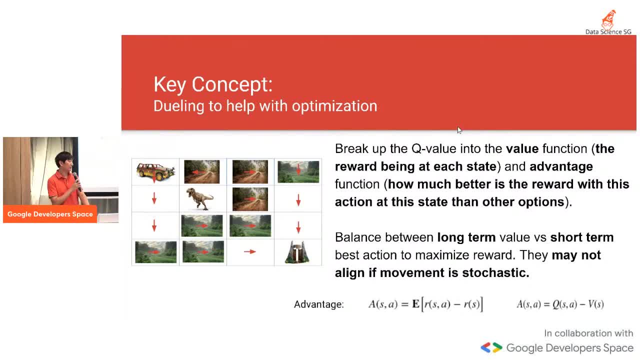 There's also a huge concept of advantage. So you see all the recent paper talk about advantage, all the recent algorithms use advantage. Advantage is the advantage of coming to the meet-up today versus staying at home. So the advantage you gain today, hopefully, is knowledge, fun, friends. 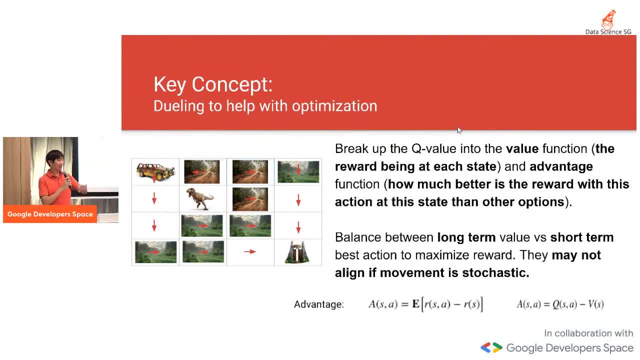 So those are positive things versus staying at home and being depressed, sad and by yourself, things like that. But you get to have a nice meal at home, So that's straight off. So advantage is against your next action, other actions, other options. 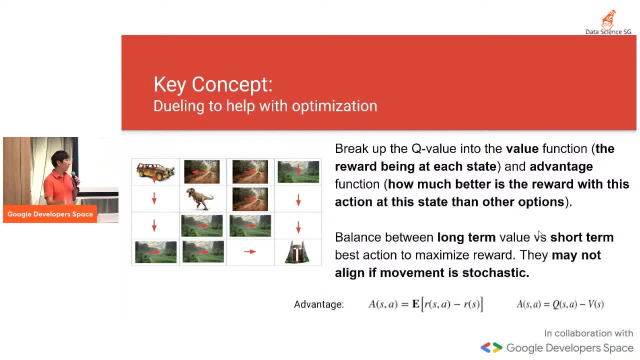 So advantage is a very interesting concept Because it now compares your- Yeah, Not just the long-shot reward, but this reward against other rewards I could have taken. And you'll be surprised, as you optimize advantage across the network, what I've seen before. 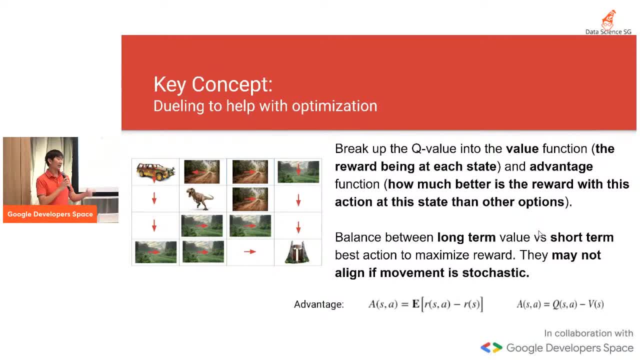 is, you can take a disadvantage position, And that happens in AlphaGo. when they explain why AlphaGo wins or even lose, as they say, though You take some very strange silly moves or not efficient moves so that you can gain the advantage 20 steps down the road. 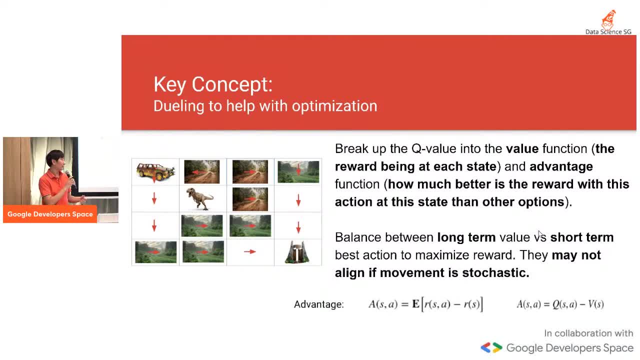 So this particular seat that you place, this particular move that you play, can be used to your advantage. So it's a long-term thing, but also can balance the other trade-off, the other moves that can branch from this. So that's a very important concept. 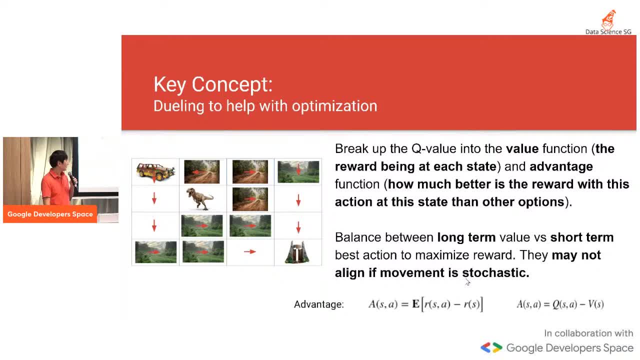 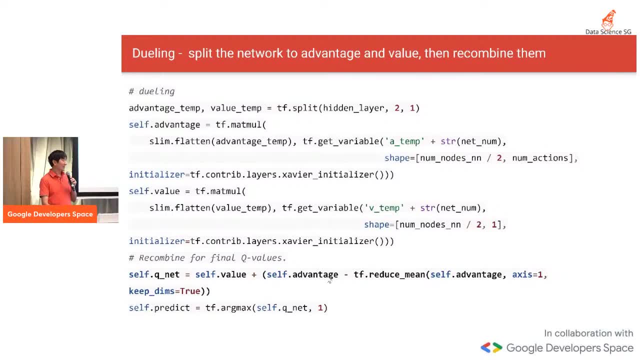 So advantage calculated like that And advantage code-wise again, is very simple. You just play up the view, the value and find it, So you can see that actually back-end again you don't implement advantage anymore nowadays. 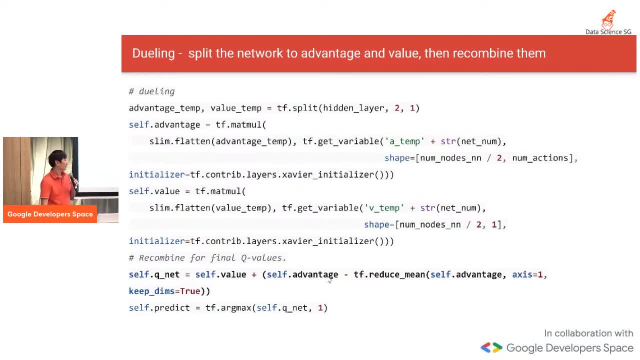 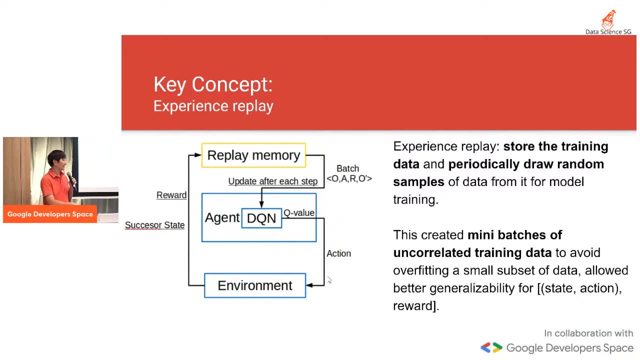 You just call it Back-end is not that hard. Back-end is just spitting it out. There's a lot of math to prove that it works. There's a lot of concepts behind it, But the actual code itself is not super hard. 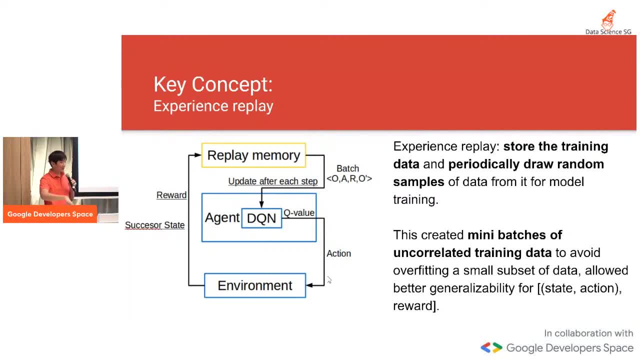 And that's why I'm trying to bring it across as well. When you bring everything together, it's super hard, So don't try to code reinforcement learning algorithms from scratch. You'll die. So use a package. Yeah, I'm just telling you, this is how it works. 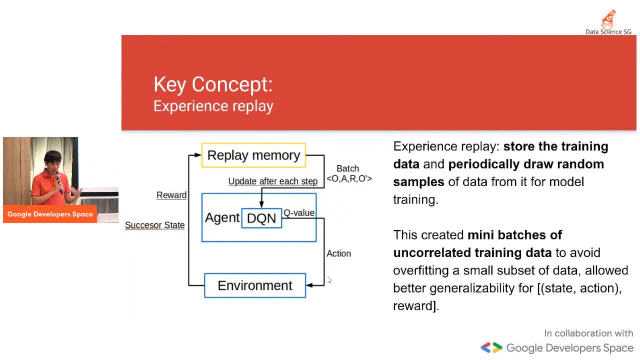 So Now, experience replay- very important Experience and all this that we mentioned. Yeah, The experience replay actually get a bunch of batches of experience so that you can train your model. For example, car Parking a car. I want it to learn how roughly to deal with situations to move backwards. 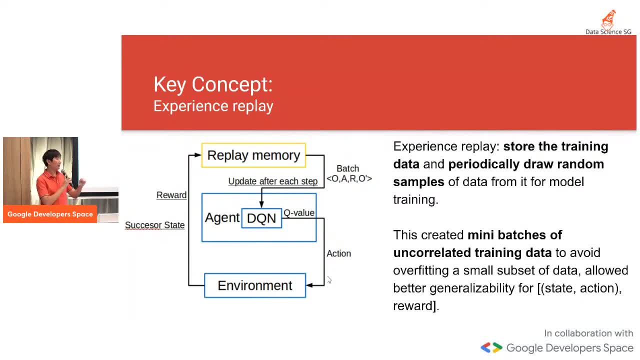 to turn the vehicle. I do not want it to remember the whole sequence Because this sequence will almost never occur again in the real world. It will always be slightly different. I mean for those who have seen people park cars Like drive yourself, right. 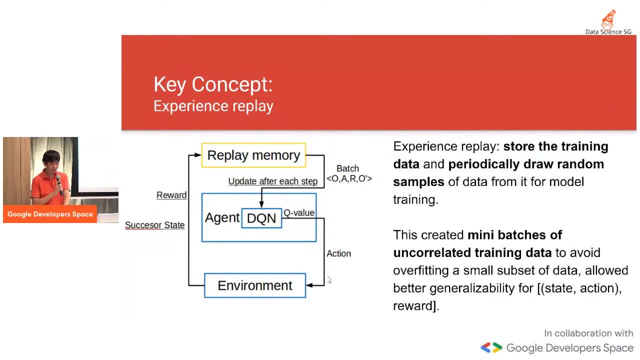 You will never get the same situation. So spin out the mini batches And also later we'll talk about some other, more intelligent way of using experience. It's very important, So experience itself is an asset that you must fully utilize, And there are many ways to do it. 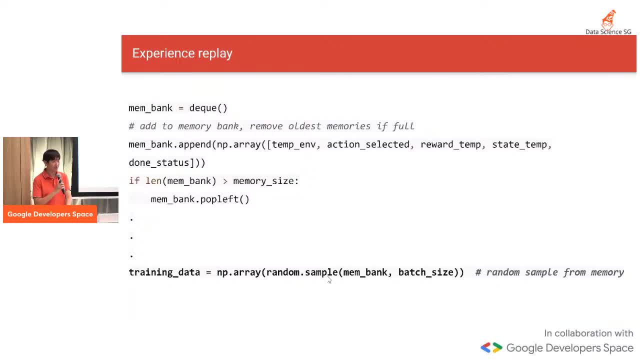 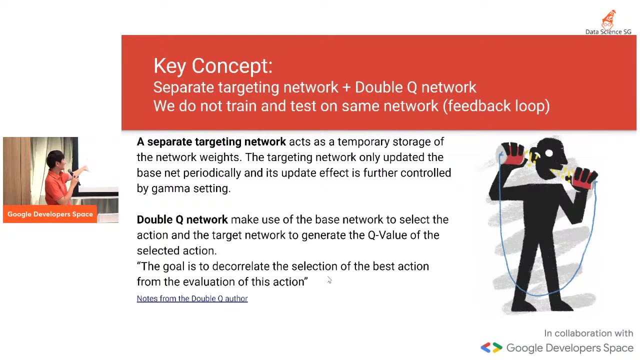 And we will learn about hindsight experience later. So it's very fun. Okay, Almost there. So separating and doubling- So again these are keywords that you will hear a lot in the papers and the methods: Separating the target layer and having a separate target layer and value layer. 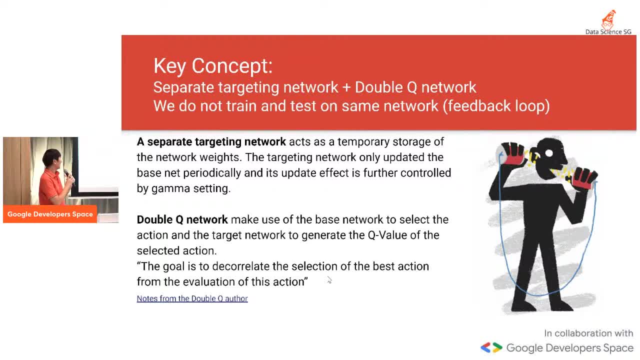 We will see that image later- And having double queue network to kind of want to generate and want to select the action, This will help with some of the adversaries that are coming. So I think that's it, Thank you, Bye-bye. 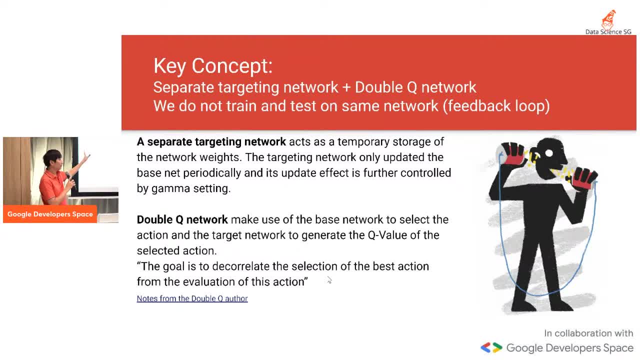 Bye-bye, See you later, Bye-bye, Bye-bye, Bye-bye, Bye-bye. This one actually improves the performance, but not overfitting your single policy. So you have two layers: Actor critic, for example, is this one. 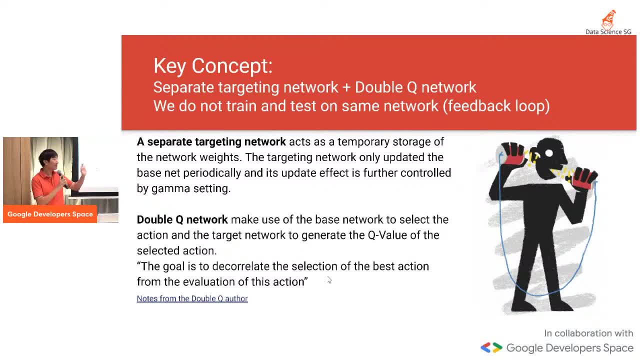 The purists will argue with me that double is different from actor critic. But actor critic is one way that you can visualize having two separate networks, One person scolding you to drive better and you drive, Rather than overfitting everything to just one network. I am the driver, I am criticizing. 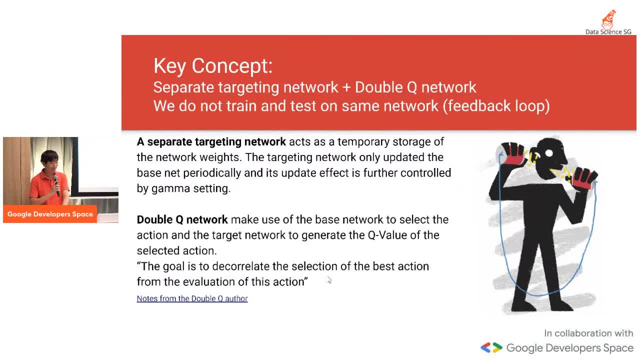 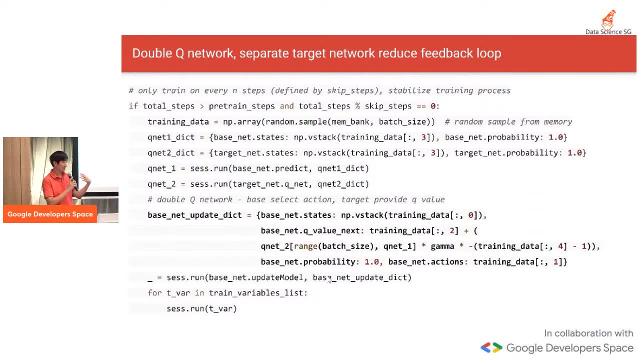 myself. I am criticizing myself, madman, scolding myself. why am I not parking it correctly? That doesn't make sense. So having multiple layers of network working together protects the integrity of the model better. So the question was about poisoning If 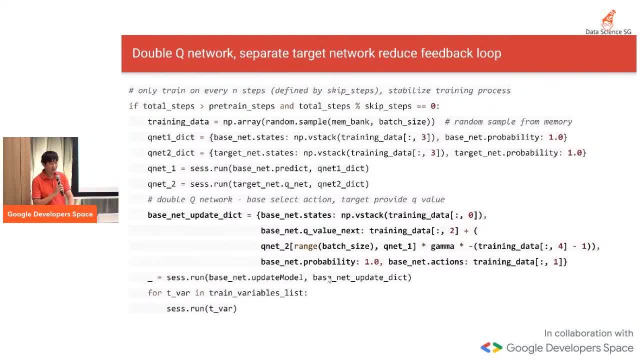 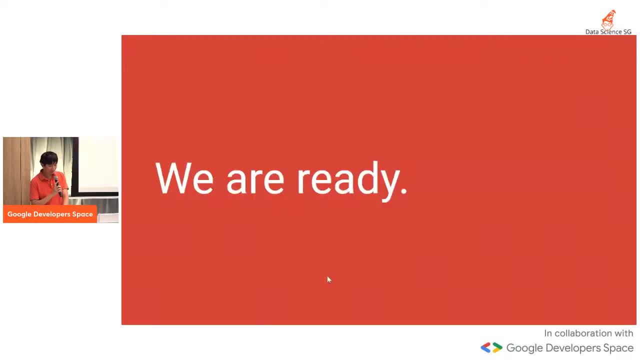 an adversary tries to poison your reward function. having multiple layers- double queue network, separate target network- will help reduce feedback loop and protect your training better. Okay, we are ready. Do you feel ready? Don't worry, Reinforcement learning is something. 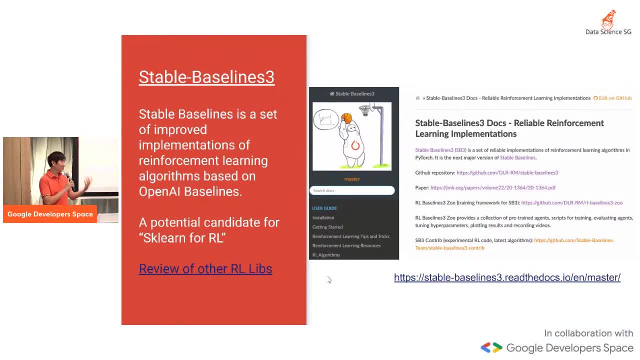 that you go again and again and again Reinforcement learning to learn. it is like reinforcement learning process. You look at it again and again over the next few years and eventually you'll get a bit hang of it. hopefully Stable baseline is the scikit-learn candidate. 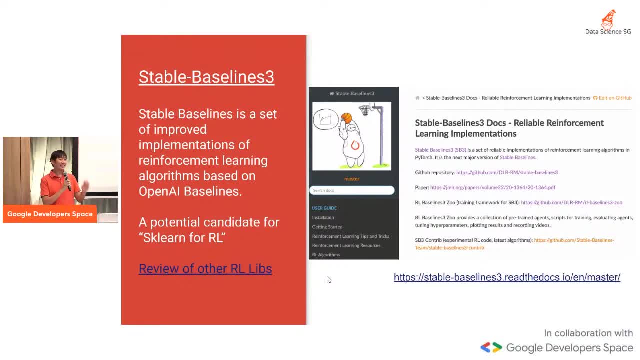 There are tons of candidates. Again, it's like Wild West. Think of it the days before scikit-learn, Think of it the days before XGBoost, Think of it before whatever TensorFlow or PyTorch, Before all these things are invented. how? 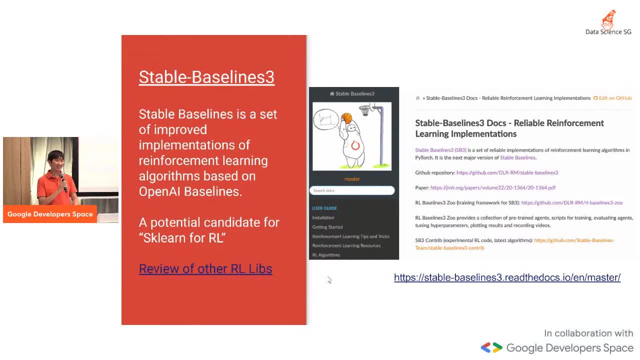 all these things are invented. how messy it was. There was no NumPy, There's no Pandas. I came from that time, Before all these things were invented. this is reinforcement learning stage. Nothing is standardized and stable baseline wants to be one of the standards. 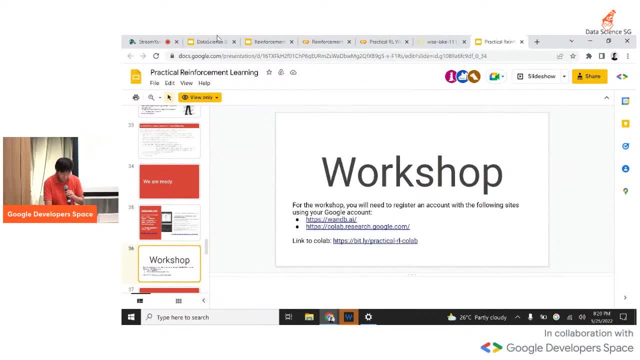 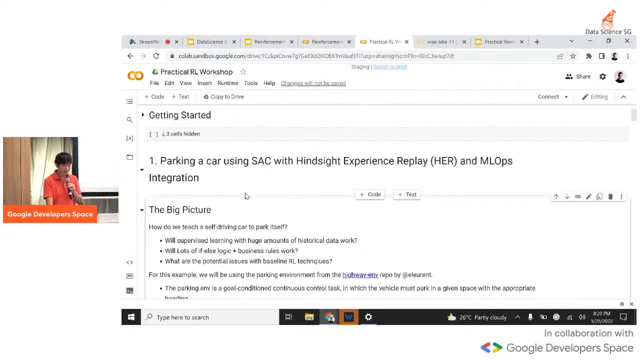 We'll see how it works a few years down the road. Okay, I got apparently 10 minutes to finish up, Let's go. Okay, Again, the slide. the first thing we have- all this Let's talk about this- is a Colab code. 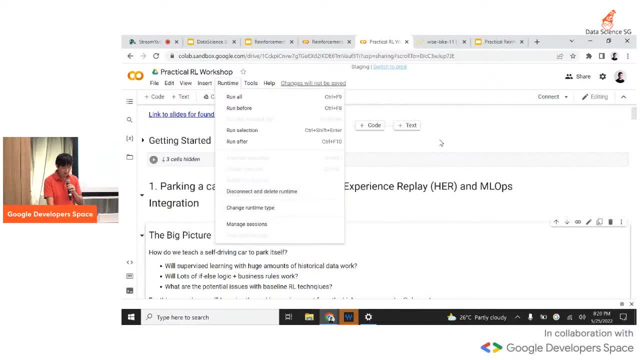 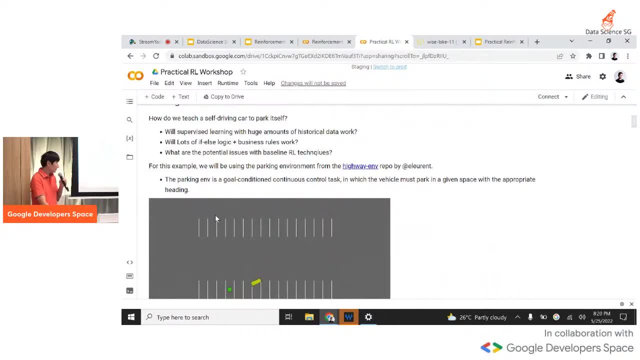 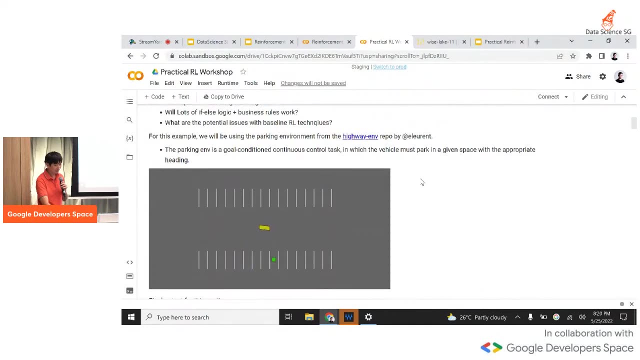 Remember to for the runtime environment. remember to set Set your GPU, Get started when you install the package. We'll go straight into hindsight: experience replay and her. How do we teach a car to park itself? Some questions here. Realistically, parking- is we call it a goal condition? 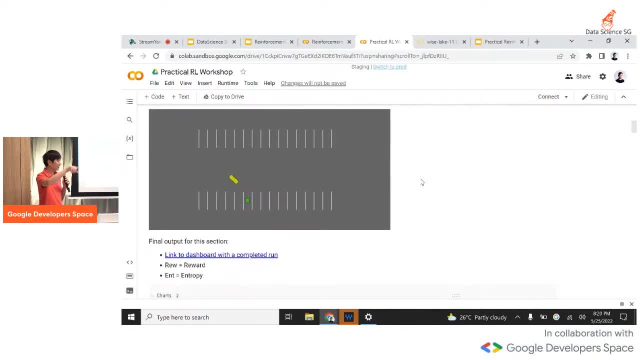 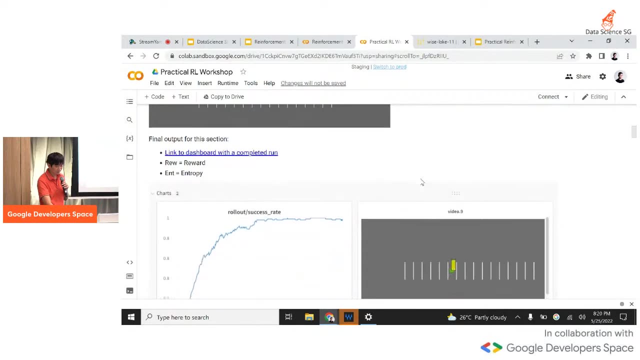 continuous task. You basically need to. there's continuous action behind the scenes is way more complex than your usual MTP already. You need to basically teach the model to run to drive. There's an angle, There's acceleration, everything. It's quite a nice simulation of the real thing. 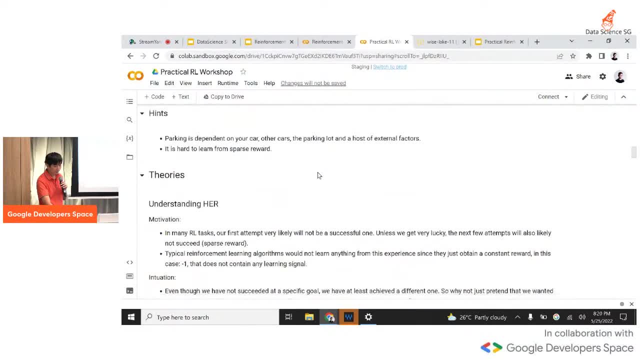 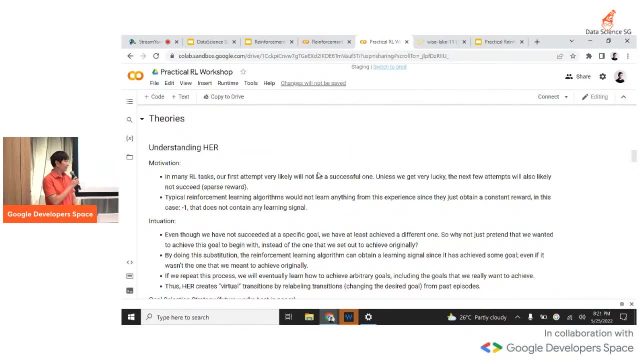 Then we have this entire dashboard that I'll show you later. But one point is: understand. her Experience can be used in many ways: Hindsight, experience replay, replace your experience. Think of it as the baby- actually my kid- was learning how to eat. 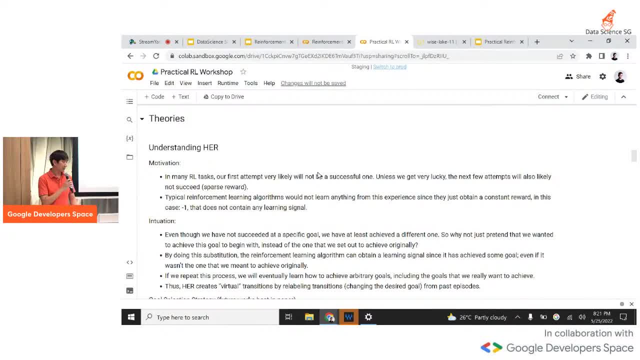 Now the problem with a lot of reinforcement learning, agent training in the real world that I've seen there is it's very sparse, In the sense that there's very, very few success. Your parking will take forever And in fact, cannot be solved until recently. 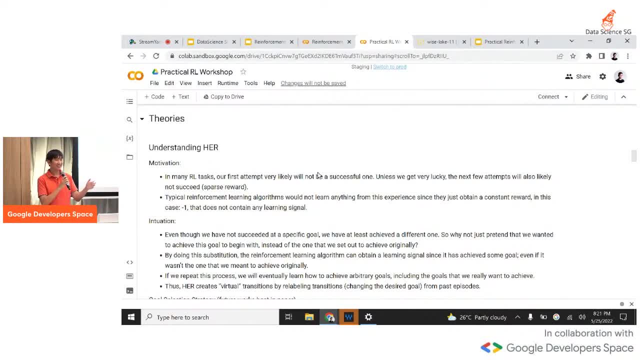 because things like this: you only get points when you park. But it's very hard to teach someone to park a car. teach an agent to park. Even a human to park a car takes months of training to park a car. Imagine teaching an agent which is a lot dumber than a normal human. 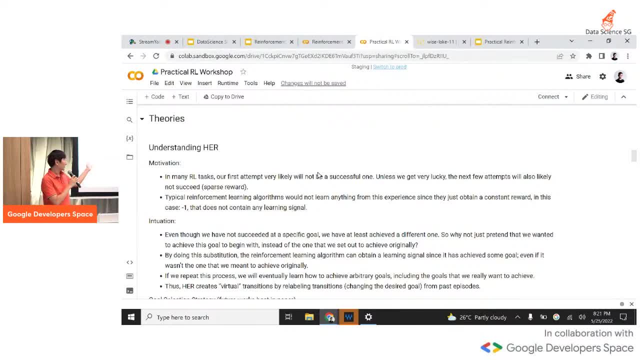 to park a car You'll take forever, Very expensive. Hindsight experience replay breaks down the problem to say that I will give you a reward even if you go backwards. So you start breaking up the parking into multiple steps. You go backwards, you turn, get closer to the parking spot. 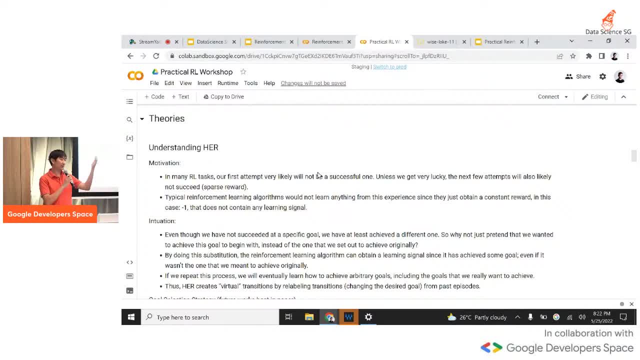 weave in the parking spot, then you stop and park there. I mean it's five or six steps. So hindsight, experience, replay is saying that why don't we, each of these checkpoints, we reward, we set it as the goal that we want it anyway? 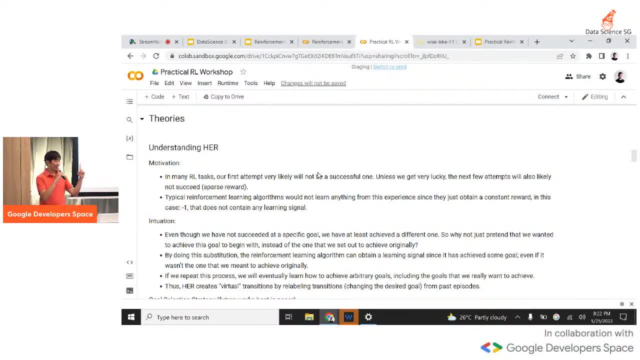 so we have a now, we have a timeline right, We have entire timeline. Let's say, this agent only managed to reach backtrack. You went forward, you crash a wall, do a lot of silly things. It managed to backtrack towards the goal one time. 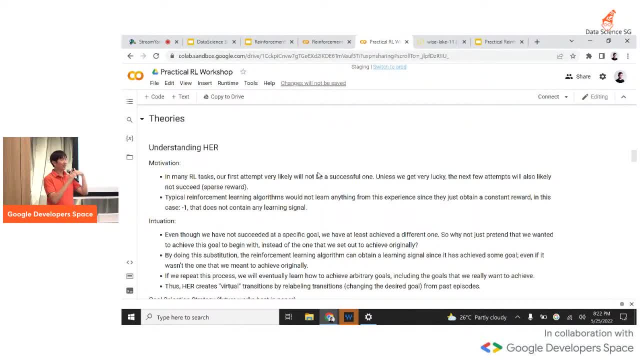 That one time we set it as the temporary goal that we want to achieve, And everything that happened before that will now be scored based on that goal. So in that case, you get some. you don't get a lot, but get some feedback. 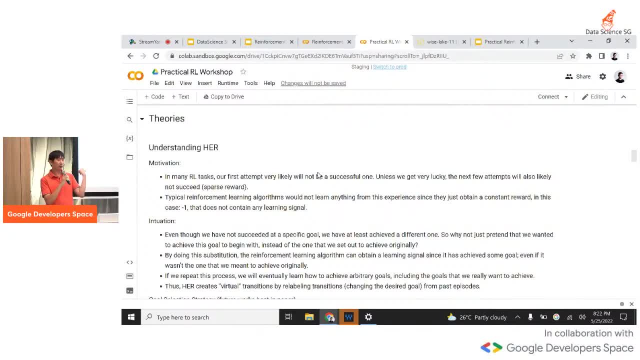 That okay. That is a positive example. You can work the negative example as well. If you crash into the wall, you set that as a negative goal. Crash into the wall is a terrible idea. Crash into car humans- horrible idea. 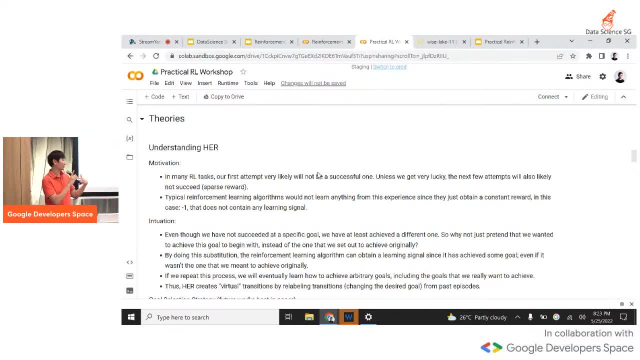 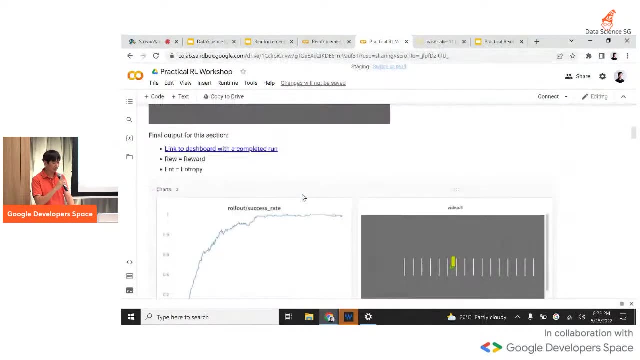 So those can be kind of neat- also part of the hindsight experience- as checkpoints. So what happens is by breaking up your timeline into chunks and then training each chunk as a mini goal, you start to be able to build this repertoire of experience that. 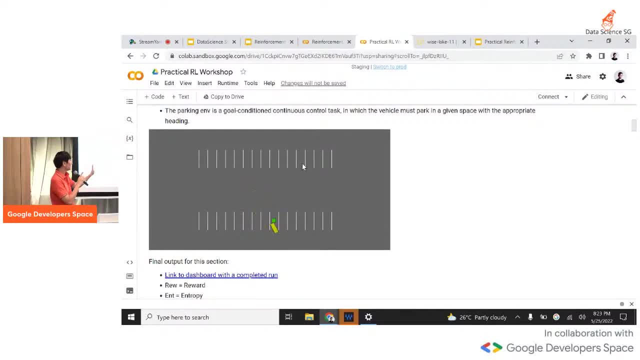 ultimately helps you park the car, And this problem can be solved, And hence nowadays there are more advanced version of hindsight experience. This is the first version of it And in fact, if you see the code, there are only three options. 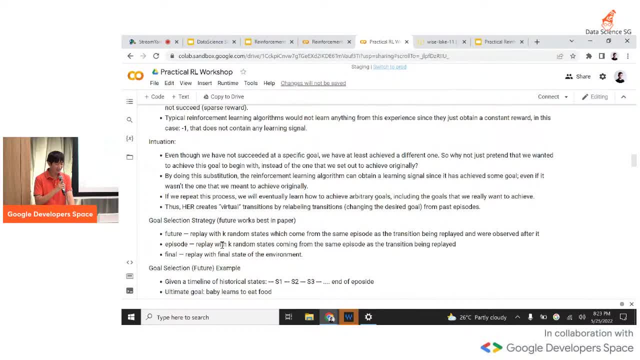 And three options, and two of it is absolutely stupid. There's only one option effectively. You either use the last state. If you crash into the wall, that's the last state. If it just go random direction, that's the last state. 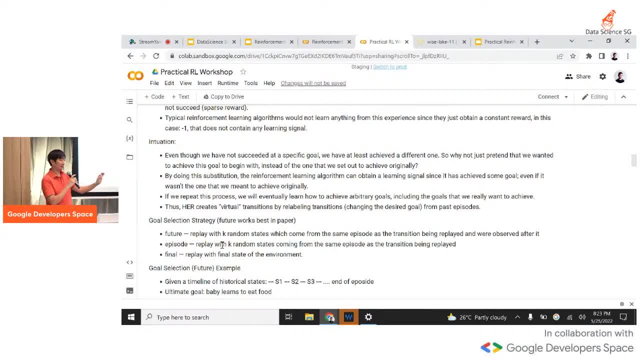 Final is a terrible idea. Episode. Take a random situation. You don't care about timeline, You can take things that happened before. Absolutely stupid idea. These two in the paper. it doesn't work at all. They're just trying to push for a future, which is: you maintain a timeline. 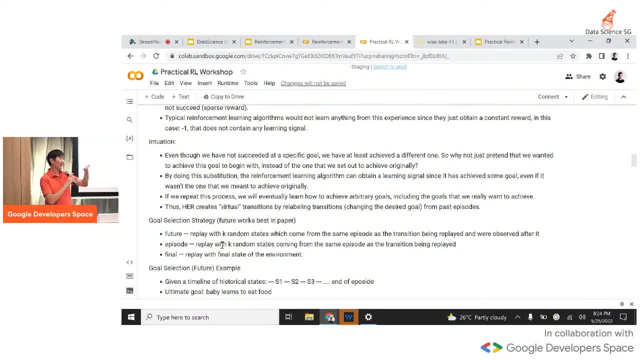 and you take something that happened in the future and you look hindsight. Hindsight has a name. You look backwards. Everything that happened beforehand is parked under this checkpoint as the steps that you wanted to reach this goal, this kind of in-between goal. 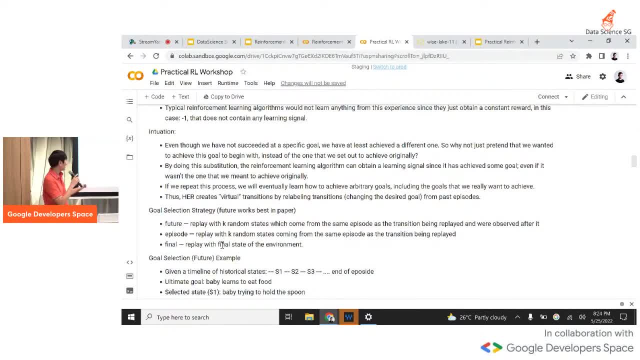 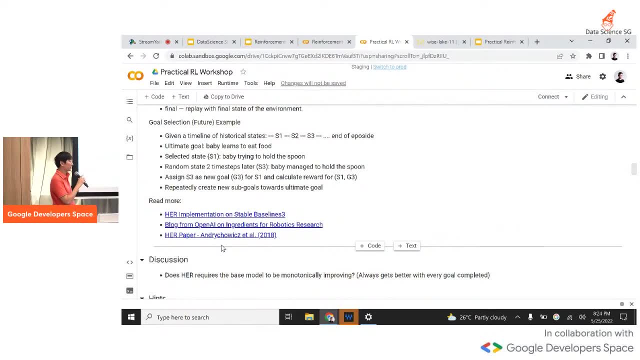 Hindsight experience replay. Ooh, I got five minutes left, OK, So yeah. so why am I explaining all this? Because this is like the foundation for experience replay. It's very hard to kind of conceptualize it without someone talking through it with you. 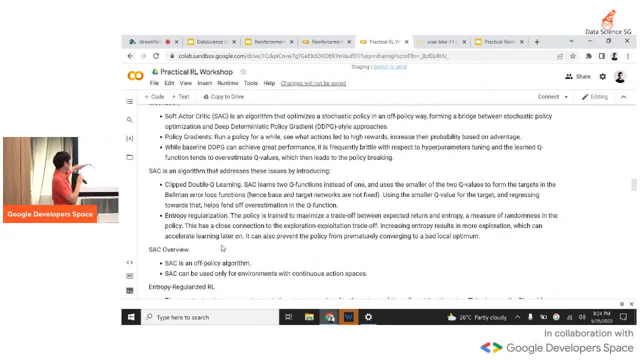 And even then you go home a few times and then you still struggle with it. There's another thing about SAC I want to share, about clipping. So basically this is where we talk about learning two things right and also entropy. 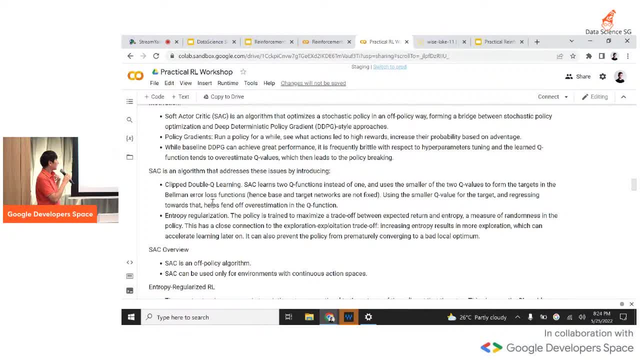 So this part is important. So the clipping is something that has been introduced a few years back Again, more advanced version now. But the idea here is that we talk about having the double-layer. double-layer, that kind of like one create the value, one create the target. 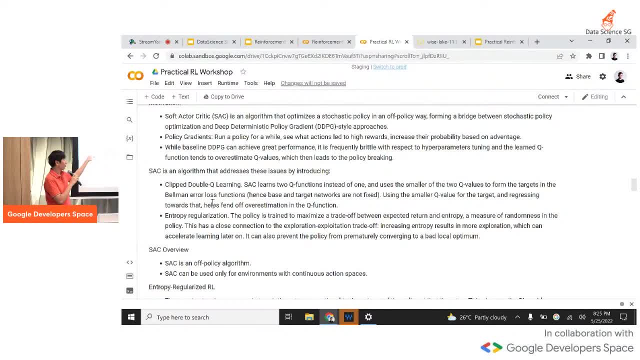 How do you solve the problem? Clipping is introduced to say that we don't need to fix them, We can swap them around. So basically, this is saying that this helps prevent overfitting again. So instead of having two nets- that is kind of fixed in the rows- you swap them around. 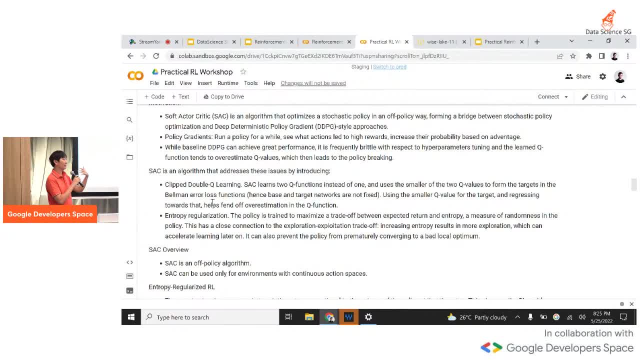 You allow them to kind of play different roles based on your training, And that's a very good, that's a great idea. Entropy is used in decision trees and things, So entropy is introduced as a noise factor. So priority, majority of priority. 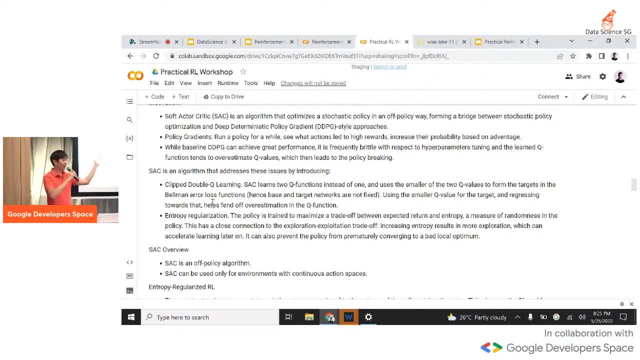 So at the start we want to say: we have very high entropy, or chaos, Do anything you want. And as we go along we decrease the entropy. So that's the remember. we talk about how we balance the exploration exploitation. 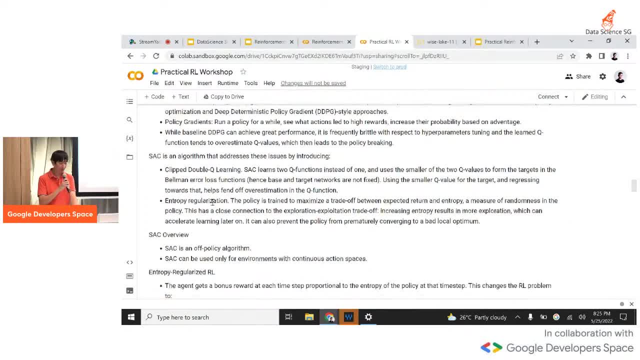 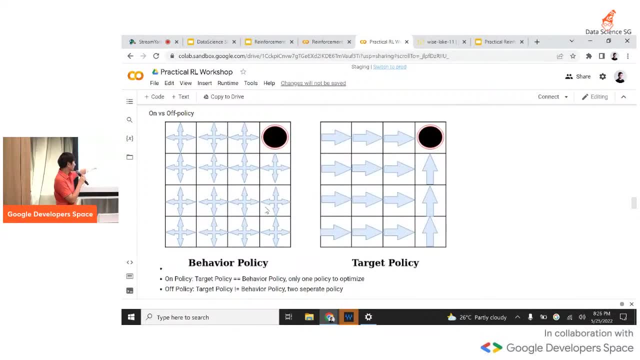 So entropy is a modern approach to it. Again, there are even more modern approach than what we see here. This entire formula- and this is what I mean by having two layers- on versus off policy, So you have a behavioral policy. This is where your optimal policy is: go left, go right. 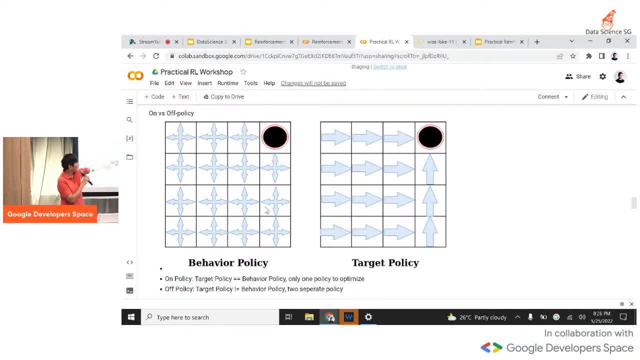 And each of these will have a score- What's the best thing to do- And it's a target that ultimately maps what you should do in each. So, by having two different policies, This is known as the off policy- Off policy approach. 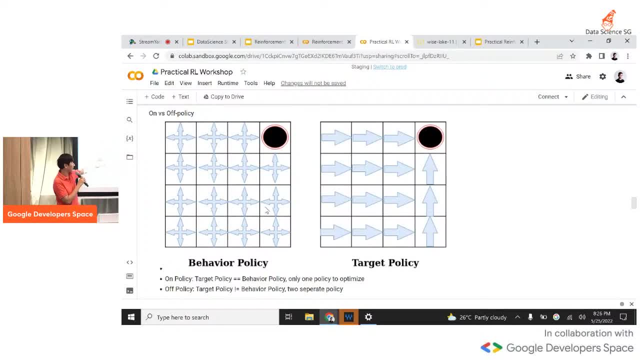 By separating them out. number one: it's a bit more resilient to some attacks Because now you have two policies that check each other. And number two: some of the modern approach. these things can swap around So the agent can learn more diverse actions and things like that. 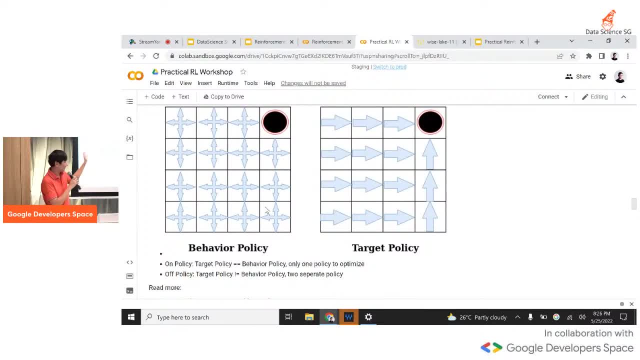 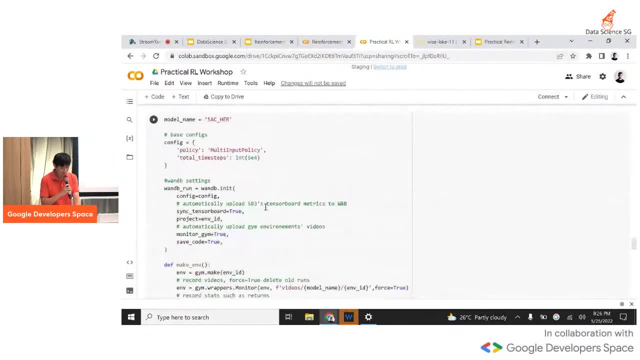 So there might be other modern approach that has multiple layers, But yeah, just the main idea of it. OK, we have four minutes, So OK, so the entire code is here. So actually you can just run it And you can train it. 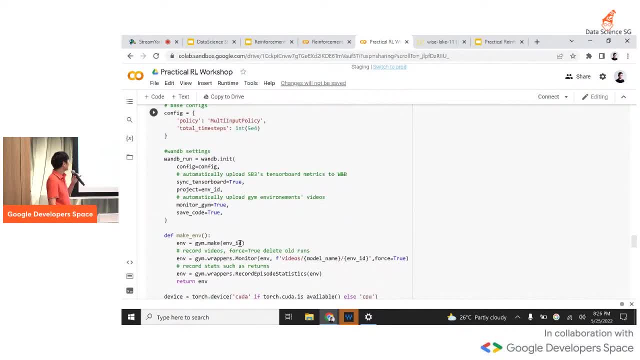 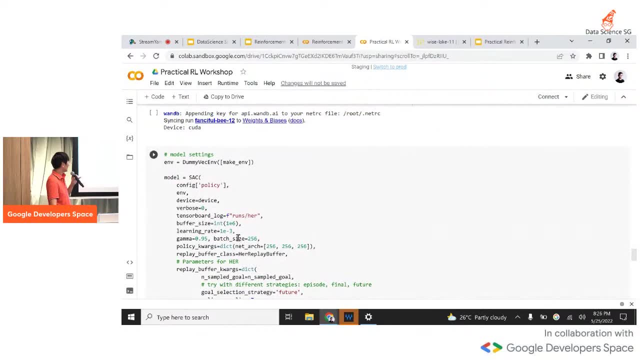 What I want to show you is actually it's quite clean in the sense that. so this is the TensorBoard thing that I'll show you later, But the model itself is like that, So they build it such that it's very familiar to those that use Vue Cycler, use TensorFlow. 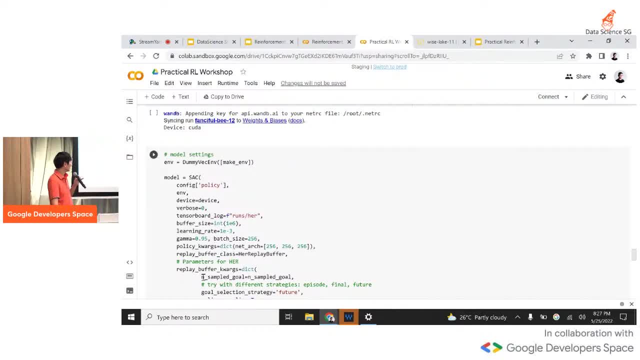 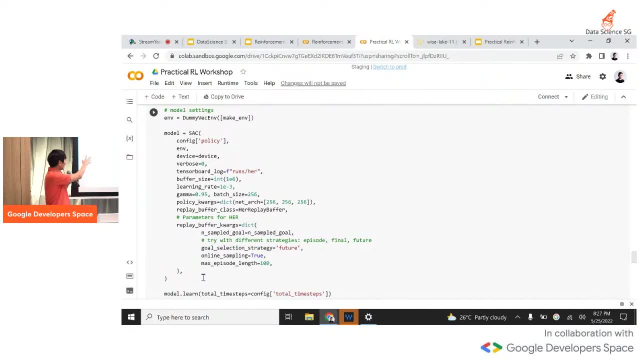 all these models. It's pretty much just: you call a function, you put in all the parameters. Below I got the Optuna that talks about how to hyper-parameter tune all this using TP three-person estimator. OK, OK, So TPE thing. 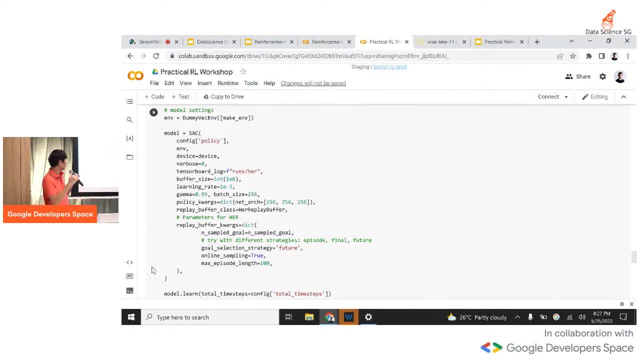 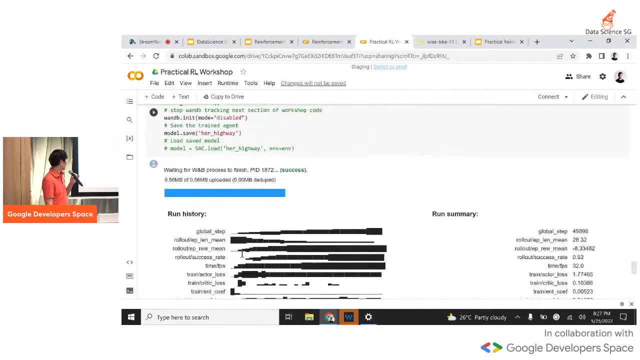 So for those who are interested in hyper-parameter tuning, go below. look at the third part of it. We won't have time to cover it today, So anyway. so you see it's pretty clean, And then it pretty much just uploads everything, all the scores. 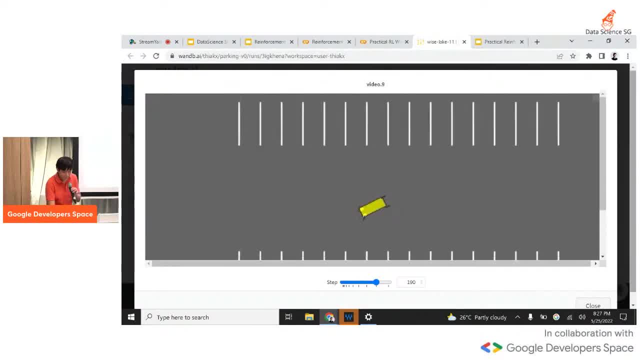 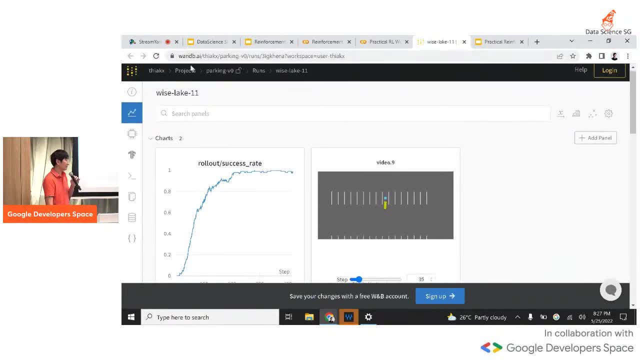 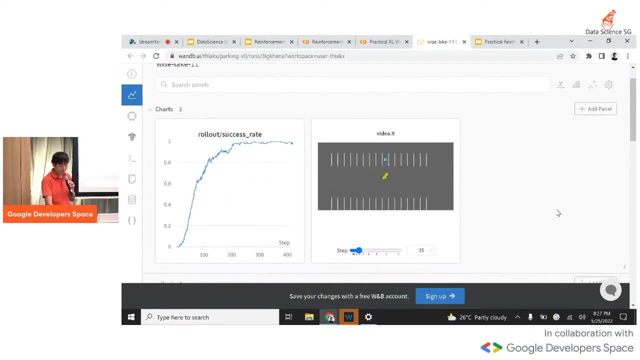 And you go to this MLOps thing And let me find a way to close this, this close button. So this is a. you can use any MLOps. The WANDAB actually integrates directly with the application. So you can see the package we are using now. 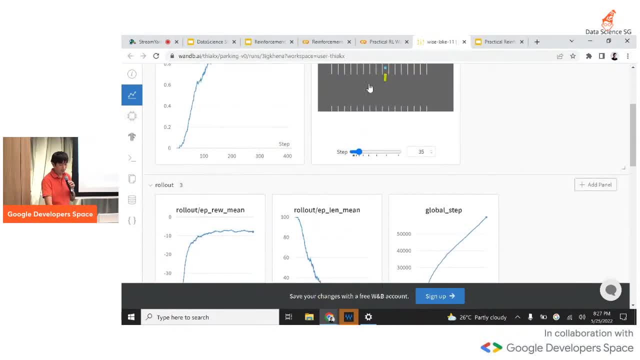 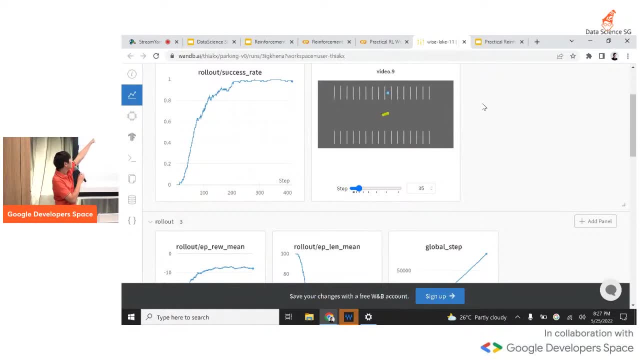 Hence, just keep it easy to see. So it has the outcome of it, which is important, But you can see the success rate. So, over time, what we're going to see is this flat line, So things that we have one shot for. 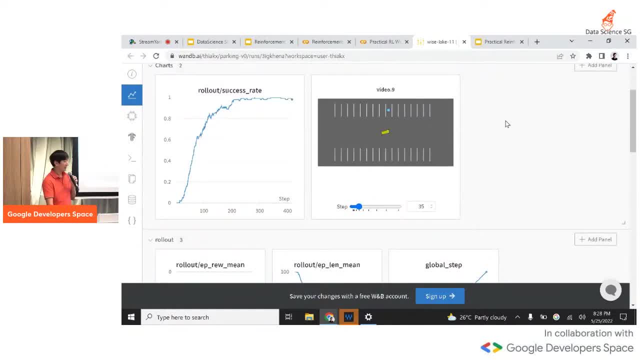 The flat sign at the top is telling me that it has 100% success rate. As you reach about 200, 200, you start having almost 100% success rate. So you can have all these topics. you don't need to train 400.. 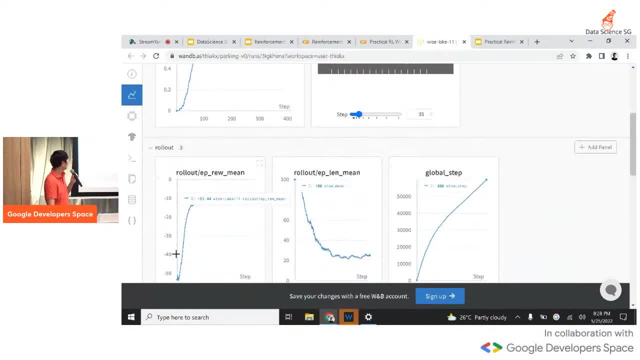 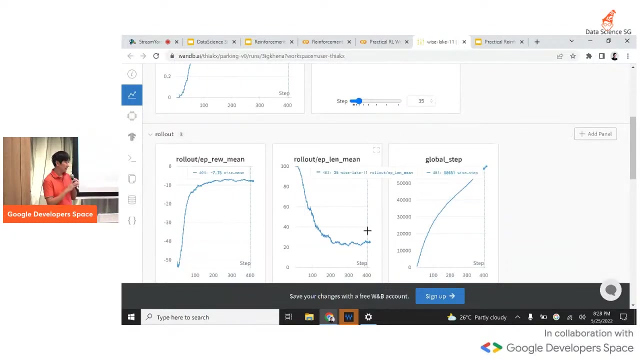 So 200 is good enough, And then this one for the MLOps things okay. parking problem: you don't want to go around in circles, so you want to see that the this thing is falling and it stabilizes. so it doesn't go around circle, you just go straight for the. 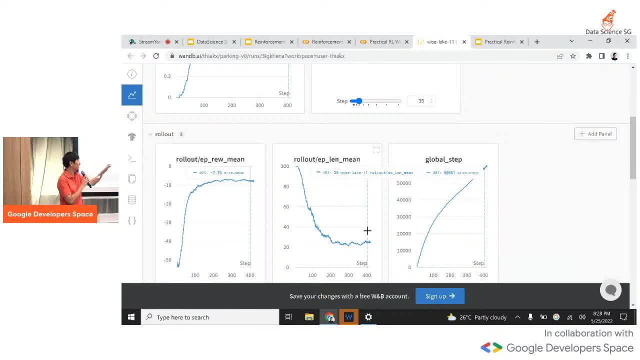 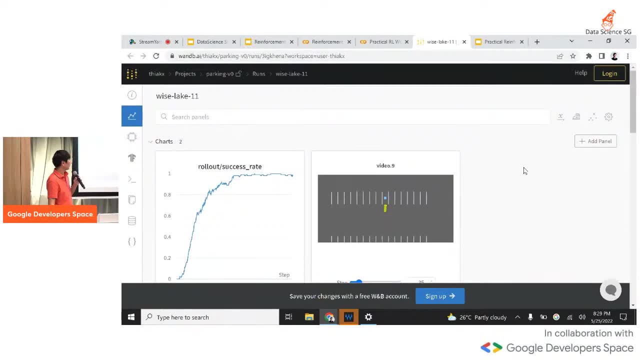 parking. so again, it's problem specific, but this is how you read this kind of chart. of course, global steps, you just increase that. i mean this is number of steps that goes over time. so having a ml ops platform like this tracks all these pieces as well as the. they have all the. 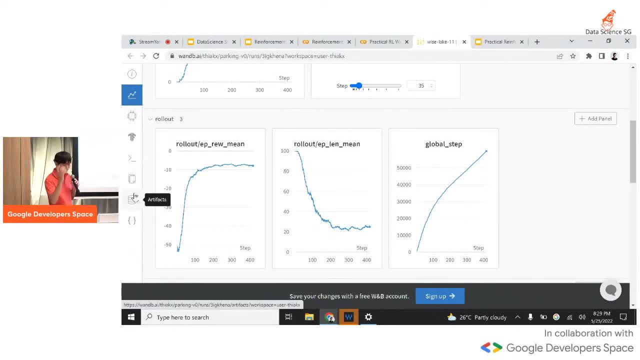 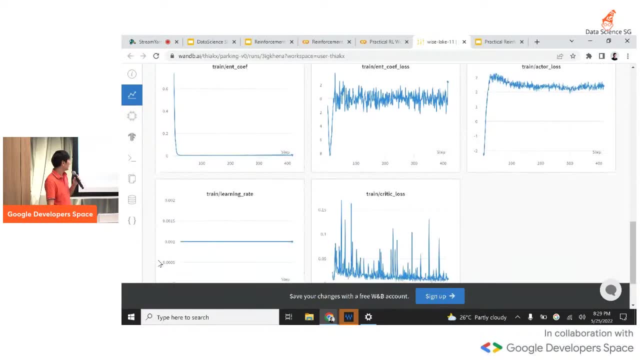 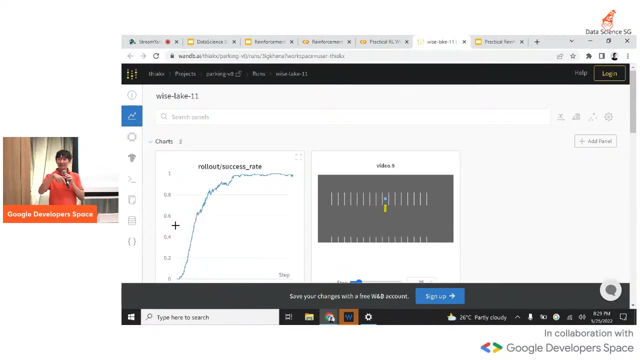 the setup, the, the whatever resource is used, and also your model is safe, things like that. so again, it's, it's important for for reinforcement learning agent in particular because you want to see all these various pieces and i have one minute, yay. so q a is after this or after this. 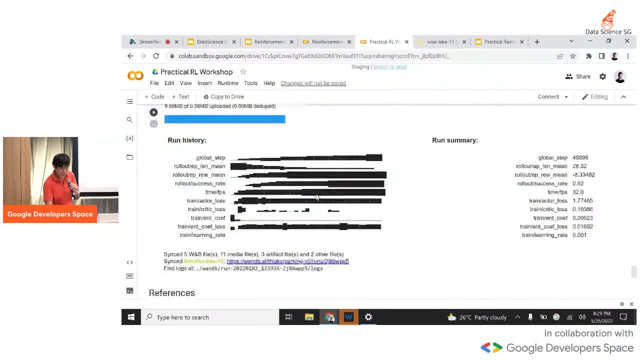 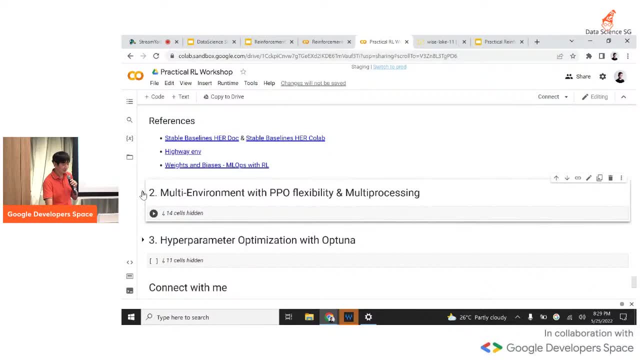 okay, so i can wrap it up quite quickly. um, so that's for the this part. so each of these i have some references and go on for the documentation, ppo is interesting because the- yes, you has multiple use case. so, uh, for ppo, you can exploit further on yourself. it's an algorithm. 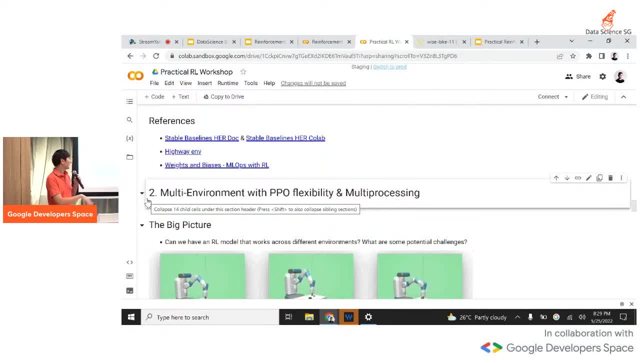 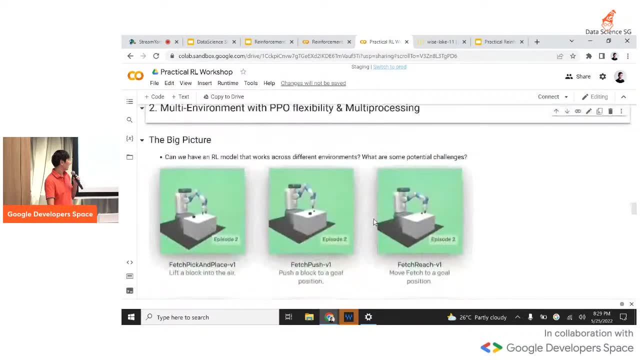 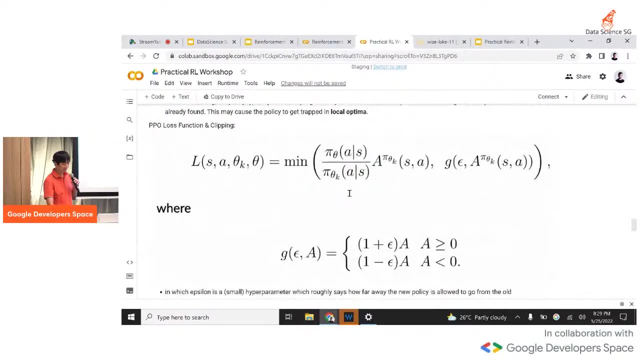 that i call it kind of the baseline for everything. in rl you can run anything. in ppo, the open ai was using ppo as the baseline algorithm for quite a couple of years because it can run in anything. you can run robots, you can run driving and run uh like all sorts of uh algorithm and unfortunately, 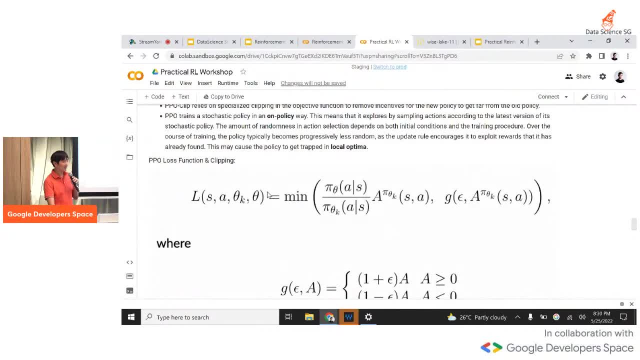 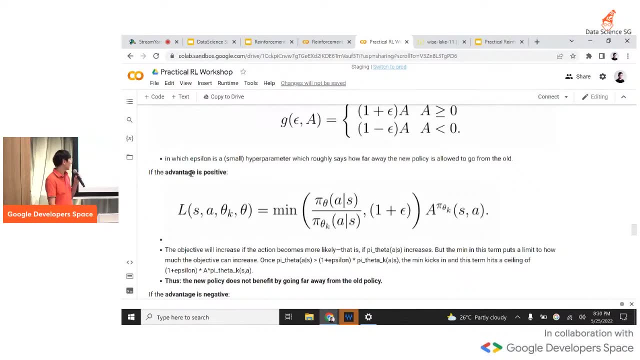 don't have time to kind of go through all these details you. you can take a look at the notes i have here and then you can ping me if you have any question. they focus on advantage, so they use advantage to talk about policy again. this is another way to counter poisoning effect. 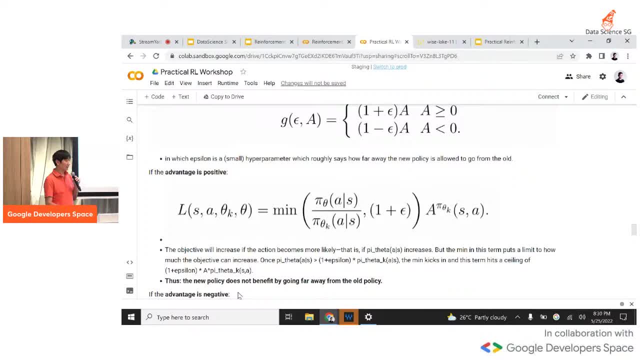 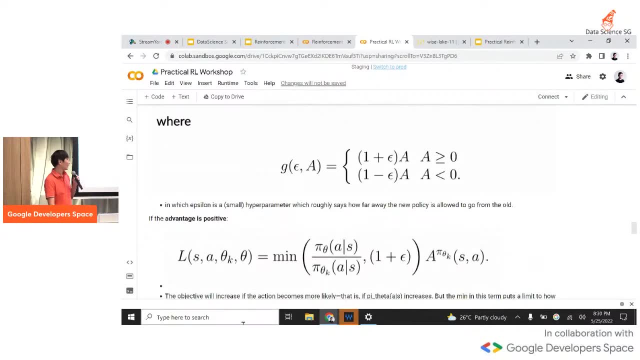 by keeping track of the policy delta that you are training between the new and old policy. you clip it using the advantage advantage formulation and value. so all this formulation is just trying to keep your delta change in a small, controlled manner so it doesn't go go total. 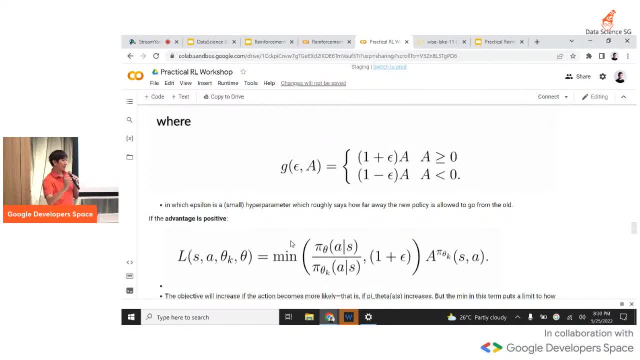 off the charts and totally go, go crazy poisoning occurs if, let's say, i want to force your- i am jealous of your car parking thing, i want to eat to crash all the time. i want to kill all your customers. so i'll put in the reward function that such that i trick it to think that crashing will. 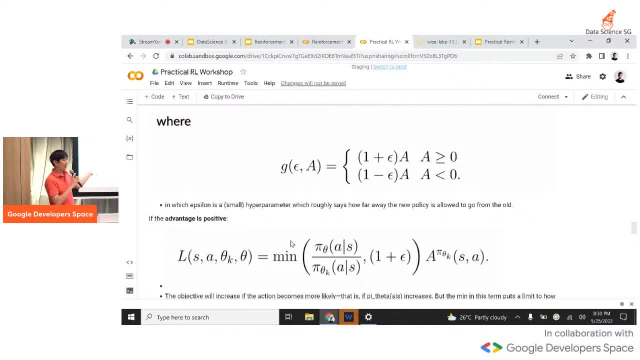 give you a lot of reward, so that's poisoning. so clipping advantage. clipping will prevent that, because you cannot suddenly switch from a parking agent into a crashing agent. the difference is too big and then clipping will stop it from happening and will flag out a bunch of errors and stuff. so that's one way to that. modern approach can also prevent such uh such. 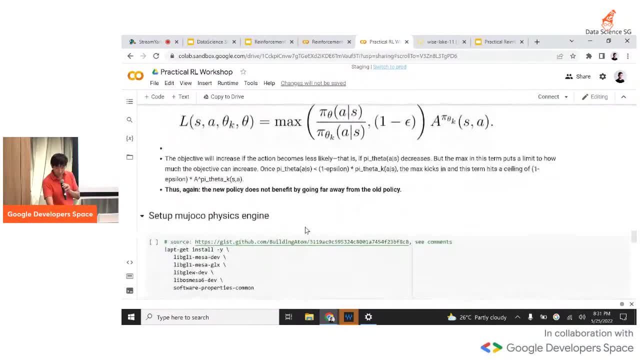 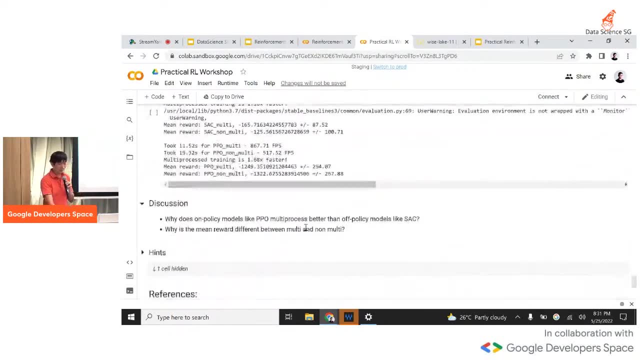 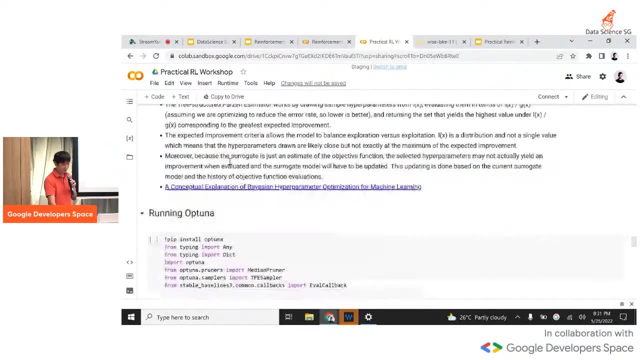 adversary attacks. okay, all right, over time, one minute, but yeah, so the last part is the, the, the. i can check the, the hyper parameter, tuning yourself the optima, and if you are familiar with tp or you are not familiar with tp, you can talk to me as a tree based parser estimator. and yeah, so this one. 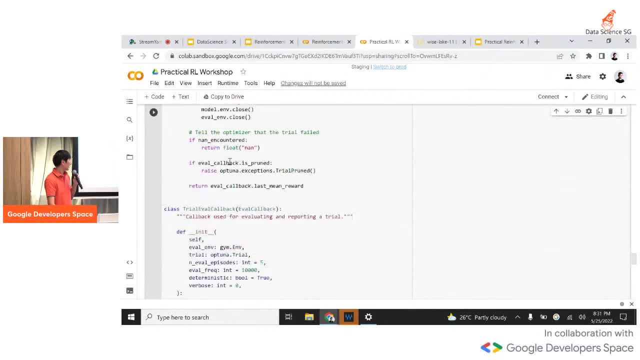 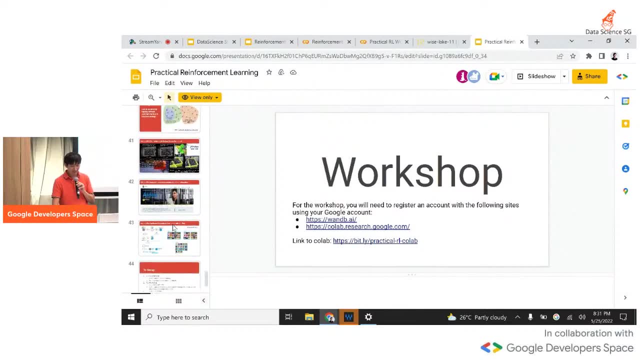 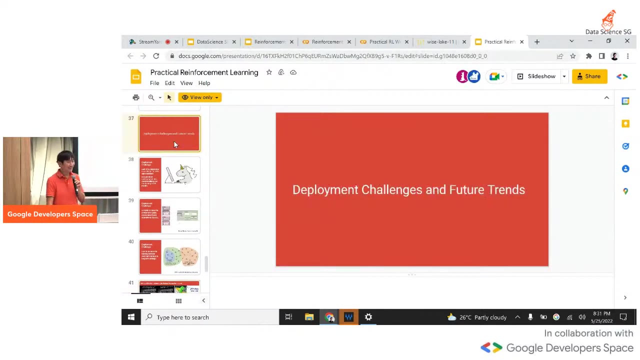 actually optimize the tp. all the parameters you see just now, uh, yeah, okay, so that's, that's a very fast- and also the actually beyond workshop, right, the? you can check out my last part where we talk about the usage of it. yes, someone is coming to kick me off the floor, is it? so last part is the department challenge and 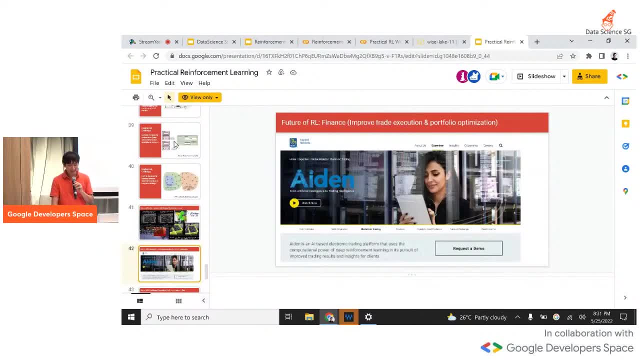 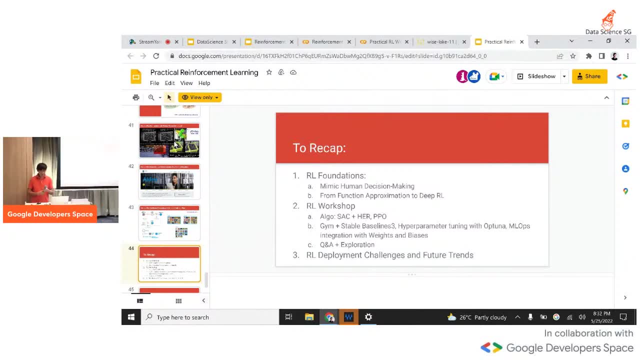 all the, all the various uh pieces of that. that. why is like five times away and how is it used in the real world? yeah, okay, thank you. okay, uh, we'll do a quick q a now. uh, we'll take, probably, i think, given the time that we have. 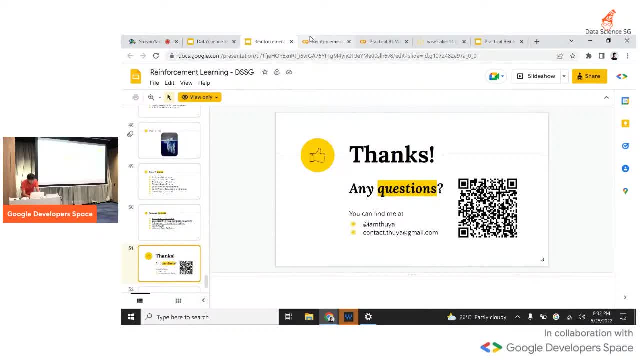 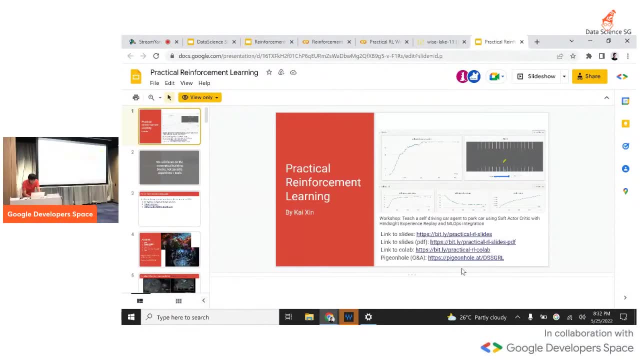 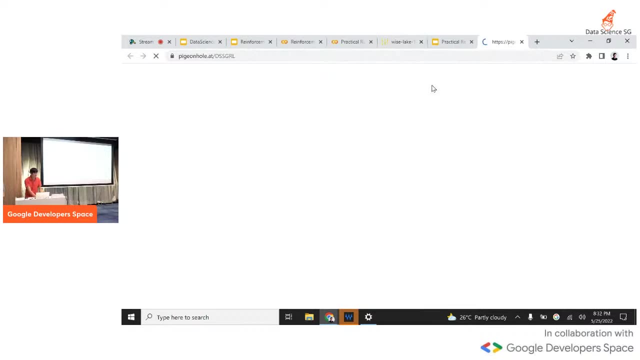 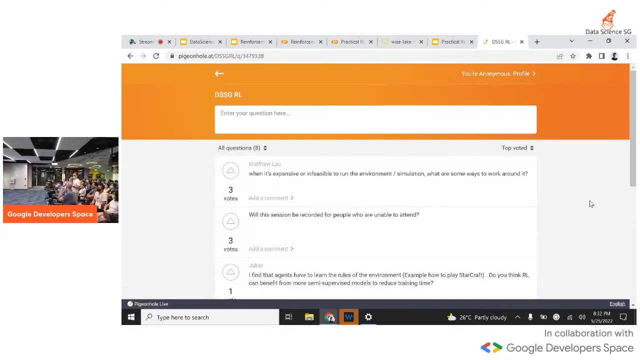 we'll take about two or three questions. uh, anyone has any questions? just raise your hand, okay. so, uh, when you ask a question, just keep your mask on, okay, yeah, okay, thank you for the presentation, so it was very awesome. so, my, i have a very common question about um data set you mentioned in the beginning. 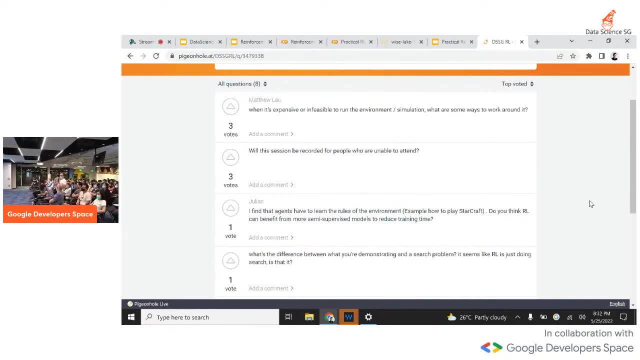 of a presentation that we have to collect all car parkings around the world, in europe, in singapore, in other countries. but to be honest, me, like i am a driver, i don't need it to do it. i don't need to travel all over the world and just look at all car parking. i just need maybe two, three of them. 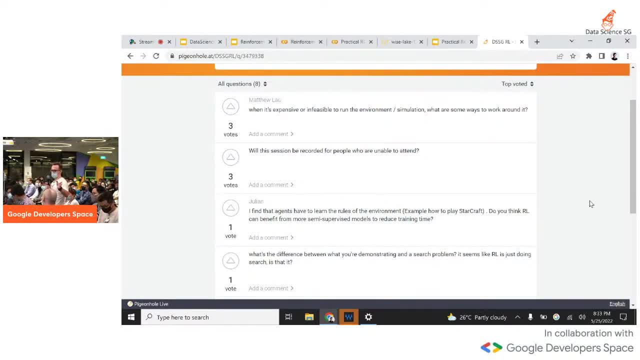 just to understand conception and i can go to the other country and just park with with no problems. so is any ideas how we can just switch from this classic approach of collecting as much as possible data to some new conception? so this is a question. yeah, so the what i presented just now, right, the 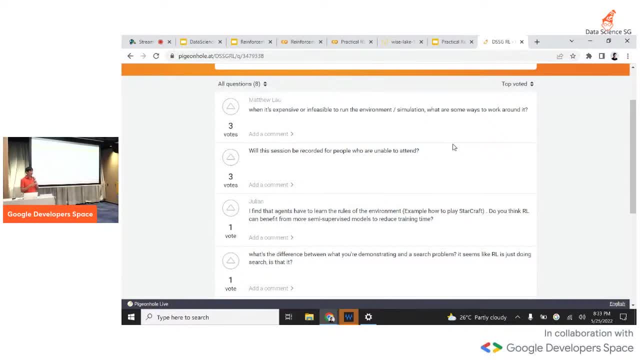 sac hindsight experience is to solve that problem. so the whole point of reinforcement learning agent is: you don't need to get all this data. all over the world you generate this data. so how starcraft they manage to play, starcraft they manage to play go, how that agent managed to park. 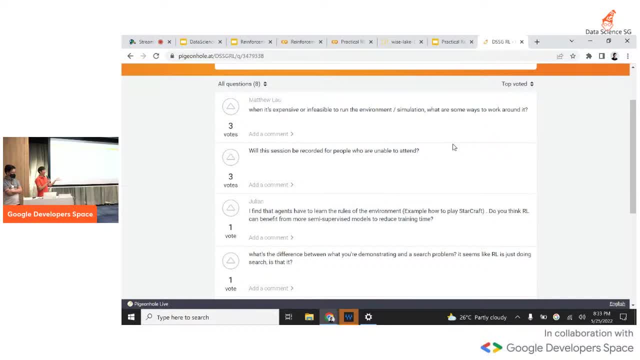 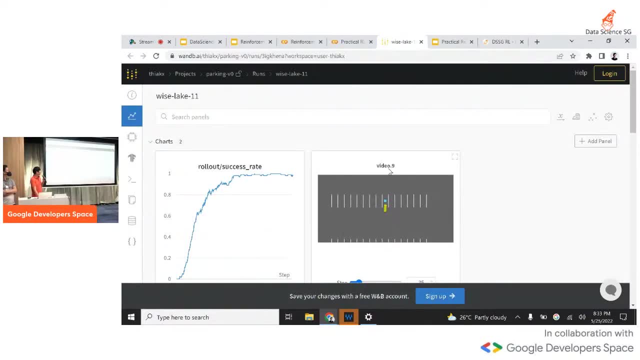 the car is by generating its own label data by running it through a simulator. so, whatever you see, that's happening here, right? so it's true that we didn't feed any data. we didn't tell you anything beyond the state action reward. so this is literally what we are presented: station reward. 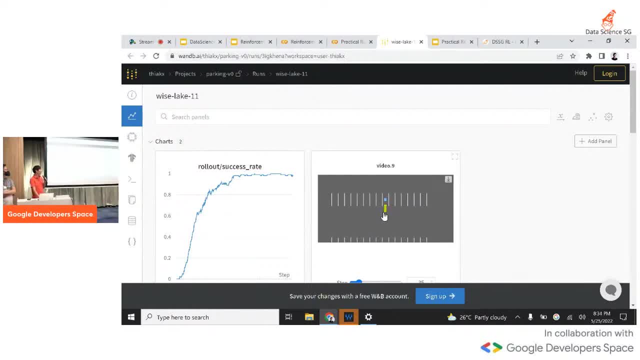 function. that's all the, the agent knows, and he learns how to park a car just by trying to optimize reward function. so in this case, he learns to go backtrack to to get to the. it doesn't understand parking at all, it doesn't. it's not fed with any additional data, it just learns that by doing this. 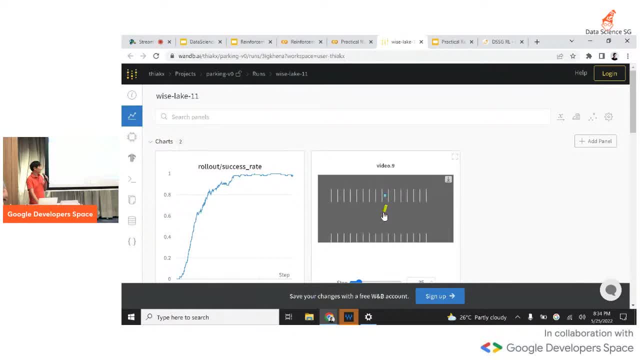 thing, i get the most reward. that's all i care about. so so the this is the modern approach indeed to solve uh problems like this, and it's used in some of the self-driving car applications. they're using this concept together with some of the supervised learning method, like computer. 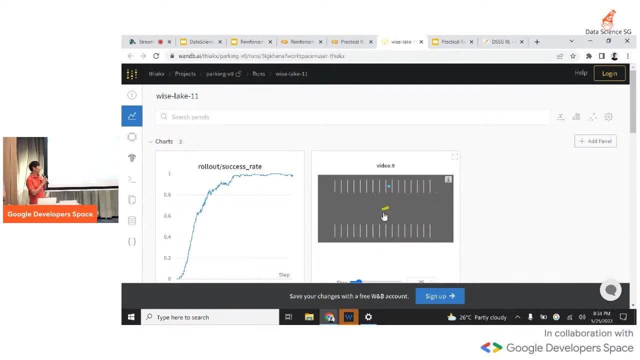 vision and all this to supplement it. uh, yeah, but the in this way you don't need to do all the collecting all the data. yeah, but by using reinforcement learning. so i have some experience with like training, this kind of model. so if you forgot to like implement, 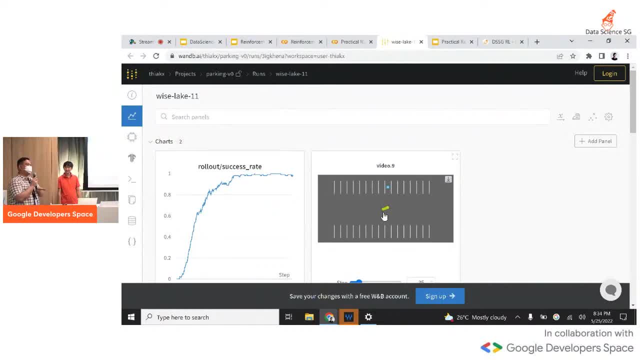 some of the rules. let's say you ask the agent to just drive straight away, right like you. just keep on the road, keep driving front. if the car is on the other side of the lane it will skip. do that, but it's wrong, right. so you've got to find out all the rules to implement it so that it doesn't. 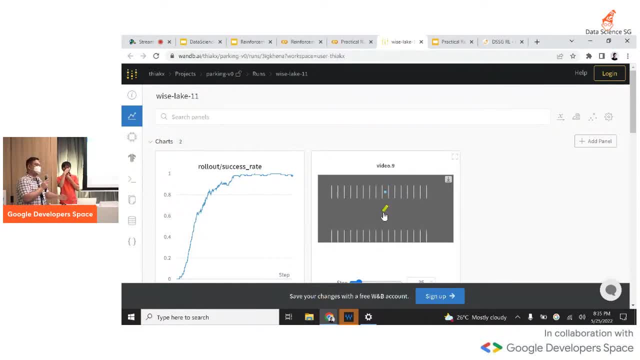 violate the traffic rules and different countries have different traffic rules. sometimes you drive left, sometimes right, so you've got to train all these rules implemented inside the model so that it will it will really work with it. yeah, excellent, yeah, excellent point. yeah, so the rules: definitely this one is like no rules on this one. it does everything you want, but the rules are important. 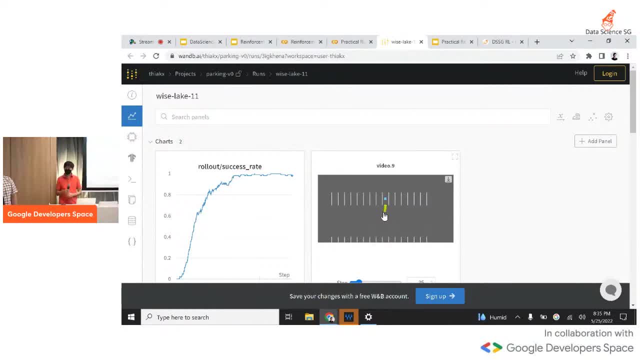 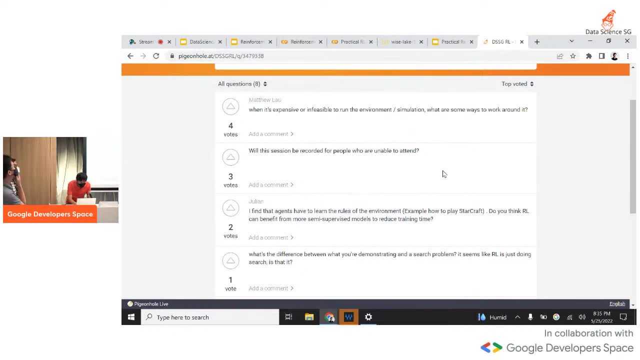 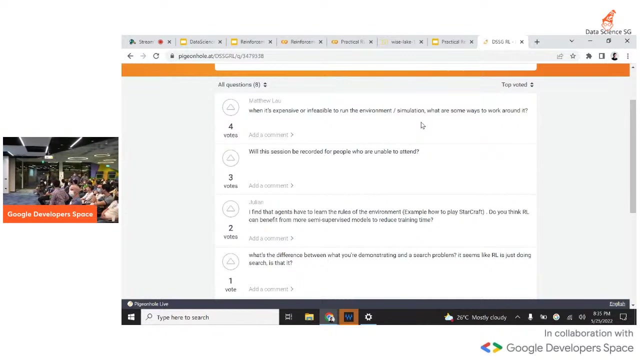 as well, to kind of qualify it. okay, uh, hello, all right, one question, hello, yeah. so my question is like: initially you mentioned that there is a difference between a agent and a model. uh, can you explain that? okay, so so in reinforcement learning, the model sometimes refers to the environment. Like, what's the model? 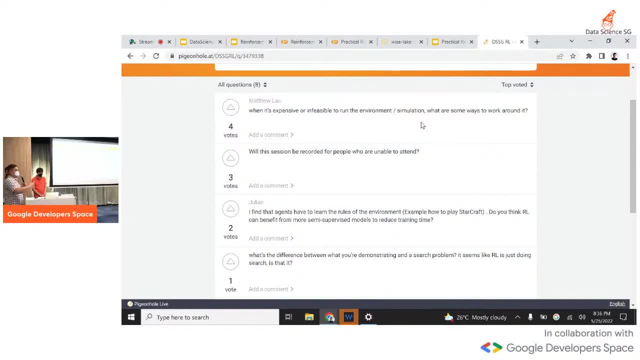 Your environment, state, reaction, rewards And in Q-learning, if you see, sometimes they convert. So you don't really see the entire environment. You only see some states and some observation. But in some other problems you don't really see the states. You have to guess. 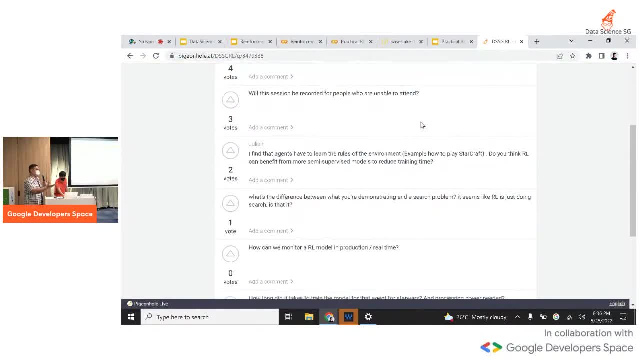 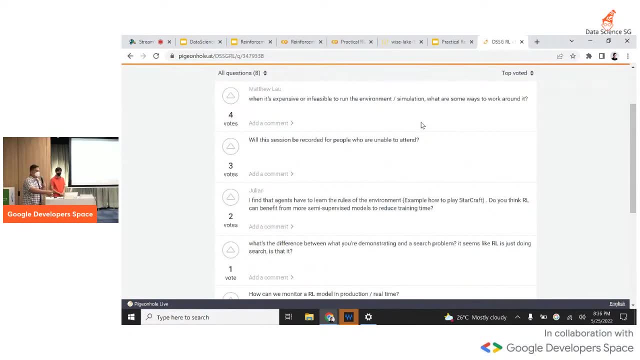 it Like you don't know, You're in a blind and try to drive at night or something. So sometimes we imagine model In D-reinforcement learning. we use D-learning model in some aspect to guide the agent to do certain things. So in that, 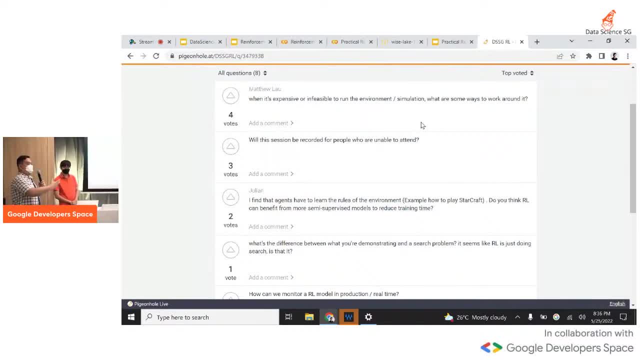 way you will call model agent. But whatever I did previously, I wasn't training anything right, So it was not model that I trained, So it just tried to find that policy plan by going through one by one, So that's not really a model. 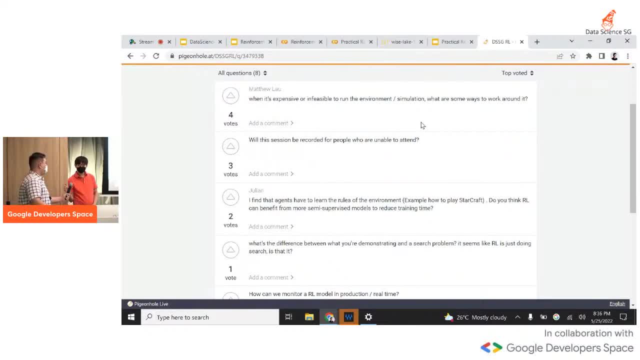 right, Yeah, So I hope that explains it. Okay, So some very good questions here. Actually, I'll try to cover a few more, Because the first one, the answer is there's no. Okay, Let's think about the biggest. 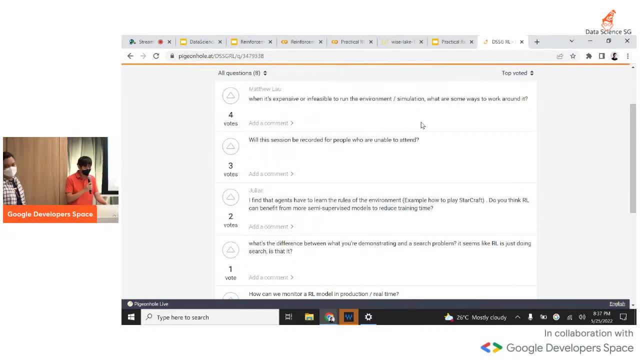 challenge of RL is how expensive it is to set up the environment, How challenging it is. There's no way around it. You need to have a very, very sophisticated and good environment. Maybe there are some experts that can correct me, But as far as I understand, 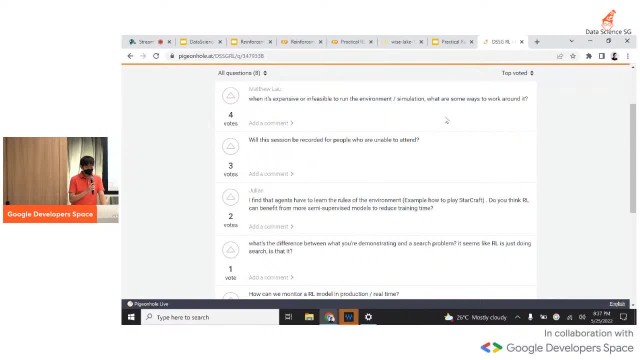 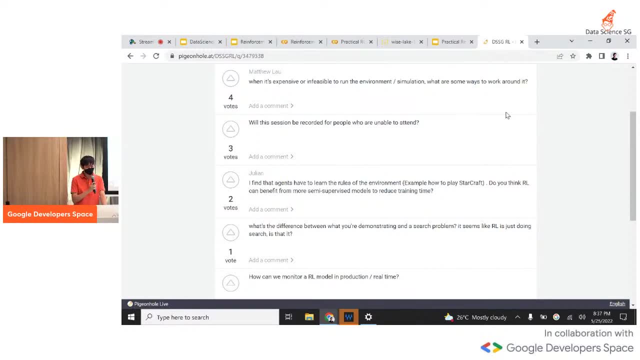 there's no way around it. It's expensive. The OpenAI team spent millions, billions of dollars to build their StarCraft and model and try to monetize it through healthcare nowadays. But it's expensive, And both in terms of hardware as well as the talents. 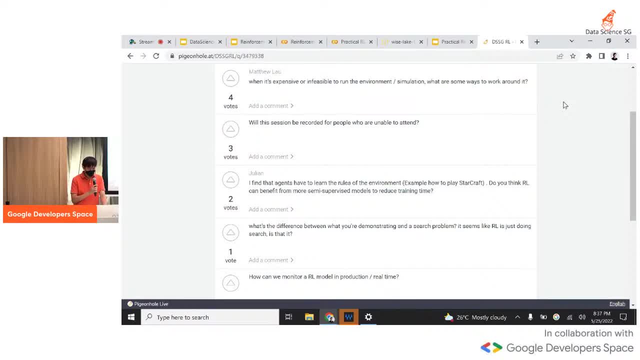 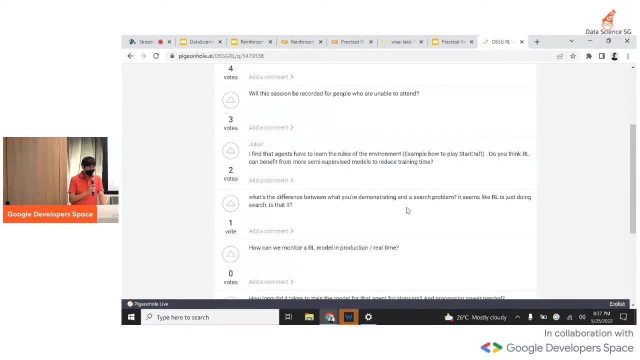 needed to maintain it. It's crazy and infeasible. Give it five or ten more years, You can't use it. There's also one very good question about the search. I thought about it So when I was doing, Even in my school days. how is it different? 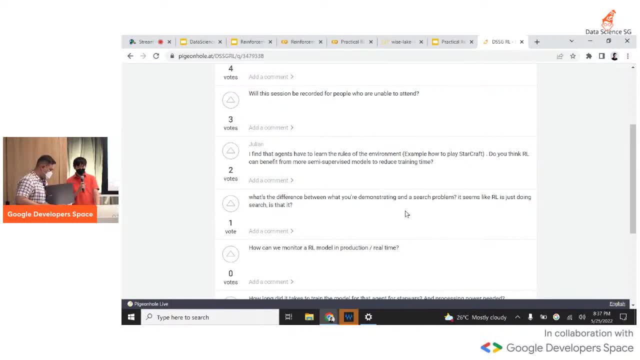 from A-star search and things like that, right. So it's true, it's a search problem to a degree, But A-star cannot park a car, So there's a limit to what all these search algorithms, computer science theories, can do. It's very defined. 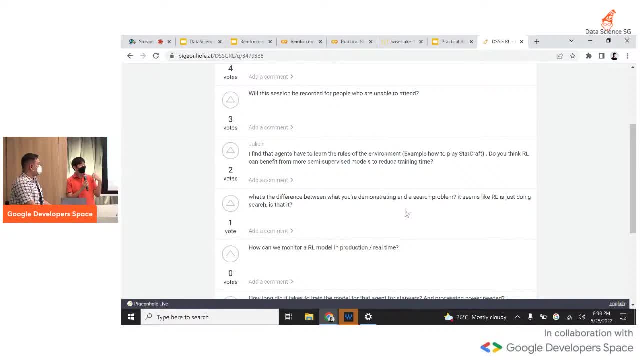 I say defined distance problem, shortest distance, But even then you know, all these Dextra, all these various pieces have a lot of limitation in the real world where there are traffic, where they need to react to crazy drivers. One guy was cutting my 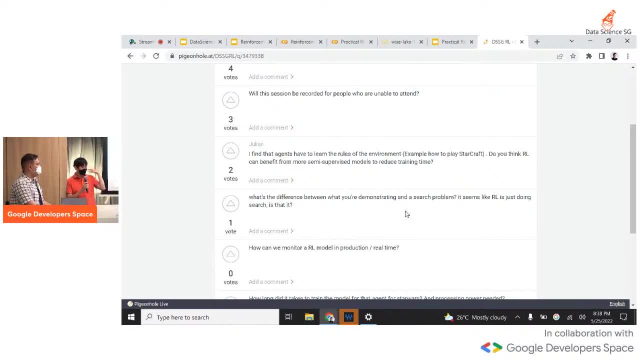 car. just now, Another guy flashed a high beam at me while I'm parking my car. So crazy drivers like this, you cannot A-star search it because they'll just assume perfect condition and crash in. So reactionary is something that differentiates RL. 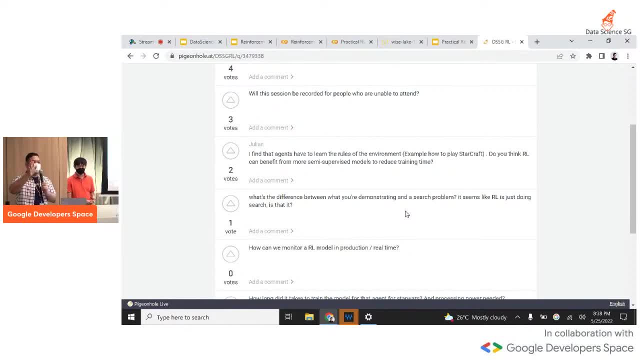 So you also have to cater. in the real world your car can go like 90 degree, turn right, So A-star probably go there. So you have to have to cater that. So the car go this way in a curve direction, but not 90 degree. 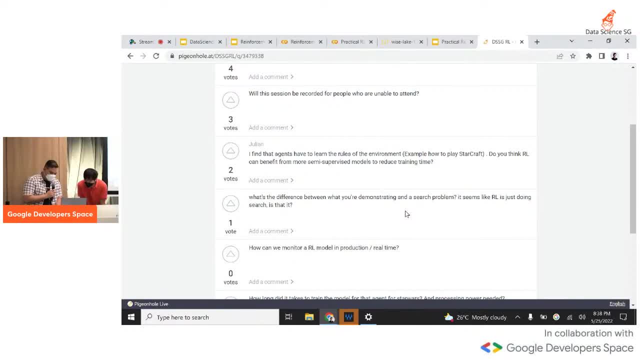 Go ahead. Some question from the YouTube is like: can cultural learning contribute to RL policies? Can Read paper? Read paper? I've seen before but I can't remember. I go find some and post it later. Yeah, but yes. 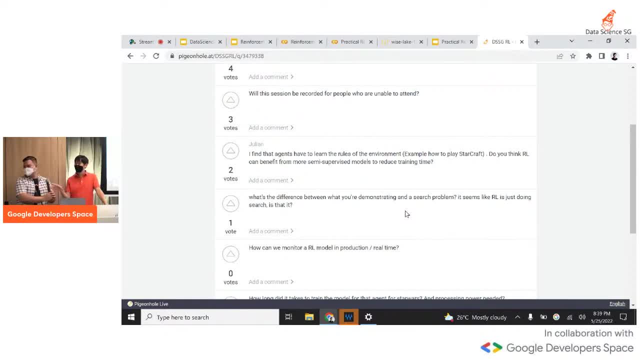 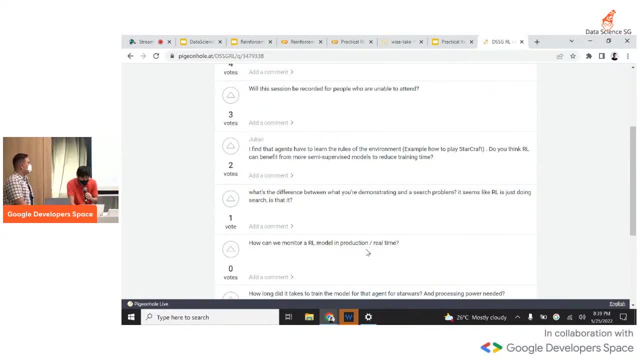 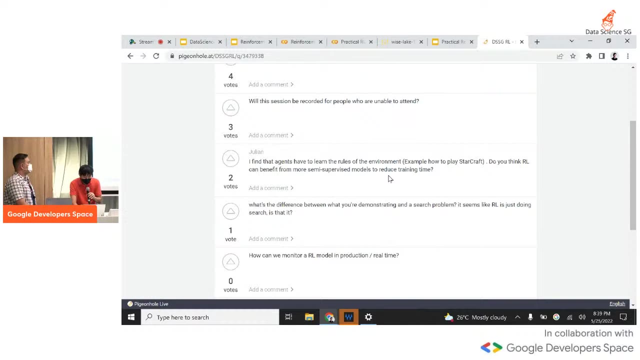 Yes, but I forgot. Yeah, One more question. So monitor RL: yeah, show ML Ops, Use ML Ops, thing similar to that You can monitor thing. I find agents have learned the rules. So the interestingly for StarCraft. 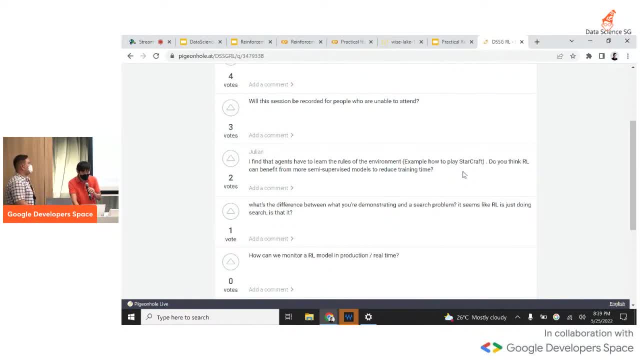 they started off trying to feed a lot of the StarCraft rules as well as the player history. In the end, it doesn't matter, They just play against itself. So again, the modern approach for RL is: you don't need rules. You don't even know what game you're playing. 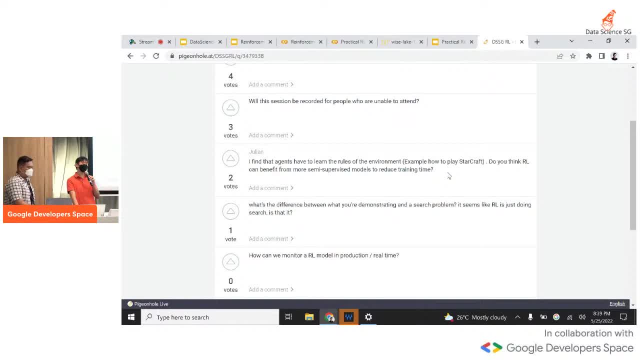 or how it works. The scary part is it doesn't know how it works, It just knows it has to win, regardless of whatever it does. So the RL agent plays against itself and just trains its own mind to solve the problem without knowing the problem. And that 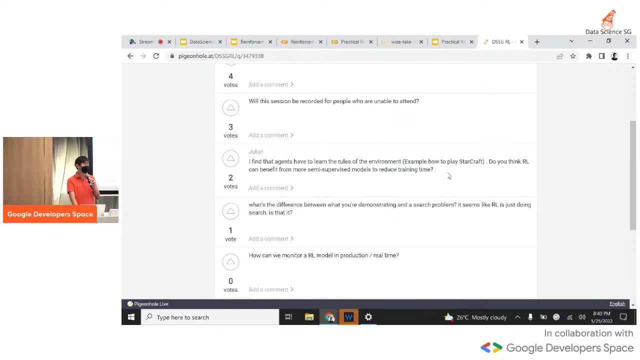 comes with a lot of issues if you want to deploy it in, say, healthcare and all these things where you need explainability. You cannot explain RL easily because it fundamentally doesn't care about rules, It just cares about reward, how you optimize the rewards, And hence I think to what I was sharing. 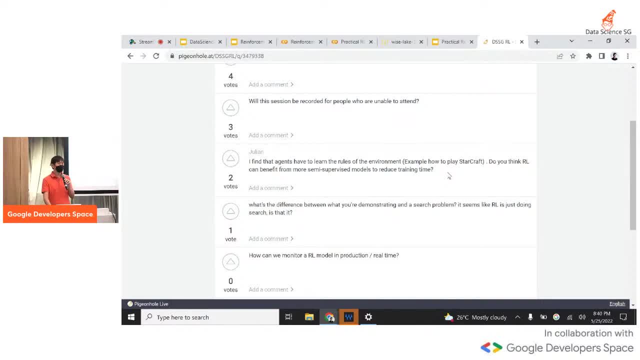 agents can play 37 games. how many games, right? It doesn't matter. You don't care about rules, They don't care about how it works, as long as it reaches the goal for them. yeah, Okay, I think, in view of time, we will stop here for. 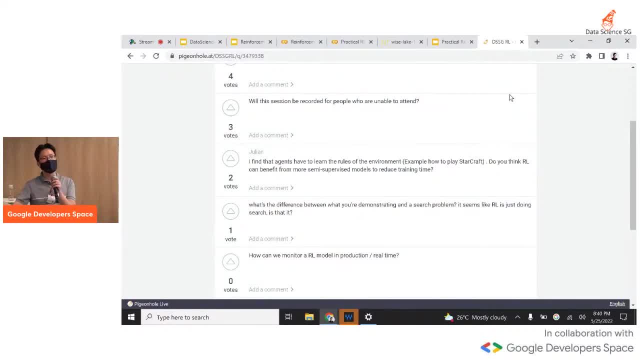 today. So first thing first is a round of applause for the speakers, please, And also to Google Developer Space team for having us hosting us. Thank you very much, Okay, And also to all of you as well. we didn't expect such a large. 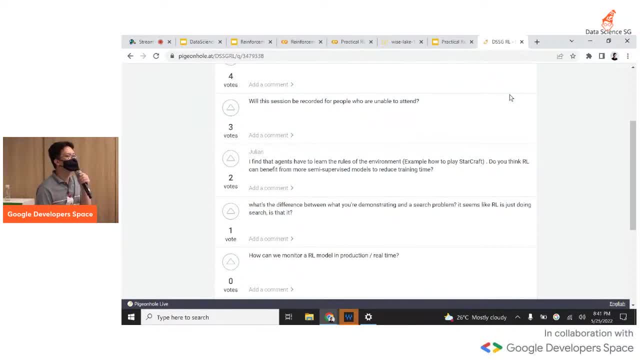 response, actually after COVID, with the physical meetups and all this. So a round of applause for yourself, please, for coming all over here for the R Science S3 meetup. So thank you very much. The speakers will still be around. You can still ask them questions. 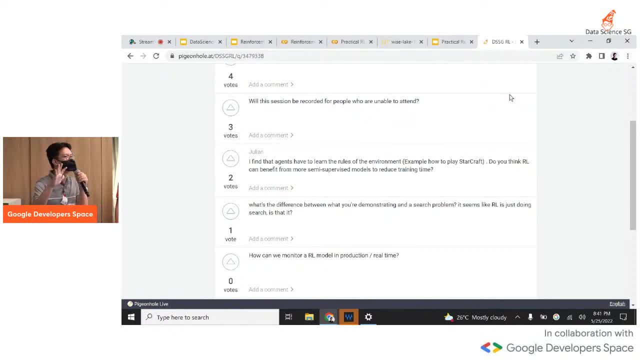 but please remember the safety measure. I can't remember what the other M stands for. Anyway, you all know what the SMM stands for. So one more thing I just wanted to remind. let you all know that the next meetup right is. 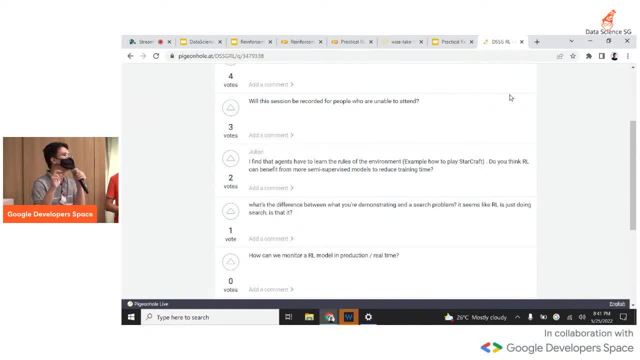 also physical meetup as well. It should be on the 22nd of June, So do mark your calendars and do join us if you are available, Okay, So thank you very much for coming and hope you have a good evening. Thank you.